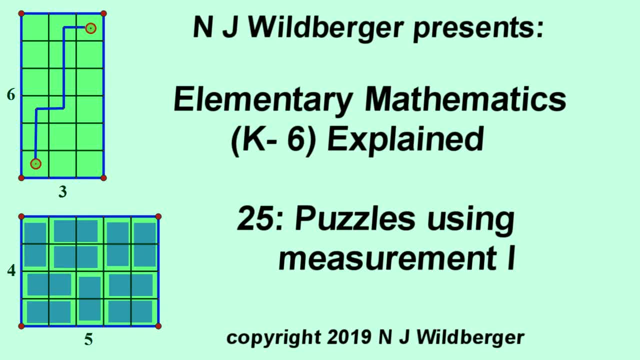 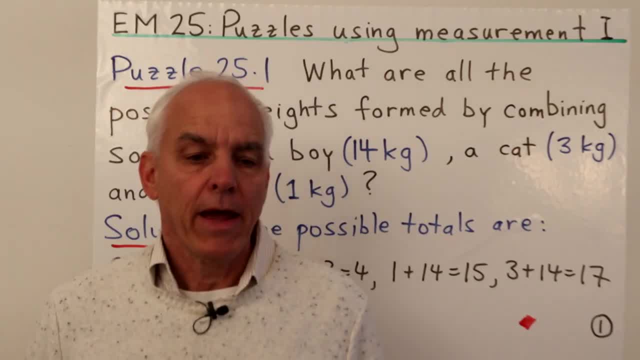 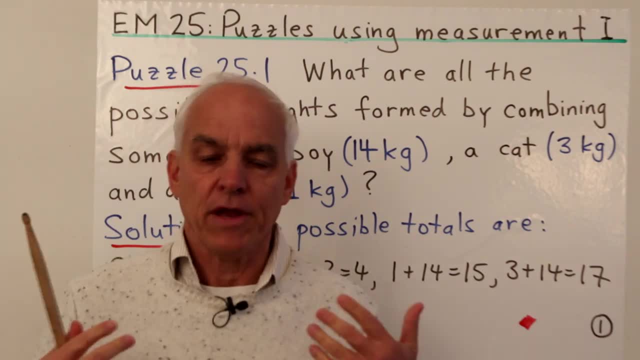 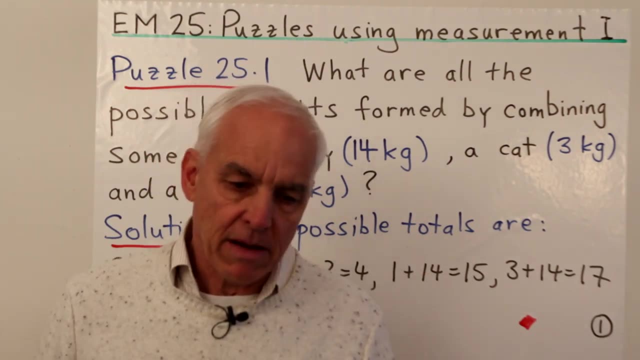 Welcome everyone. I'm Norman Wahlberger and we're engaging with some puzzles for young people K-6 which strengthen their arithmetical understanding by presenting them with some challenges. So we've already talked about some puzzles in the arithmetical direction. Today we're going. 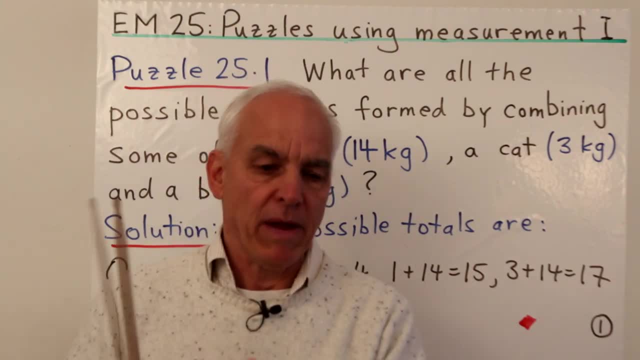 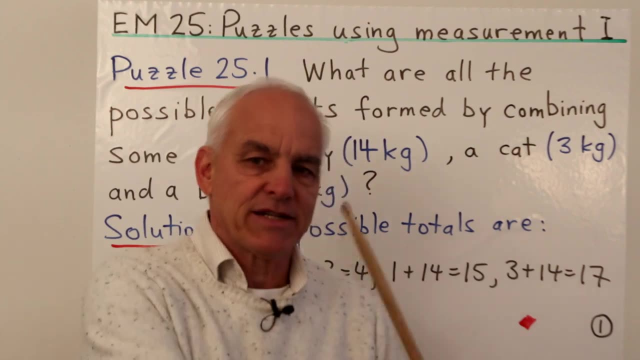 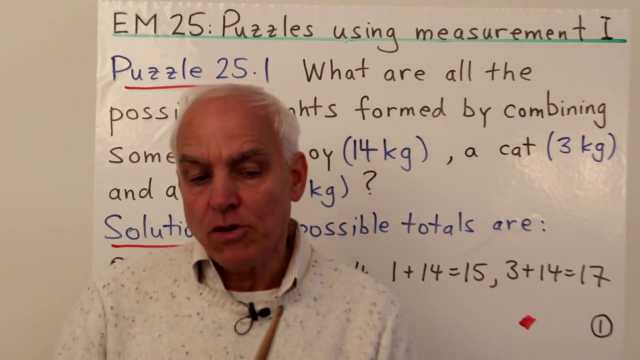 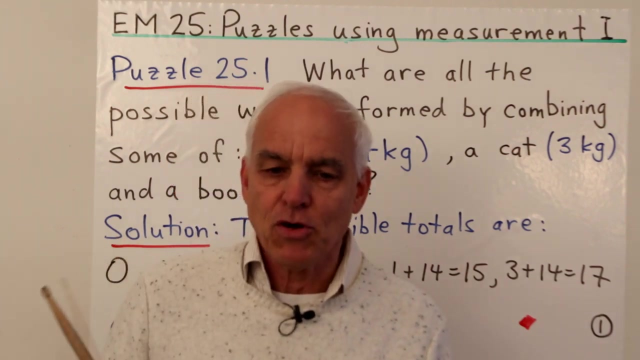 to start thinking about some puzzles which have a measurement basis, and we're going to actually touch base with some interesting problems that you know suggest further directions of understanding and exploration. So maybe a few words about puzzles more generally. So we're talking about very young people here, right? so some of them may not be able to read okay. so I'm really presenting. 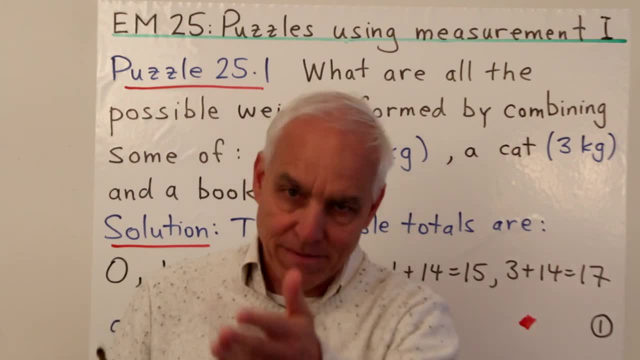 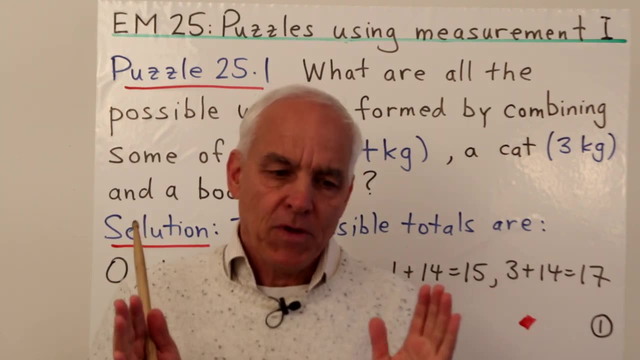 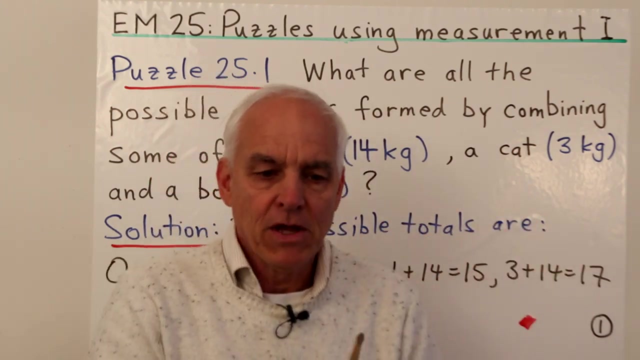 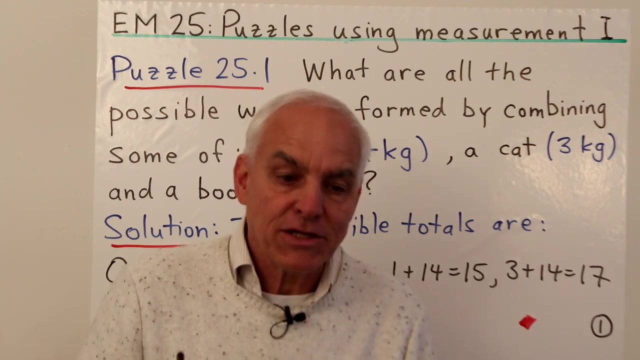 the puzzles to the educators and to the teachers and parents of these children. So I'm hoping that you take these puzzles on board as as potential directions to investigate with your children. Okay, so there's also an element here of judgment required, because obviously the kinds of questions 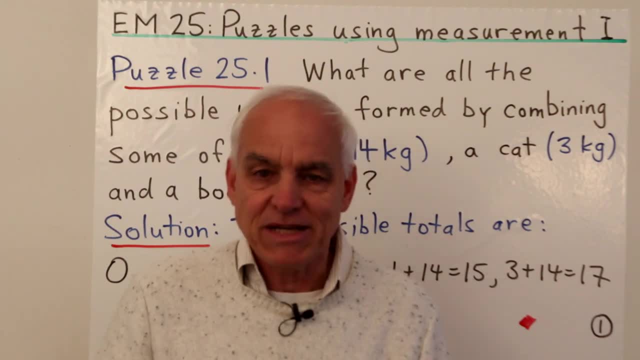 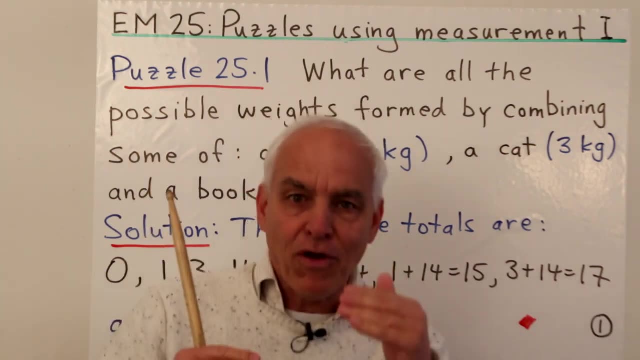 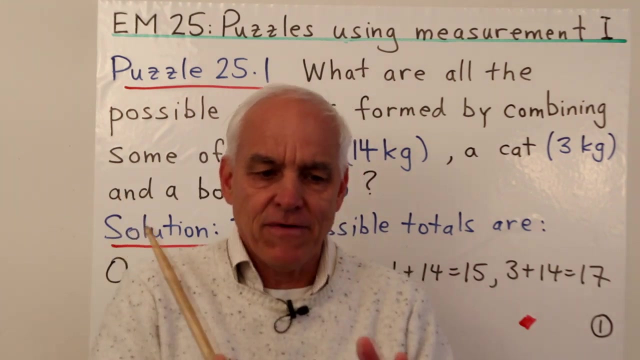 that you ask a kindergarten child is that's going to be different from the kind of questions that you're asking a year six child. So I want you to adjust the level of the problems and and be conscious of the fact that these puzzles have simpler versions. they also have more complicated. 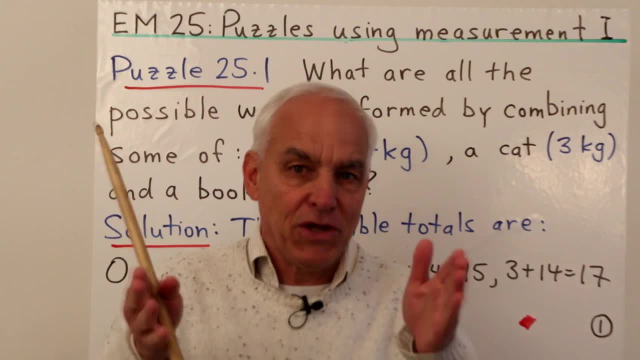 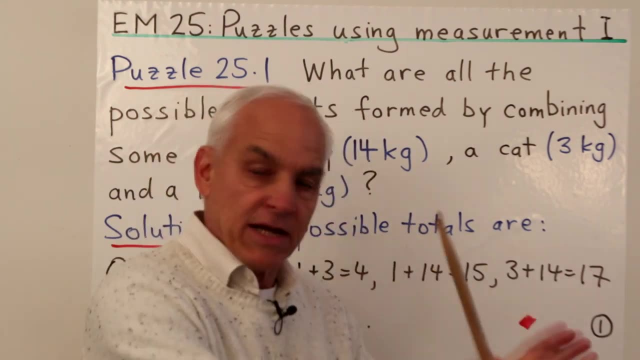 versions. They're a little bit open-ended, so it's important for you to understand the situation first. But what I'm trying to do is trying to say: look over here, this is a topic that's potentially of benefit for young people to learn about, so please introduce them to this topic through a 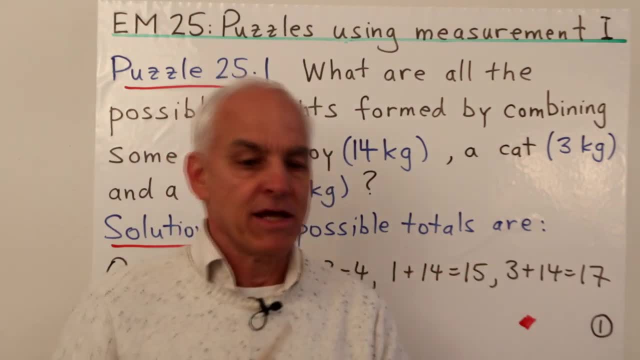 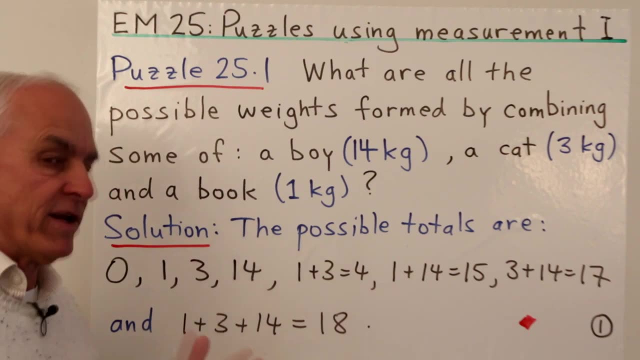 puzzle in the direction that I'm suggesting. Okay, so some flexibility on your part is required. So our first puzzle is an arithmetical one. essentially, We're weighing things. we've got three things actually- a boy, a cat and a book- and we're asking what are all the possible weights formed by? 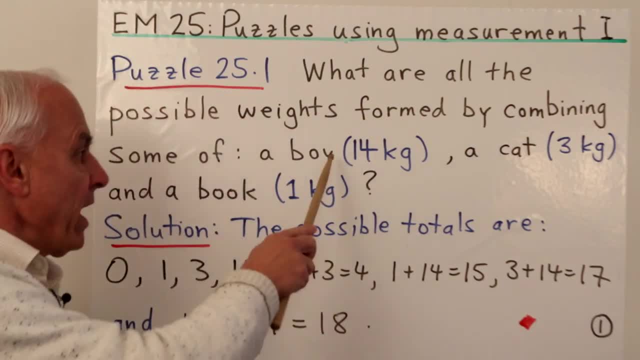 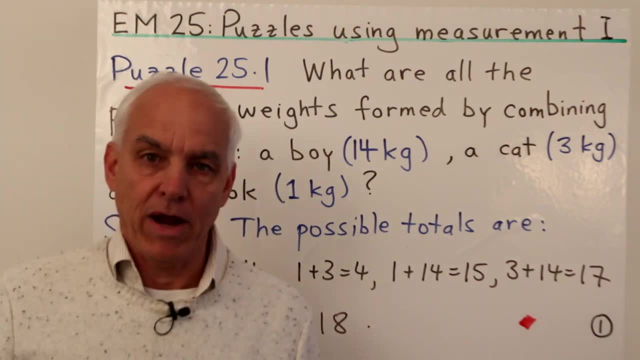 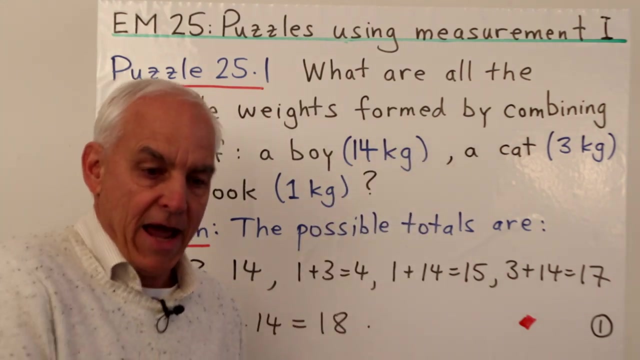 some of these three: A boy weighing 14 kilograms, let's say, a cat weighing 3 kilograms and a book weighing 1 kilogram. So we can imagine a scale and we're going to put a certain number of these objects on the scale and ask what are the totals that we can get? Okay, so the solution is that we 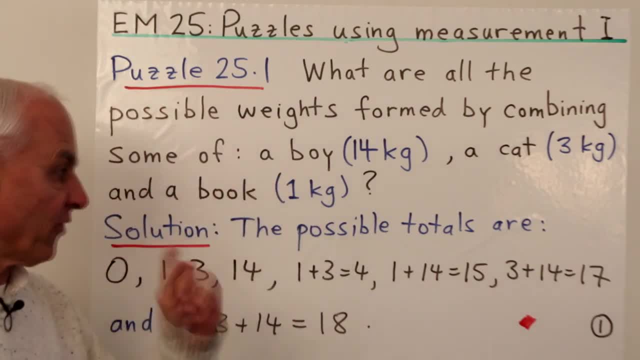 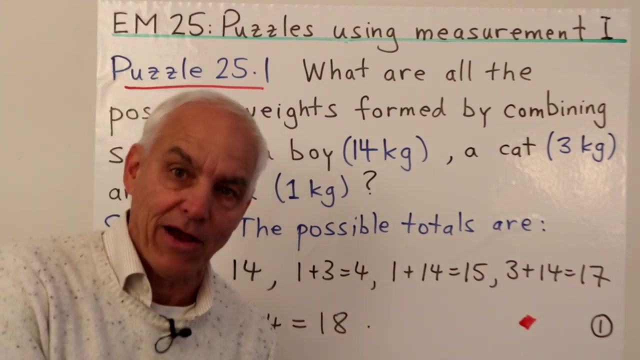 have a number of additions to do. the possible totals are- and I've kind of put them here in some kind of reasonably logical order- First of all, the zero solution, when we decide to put none of the objects on the scale. Now it's maybe a question of debate whether 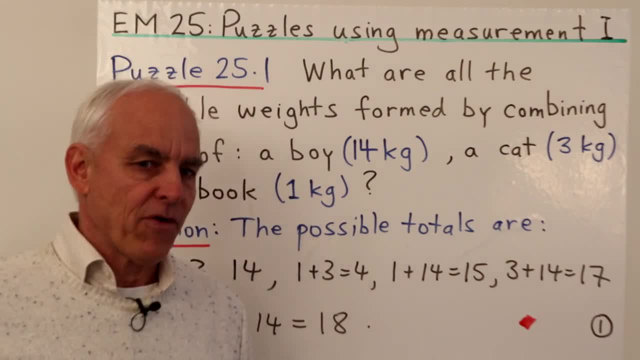 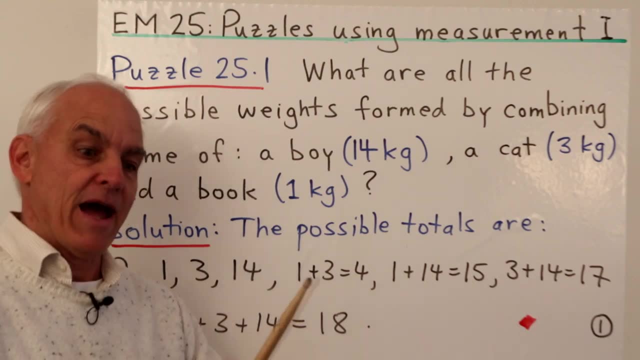 we should include that as a possible answer or not, And from the purely mathematical point of view, it turns out that it makes more sense to include that as part of the solution overall. Okay, so we're gonna put zero there as the first possible weight that we can. 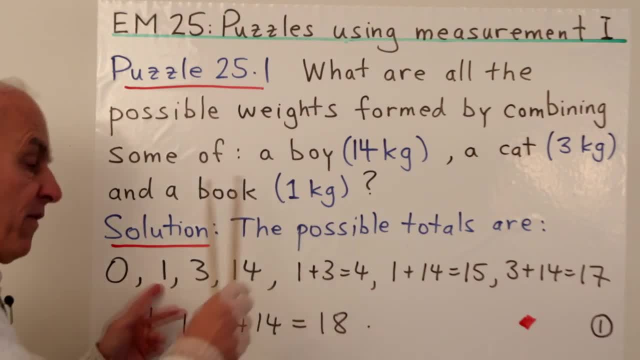 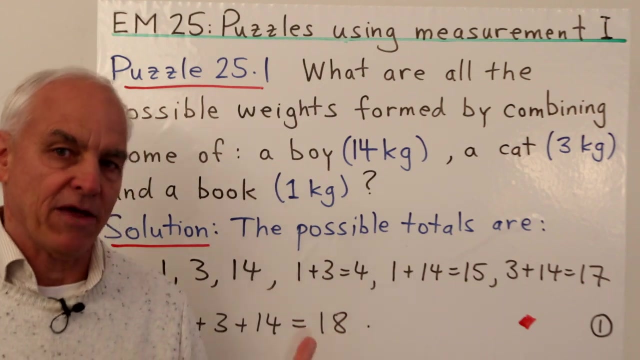 get. The book by itself gives us 1 kilogram. the cat by itself gives us 3 kilograms. the boy by himself is 14 kilograms. So those are possible weights that we can get rather obviously, And then we can weigh two of them together at a time, The book and the cat, making total weight of 4.. The 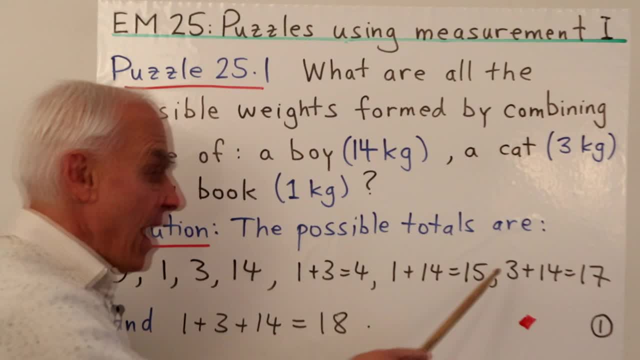 book and the boy total weight of 15, and the cat and the boy a total weight of 17.. But then there's one more possible combination, which is to put all three of them together on the scale, if they all fit, and then we get 1 plus 3 plus 14, which is 18.. So there are eight possible solutions. Okay, and 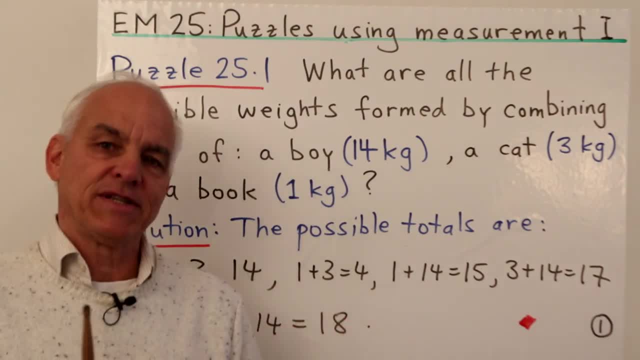 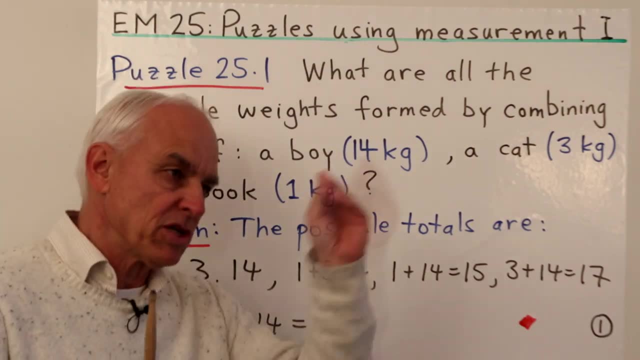 here they all are and I've presented them in a sort of systematical way. That's something that we want to emphasize to the young children, that when we're doing this kind of problem we shouldn't just be thinking: oh, that's a possibility, that's a completely unrelated possibility. now We 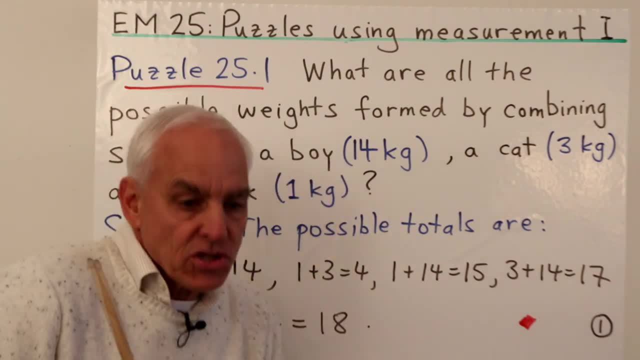 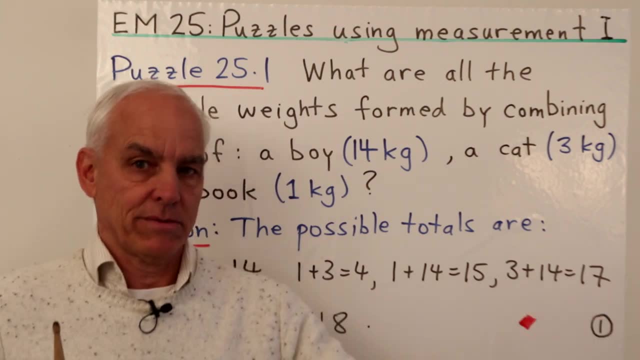 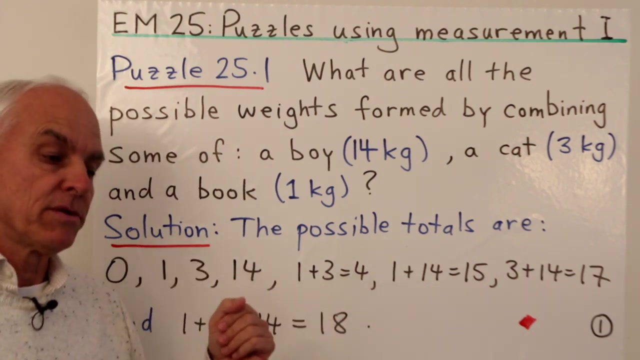 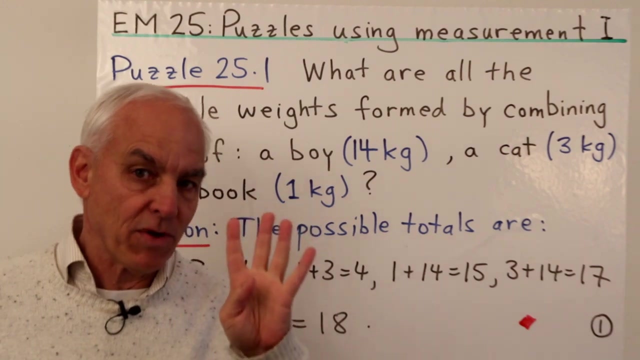 want to organize right. we organize the solution starting from the simplest ones and then working our way forward gradually, step by step, in an organized fashion. And if you have a more advanced student or an older student, then it's logical to proceed one more step and try the same question with four different weights. Okay, you have to be. 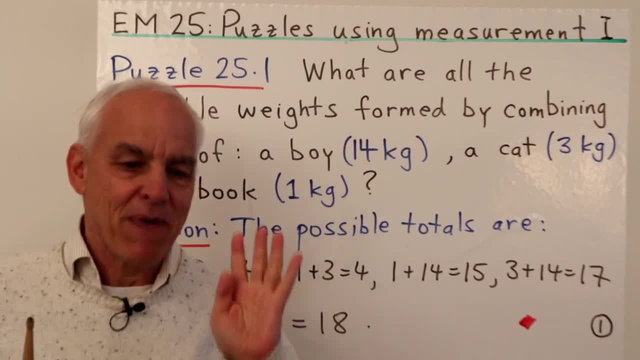 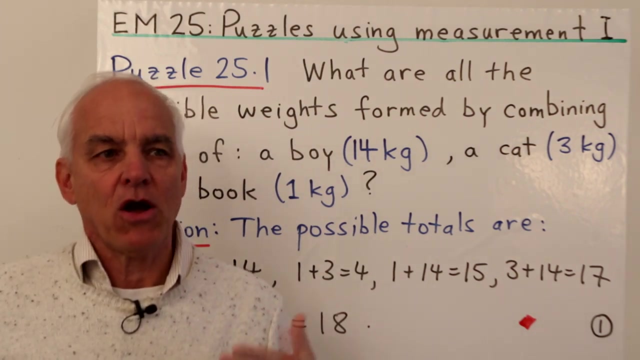 a little bit more systematic there and there's a lot to learn by doing doing that question with four weights systematically and writing down all the solutions. So maybe I'll make this point also that when we're doing these kinds of puzzles, it's not always cleverness that we're aiming for. We're 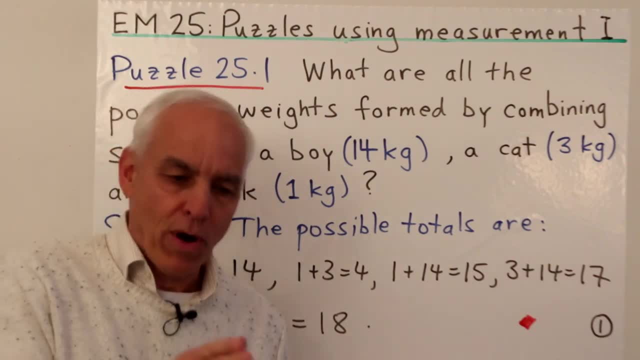 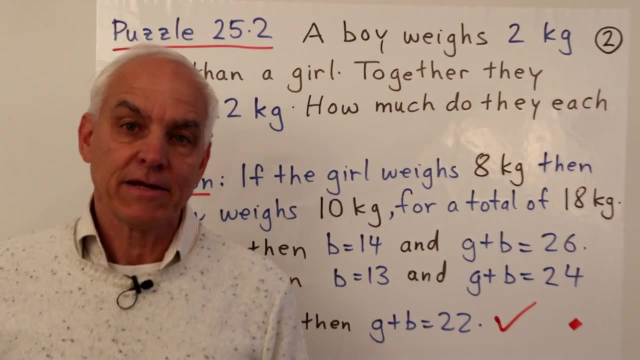 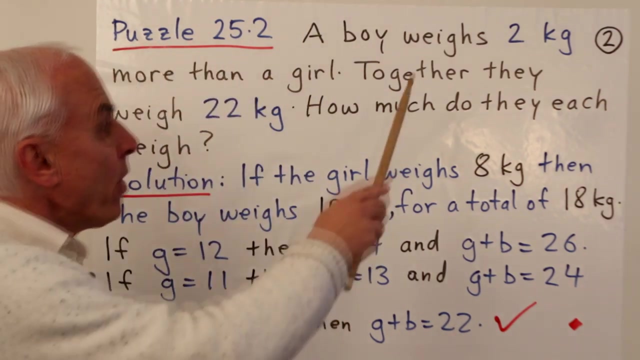 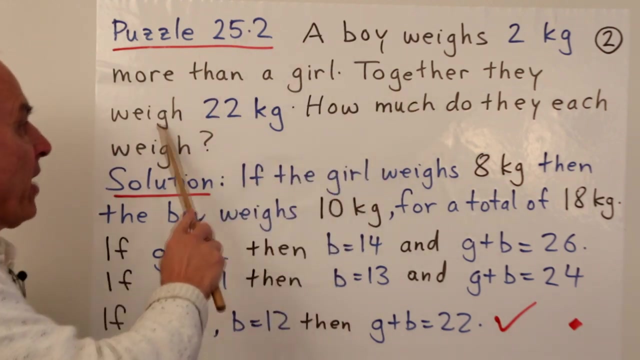 also aiming for systematic thinking, Organized, systematic, step-by-step thinking. All right, so our second puzzle: we're also weighing things, in this case a boy and a girl, and we are told that the boy weighs two kilograms more than the girl, And we're also told that together they 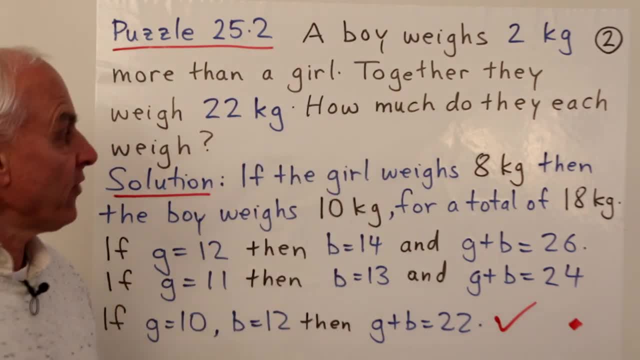 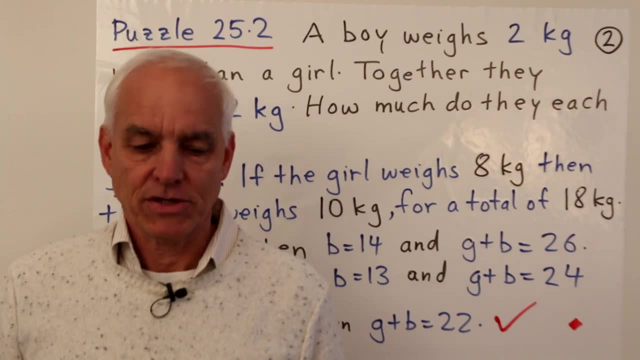 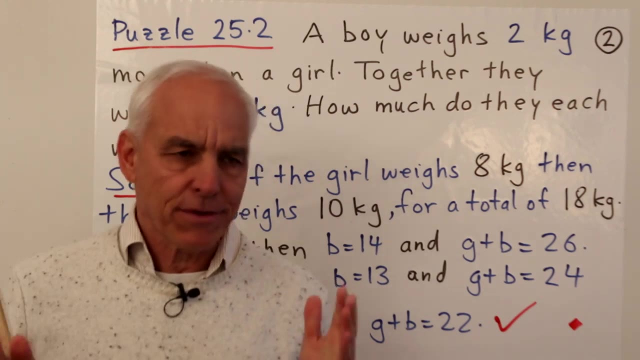 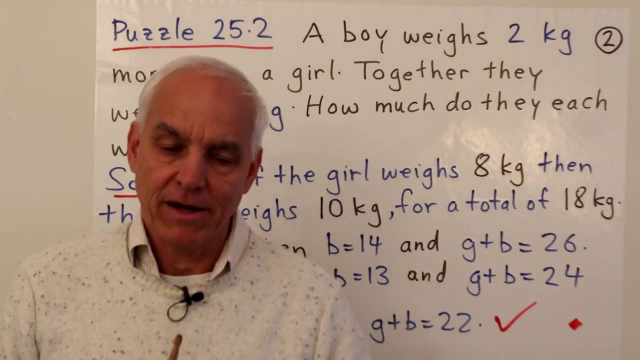 weigh 22 kilograms, And the question is: how much do they each weigh? So this is a nice question. So how do I want you to teach your young children how to think about such a question? Later on, when they become more sophisticated mathematically, they'll solve a question like 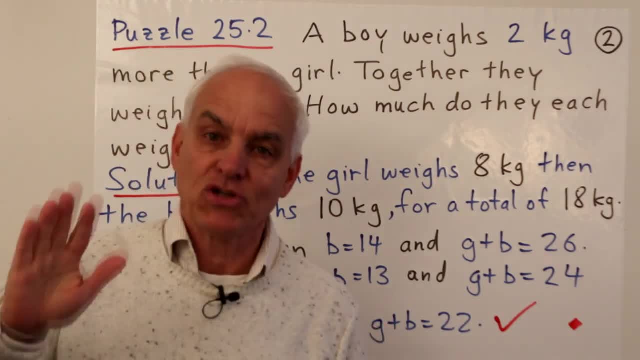 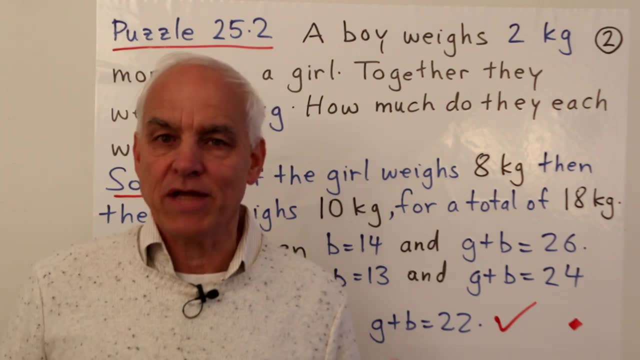 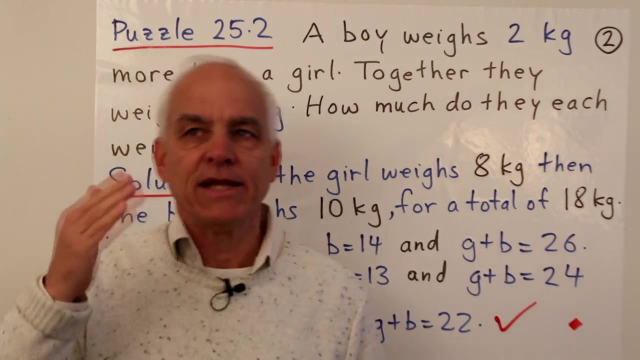 this by introducing variables and doing equations, But that's actually quite a lot further down the road. We are nowhere near doing that right, So we do not want to present a solution that looks at all like that. What I want you to do is to approach this in a kind of a common sense, almost. 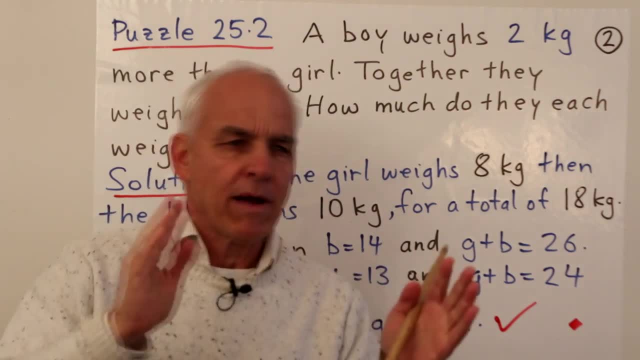 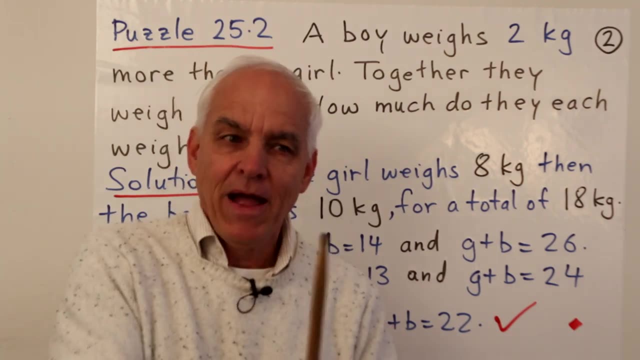 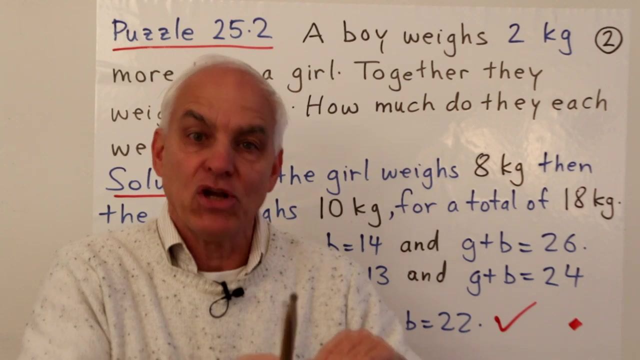 trial and error fashion. You know what approximately would be a reasonable guess. Let's see what happens if we guess something and determine whether the result is lower or higher than what we're aiming for And then adjust the guess correspondingly. This is a kind of a strategy. 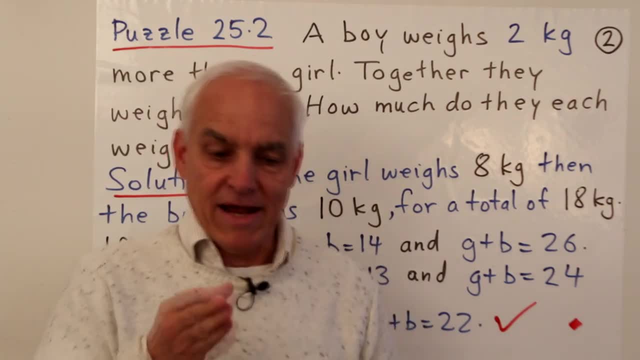 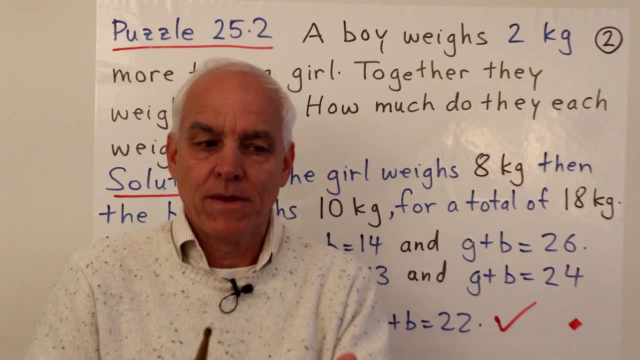 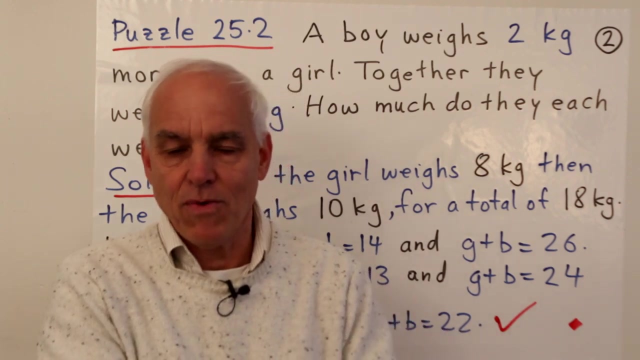 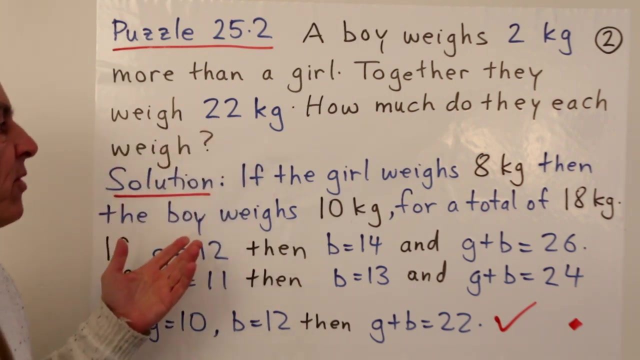 underlying here, which is actually very important, to make an estimation, see what happens with that guess and then adjust the guess the next time around, depending on where your initial answer lies with respect to where you want to be. so let's illustrate that here. so together they're going to weigh 22 kilograms, so maybe the girl weighs. 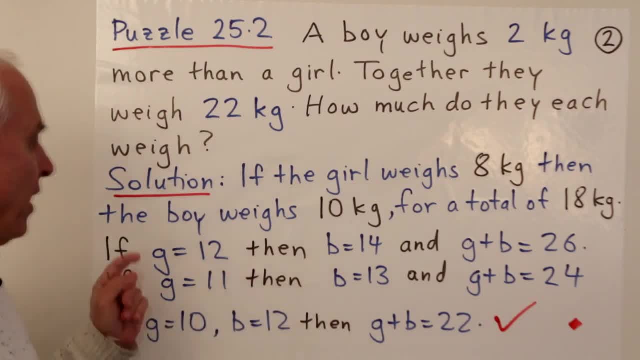 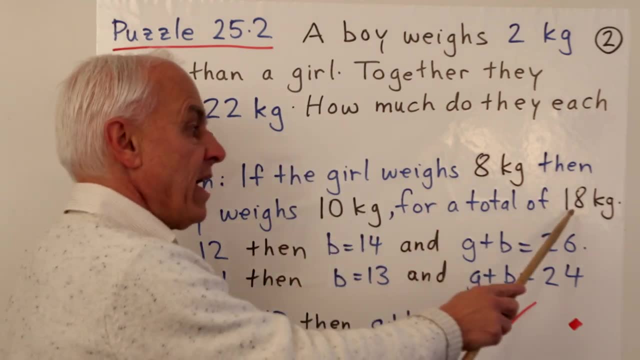 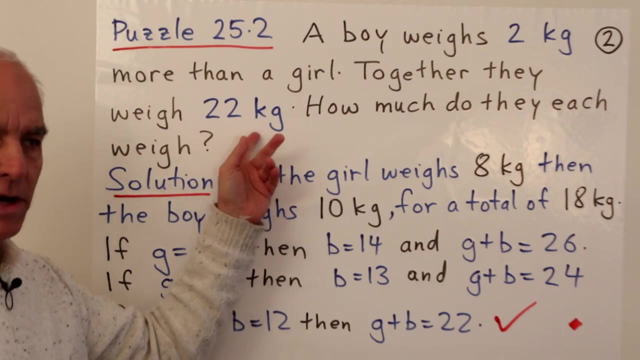 eight kilograms. in that case, the boy would weigh two more, which would be ten, and their total would be ten plus eight, which is eighteen kilograms. okay, that's under what we're looking for, right? so we have to have a sense of order. we have to realize that 18. 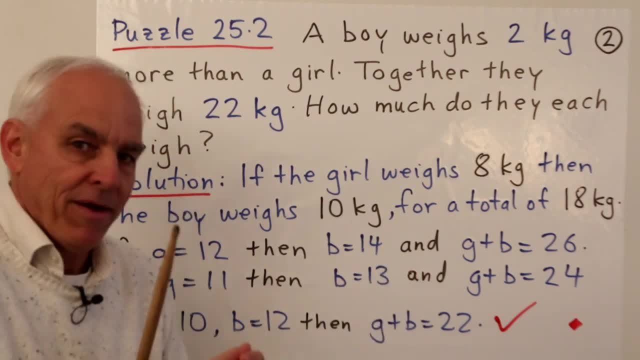 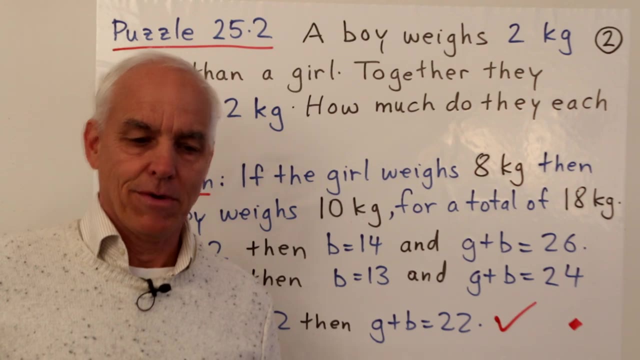 is less than 22.. so we want to up the weights of the boy and the girl. okay, so let's try something bigger. how about if the girl weighs 12 kilograms? and I'm going to introduce this little shorthand: if G equals 12? okay, so G stands for the weight of the girl, but we don't have to. 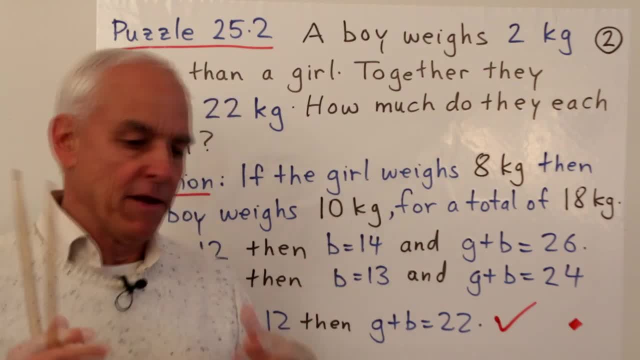 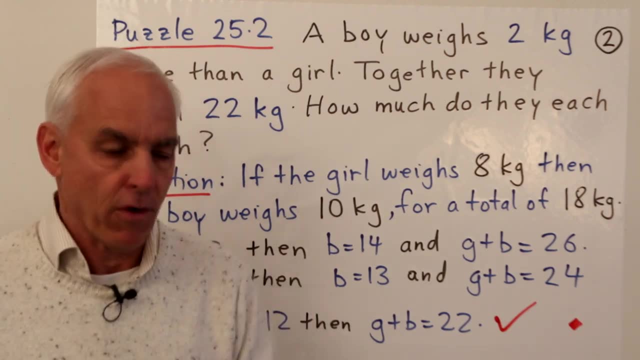 be too formal about that. we could just write that down informally. so the student starts to see how we're using a little symbol to represent what it is that we're looking for. so if G is 12, the girl weighs 12 kilograms, then the boy 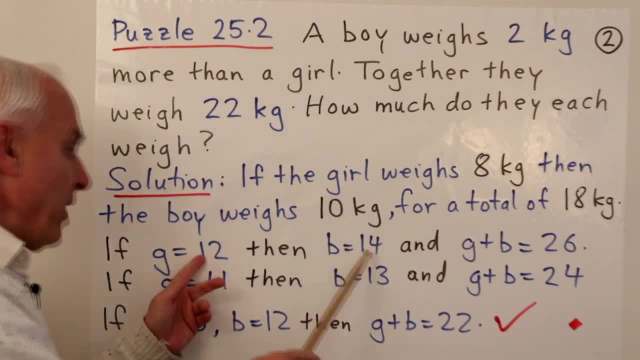 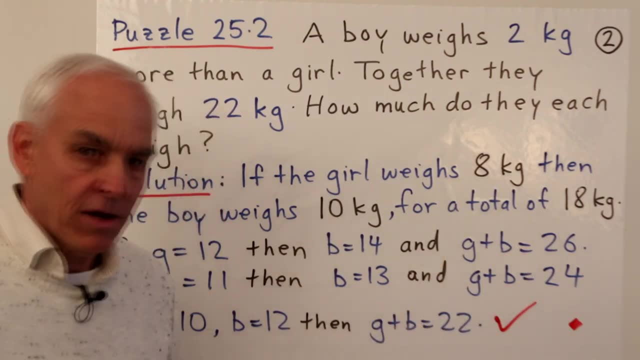 will weigh 2 more, which is 14, and then we have to do a bit of arithmetic, we have to somehow add these two things and hopefully we can do that one way or the other and get a total of 26. comparing that with 22, that's too high. so we 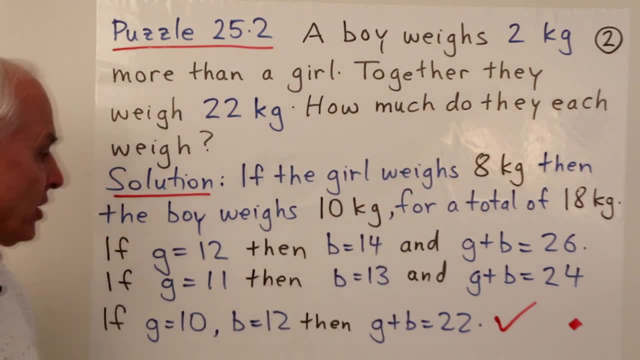 started too low, now we're too high, okay, so we have to adjust. so let's go down a little bit. if G equals 11, the B equals 13 and the sum is 24. still a little bit too high? let's go down a little bit further. if G equals 10, then B equals 12, then G plus B equals 22. ah, that's. 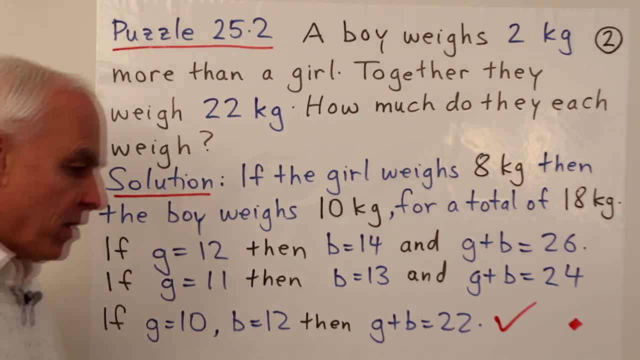 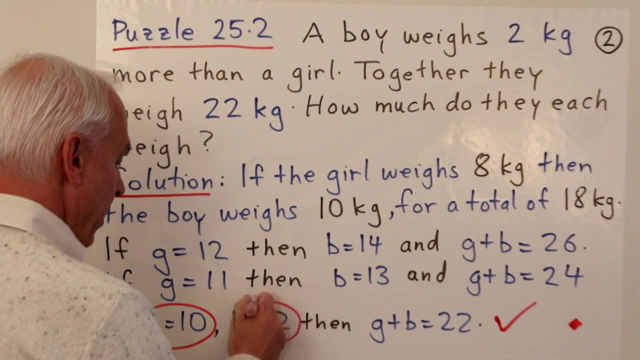 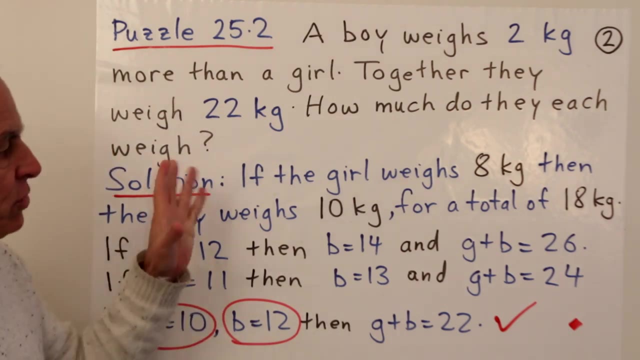 great, that's exactly what we want. so the answer is: G equals 10, the girl weighs 10 and the boy weighs 12 kilograms. now I've chosen certain numbers here, okay. so the numbers that I've chosen I think would be sort of suitable for sort of a mid-level student in the age bracket we're. 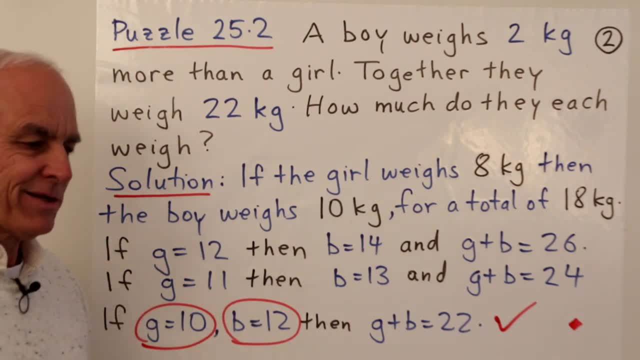 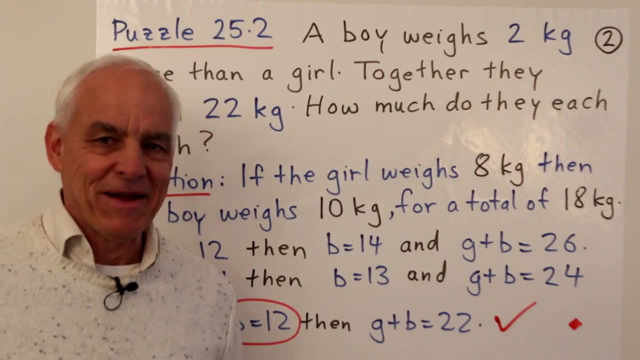 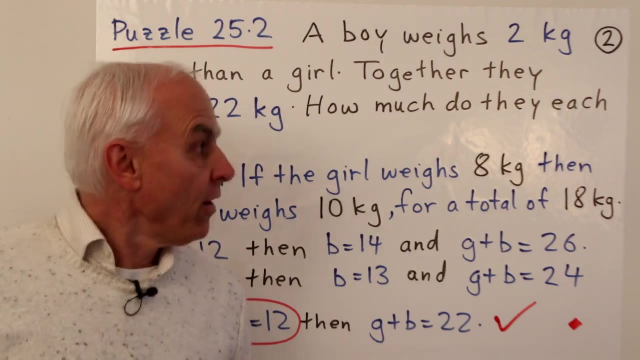 thinking about. but if you're starting with a very young child, these numbers are perhaps too big, right? so you would want to give them a version of this puzzle which has smaller numbers. so you have a kindergarten child, okay, you want to ask them a question like this. well, you could simplify it. you could say that: 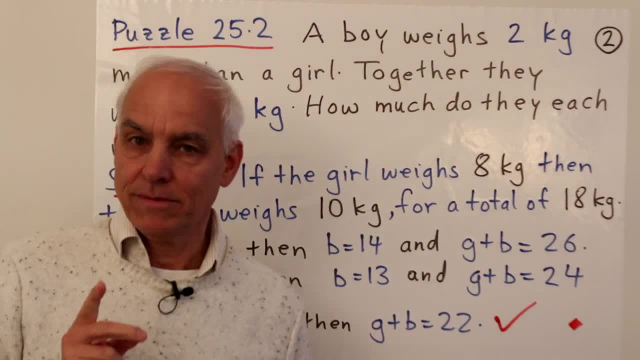 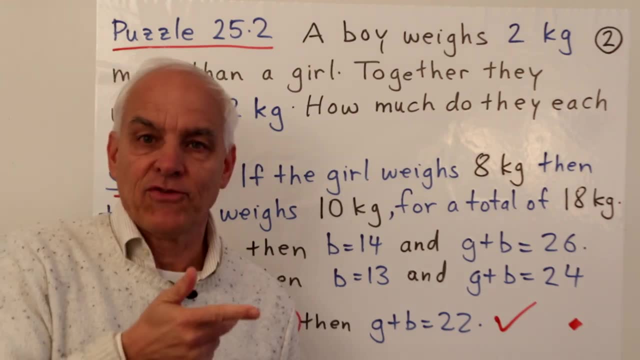 a boy weighs 1 kilogram more than a girl. that's a lot easier, and so in your mind you think: 1 kilogram maybe. maybe one of them weighs 5 and the other one weighs 6. then the total would be 11.. so the question would be: boy weighs? 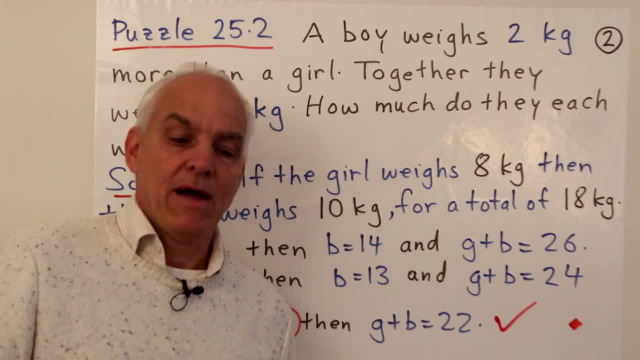 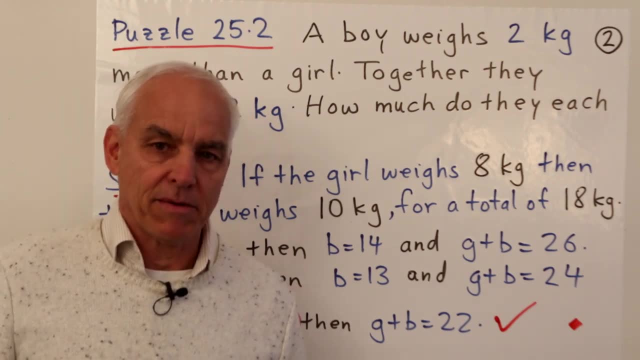 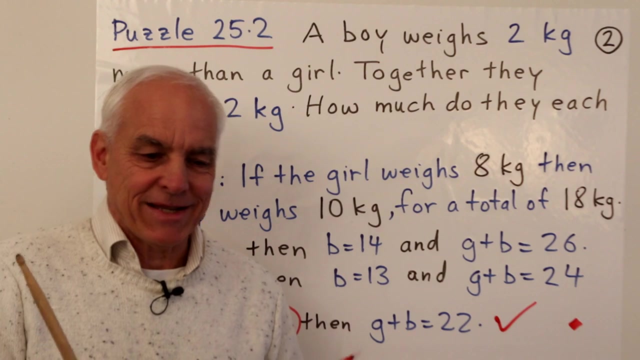 1 kilogram more than a girl. together, they weigh 11 kilograms. how much do they each weigh? okay, oh, that's, that'd be very low total. maybe cats would be more suitable, okay, but anyway, you get the idea that what we want to do is we want to adjust the numbers in these puzzles. 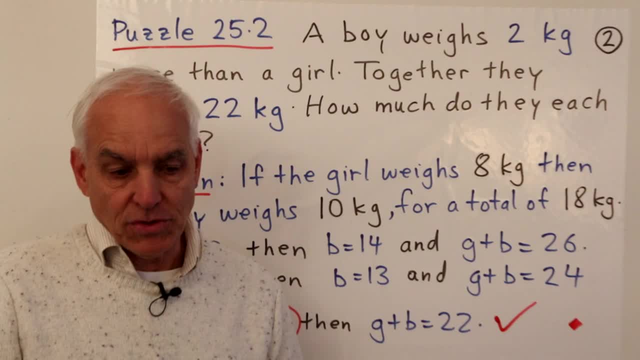 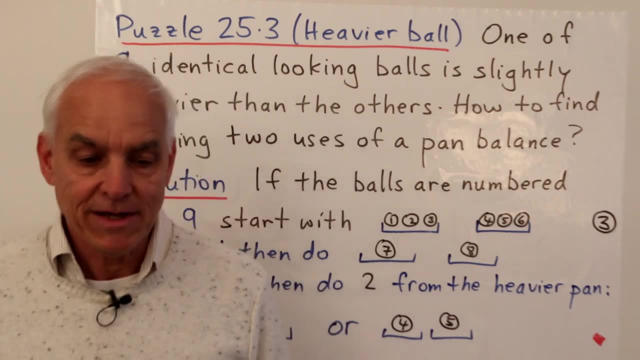 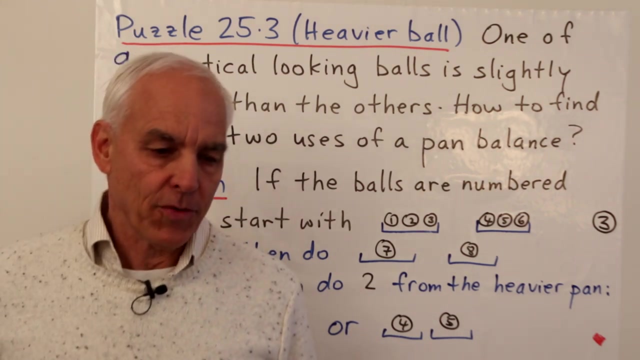 to suit the level and the aptitude and experience of the children that we're talking about. all right, so our third puzzle- might call it the heavier ball puzzle- is a very classical uh puzzle that's uh familiar and has a lot of different variants also. so again, there's additional kinds of questions in the same direction that we could ask and in: 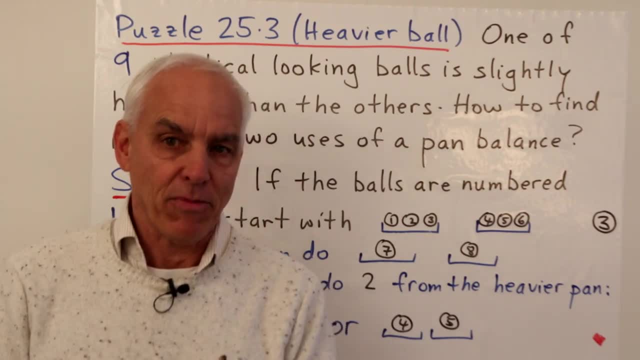 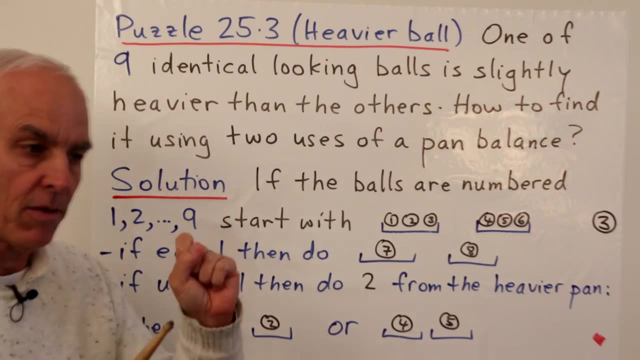 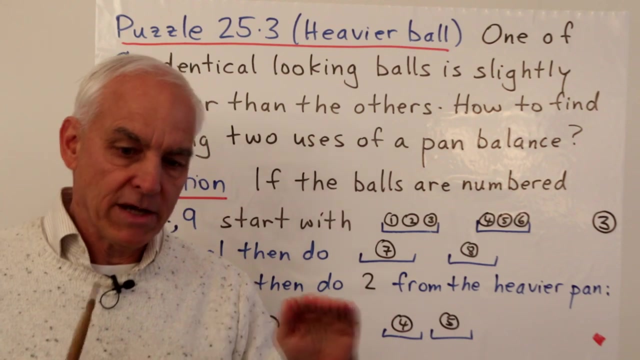 the course that I'm designing, there will be lots of other examples in this kind of direction. so the idea is that we've got nine identical looking balls and one of them is slightly heavier than the others. the others are all the same weight, but one of them is heavier than the others. but 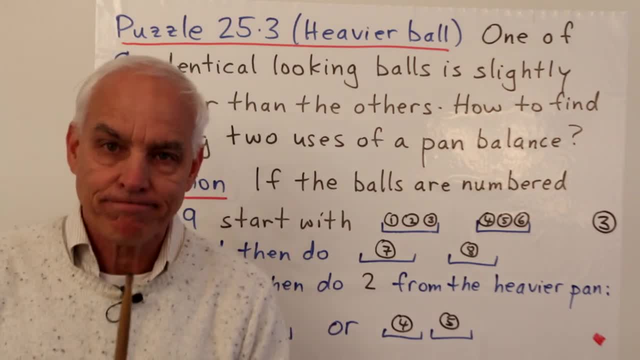 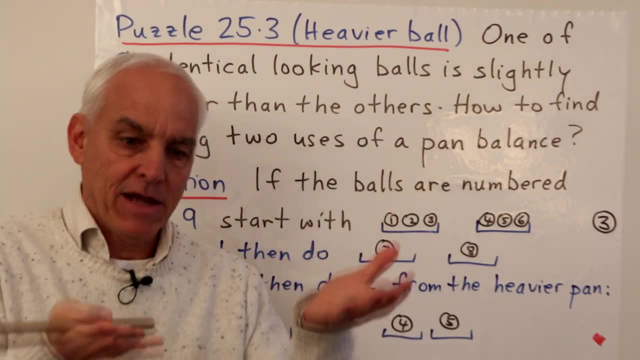 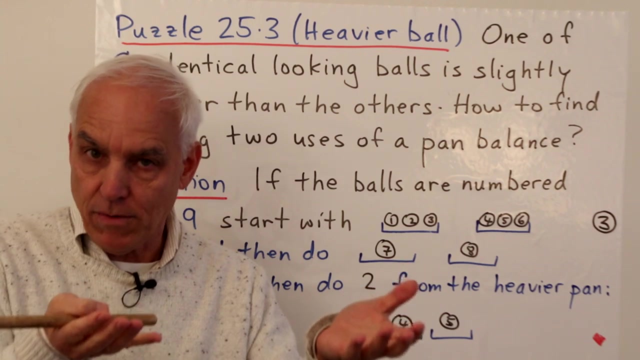 we don't know which, because they all look exactly the same. now we're trying to find that heavier ball and what we have is a pan balance. okay, so we're able to put things in two pants and see which one is heavier or whether they're equal, and we're trying to determine the heavier ball. 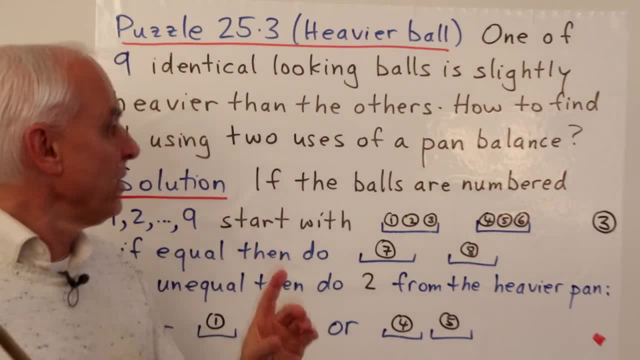 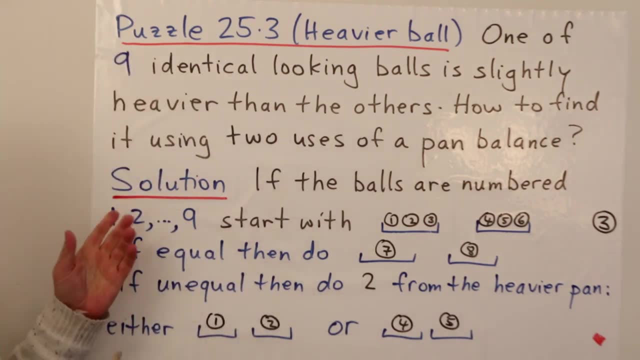 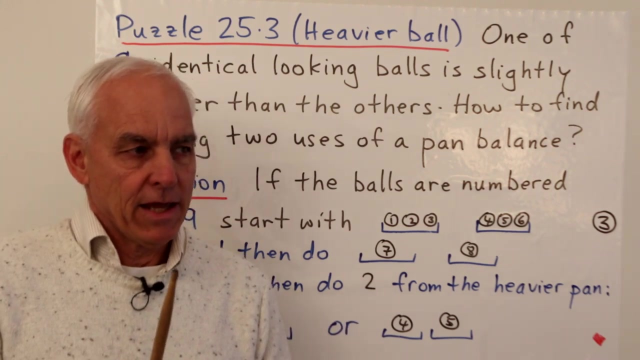 using exactly two weighings, two uses of the pan balance. okay, so this problem is already a little bit- you know- extensive it. it involves a fair number of things. there's nine balls, so it's not a bad idea probably to start this kind of investigation with a simpler example, sort of 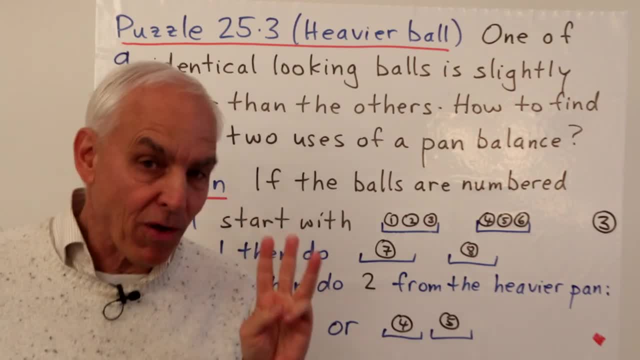 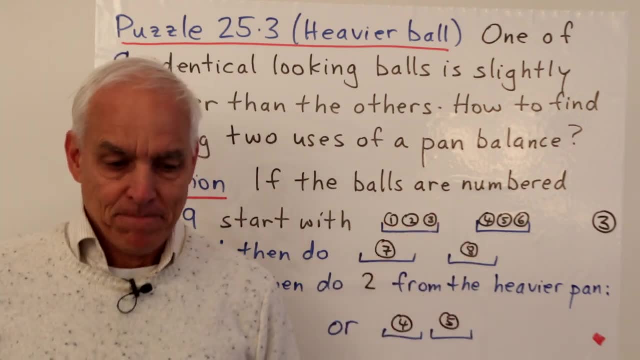 you know. so the simpler example would be what happens if you have three balls and one of them is heavier. okay, so let's just think about that one first, because that's actually involved in this one. okay, so if you have three balls, let's call them one, two, three, okay, and uh, one of them is heavier. 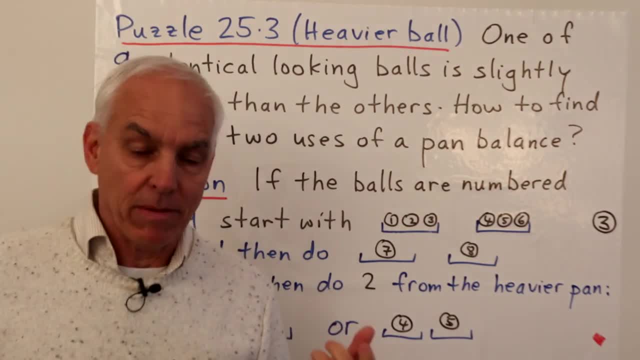 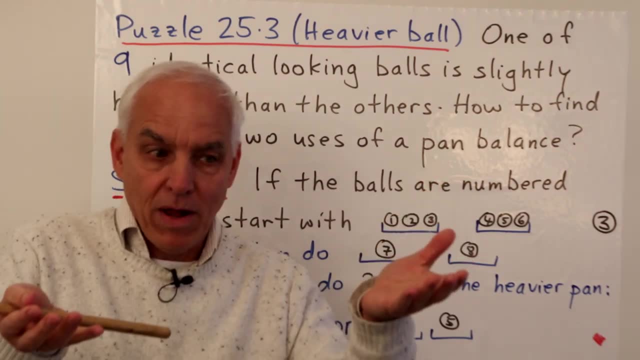 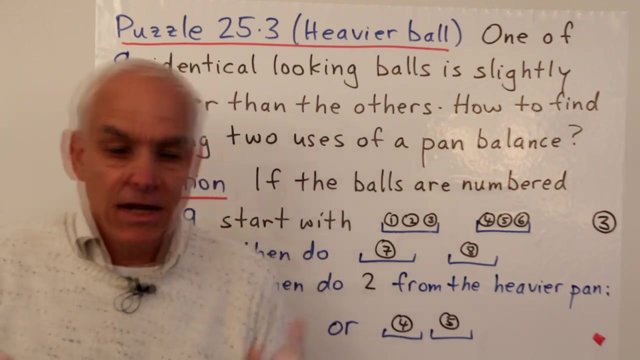 but you don't know which one. what you're gonna do is: you can take two of those balls, say ball number two, put them in the pan balance and if they are equal, well then those are the two equal balls. it must be that the third ball, number three, is the heavier ball. on the other hand, if they're not, 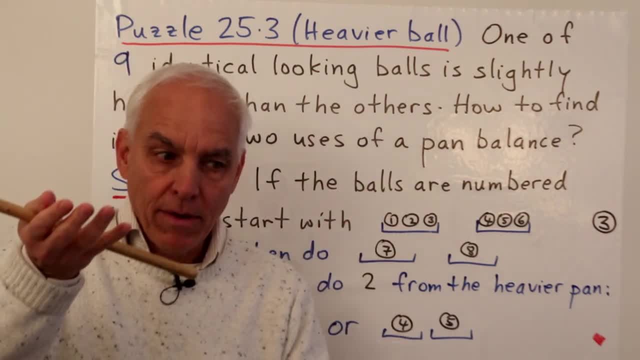 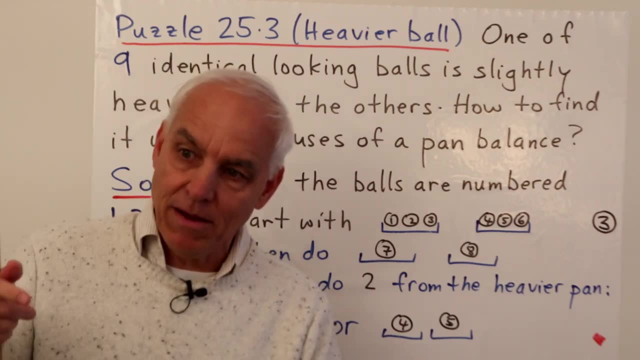 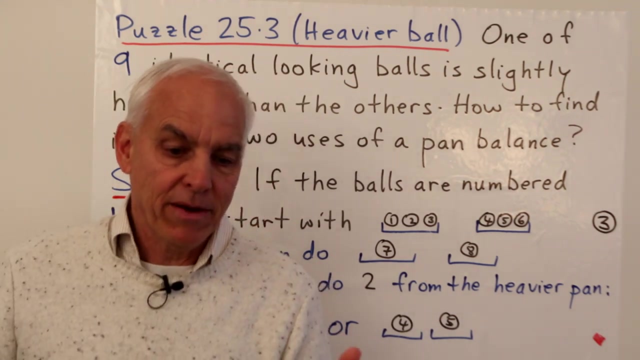 equal. say, one is heavier than two. well then, the one is heavier than two, and so one must be the heaviest ball of all three, because we know that the two lighter balls have the same weight. okay, so we determine the heaviest ball if we just have three of them, okay. so that's a kind of a 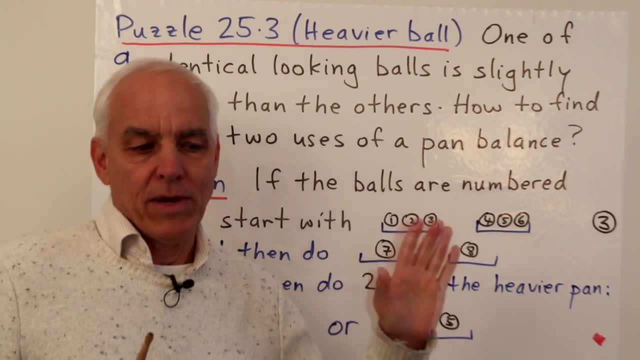 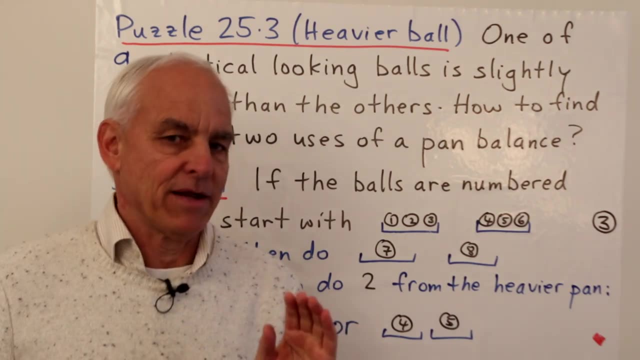 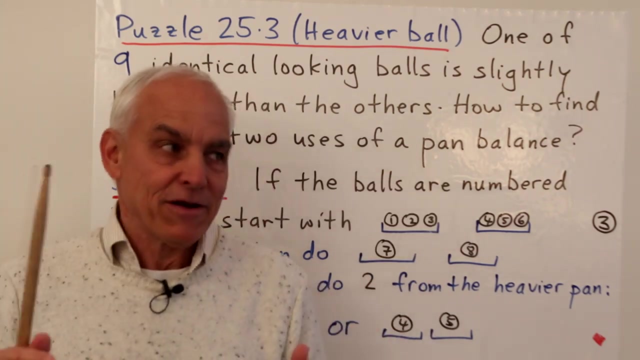 preliminary that we can do first before we tackle the main puzzle. but if you have a clever child maybe you don't need to have that discussion beforehand. you can let them work that out as part of the puzzle. okay, so you have to kind of assess what what preliminary training you should. 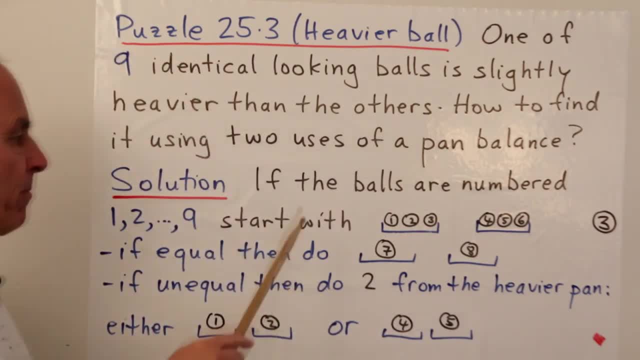 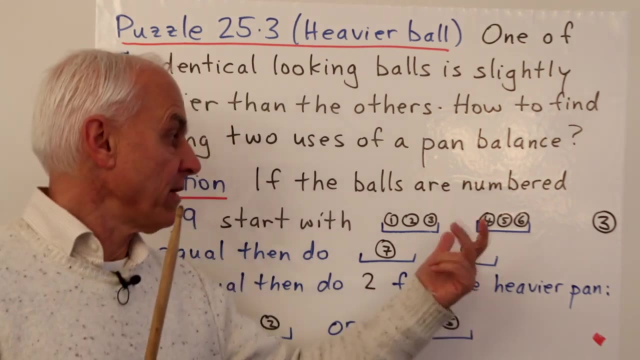 do with your student. okay, so here is our solution now. so if the balls are numbered, say, one, two up to nine, then let's start by weighing with the pan balance: the balls one, two and three in one pan and the ones four, five and six in the other pan. okay, we put them in there and see what happens. 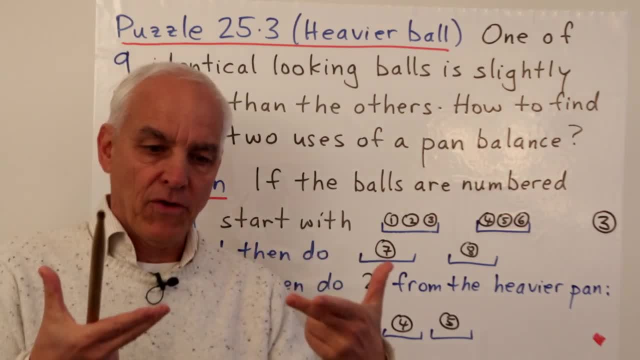 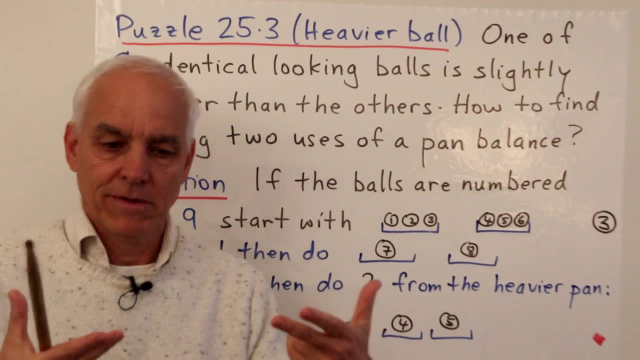 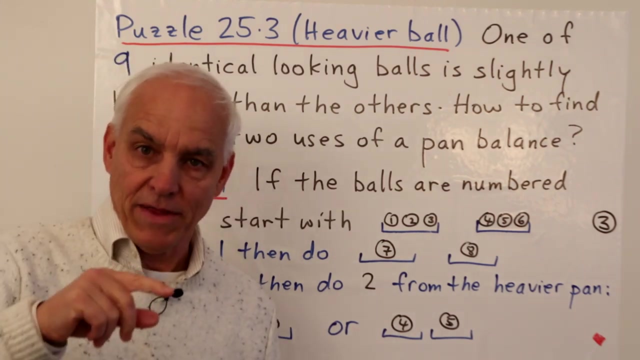 if they are equal, then is that none of these six balls is the heavier one, that we're looking for, none of them. okay, so we can put them aside and concentrate on the other three balls. then we're in that situation that we just were in, that we've solved. so what you do then is you: 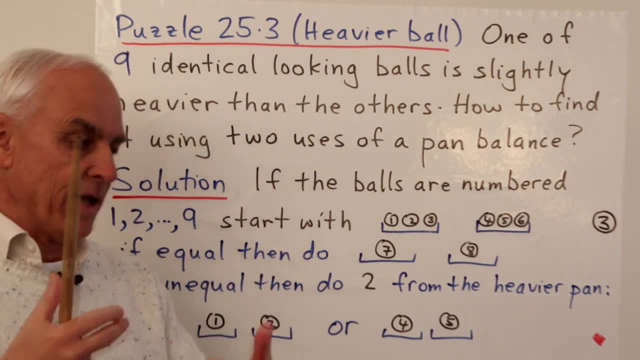 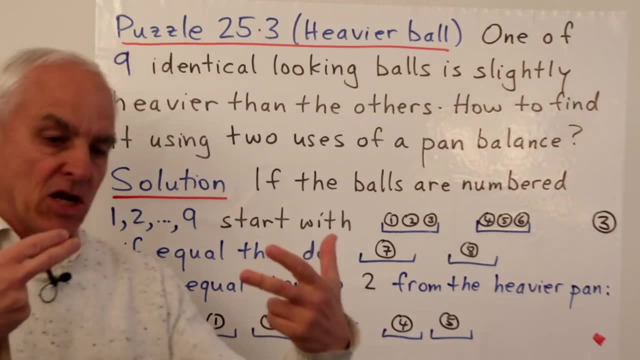 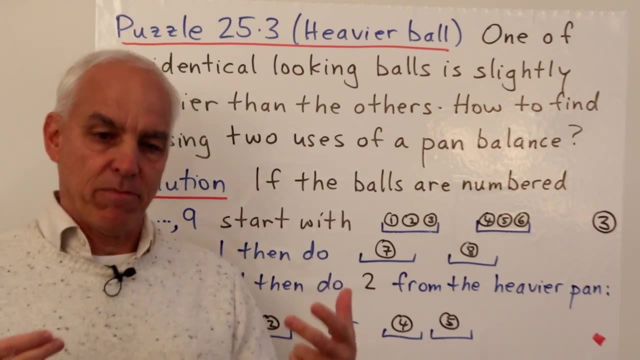 would weigh two of them, say seven and eight, and uh, and quickly determine then which of those three was the heaviest. on the other hand, if the initial groups of three were unequal, okay, then you're going to take two from the heavier pan. so, for example, suppose that the 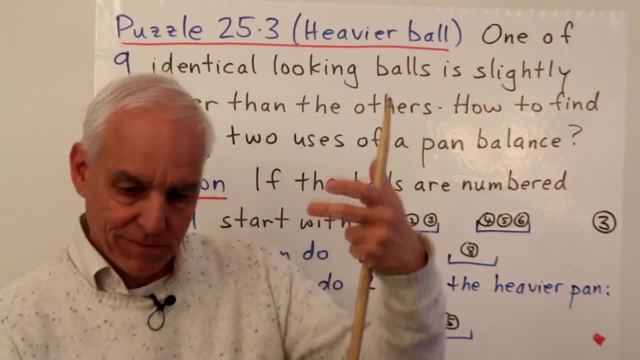 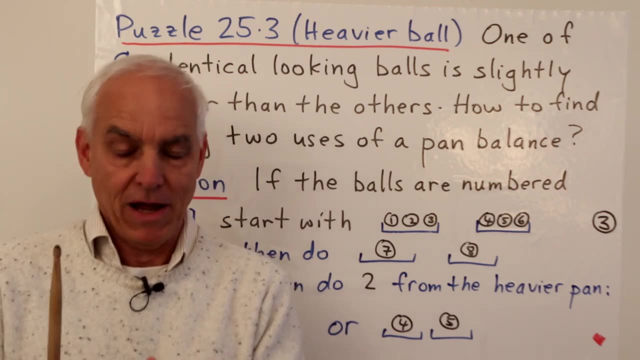 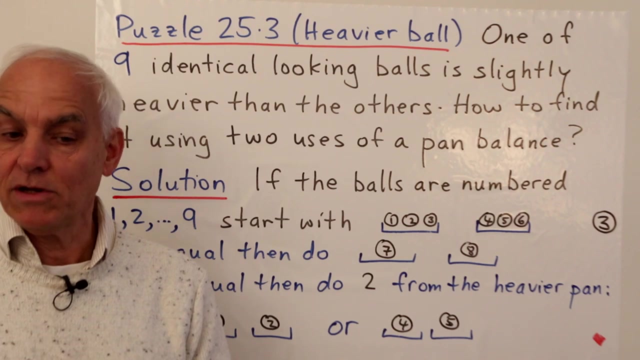 one, two, three pan was heavier: one, two, three. that means that the heavier ball is one of the triple: one, two and three. so again we apply what we've already talked about. we would take two of those balls, say one and two, and weigh them and from that we would deduce which of the three balls is the heaviest. 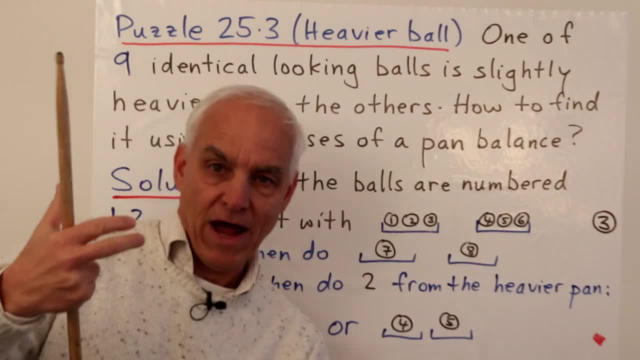 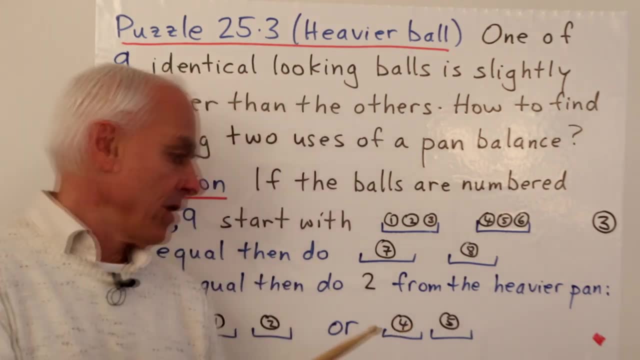 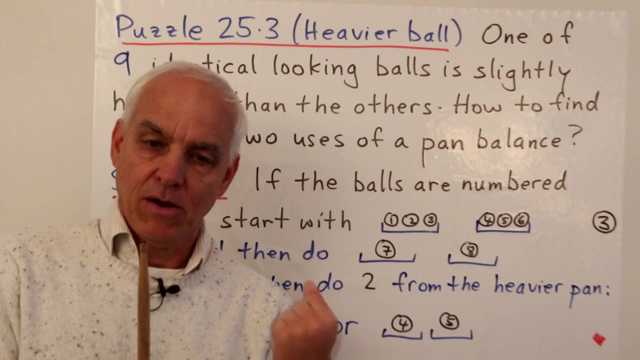 on the other hand, if when we weigh these two sets the four, five and six ball set are the heaviest, then again we would apply the same reasoning to those three balls. take two of them, say ball four and five, and weigh them and deduce which of four, five and six was the heaviest. so we have to kind of go. 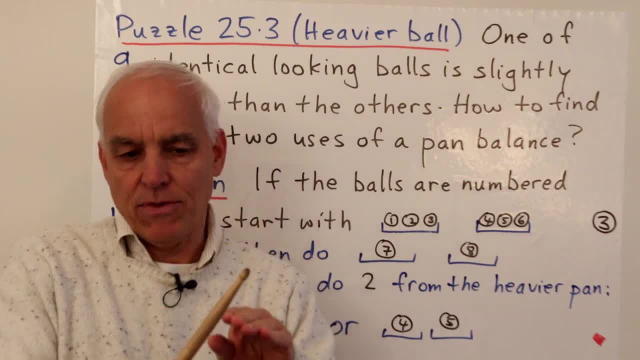 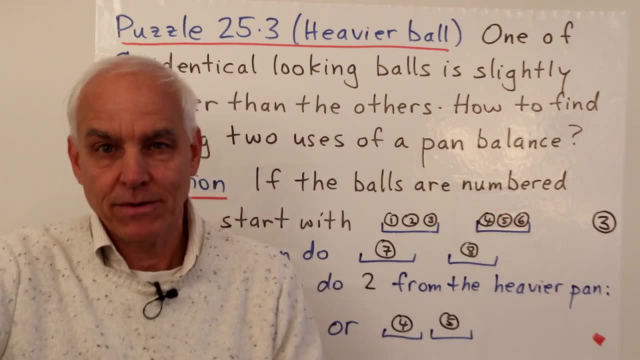 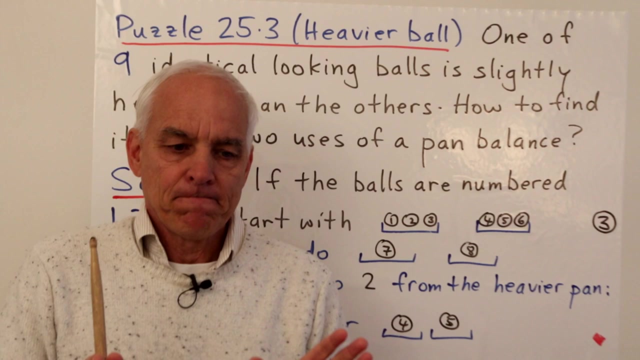 through the possibilities here. it's not exactly a linear thing. it's a more like a tree kind of structure. if this happens, we go in this direction. If this happens, we go in this direction. So this is a great puzzle because it's teaching children the importance of a kind of a logical structure. 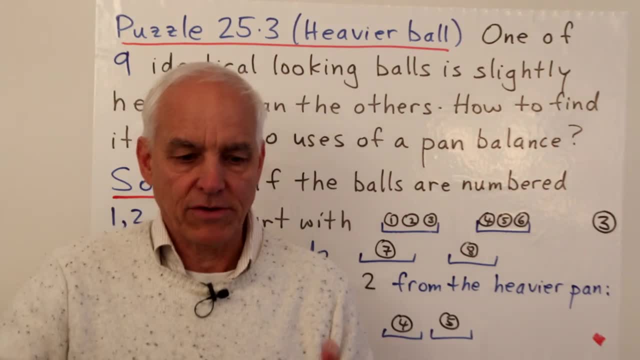 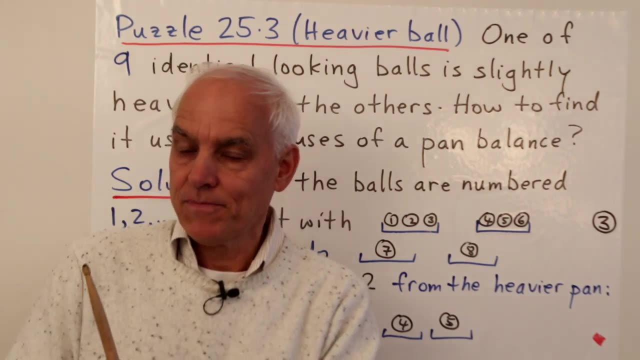 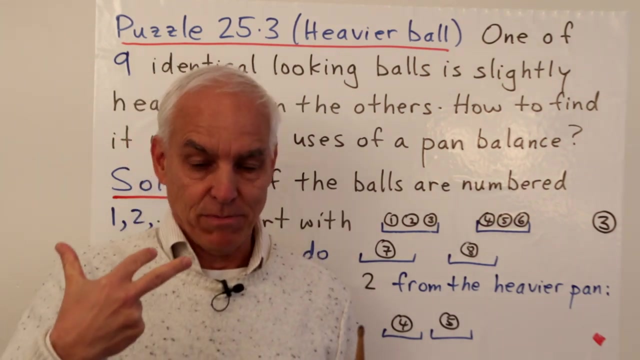 If this we go in this direction. If this we go in this direction. There's different possibilities and we have to deal with those possibilities in slightly different fashions, Although ultimately it comes down to the same underlying idea: that once you know that the heaviest ball is one of three, 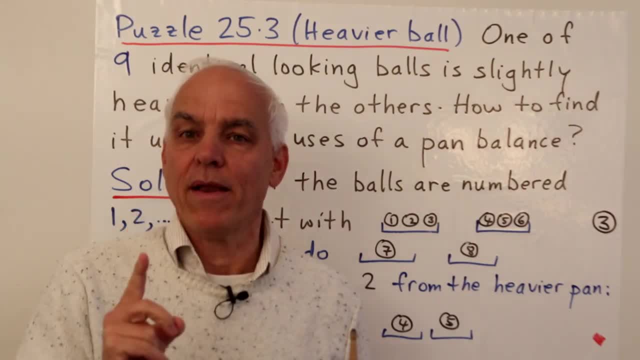 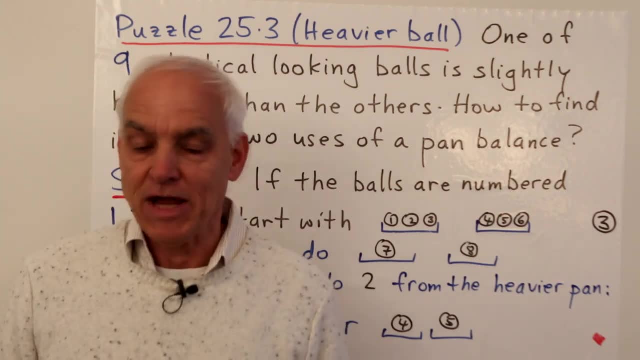 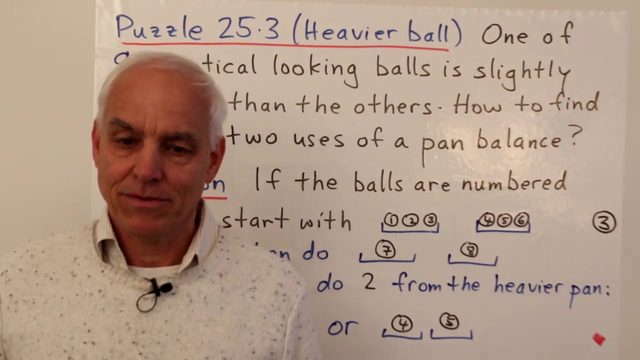 then you can determine which it is with just one way. Now there's all kinds of interesting variants to this puzzle also. For example, you might know that one of the balls is different, but not know whether it's lighter or heavier, Or you could have two of the balls being heavier. 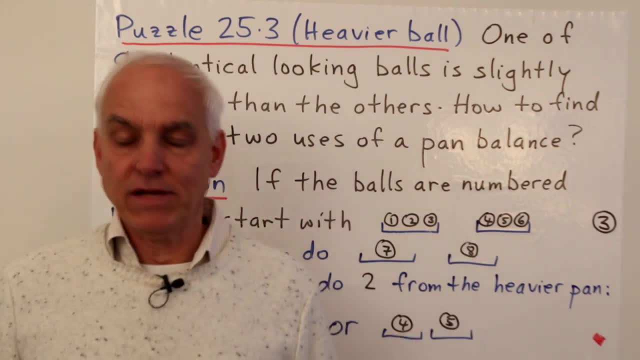 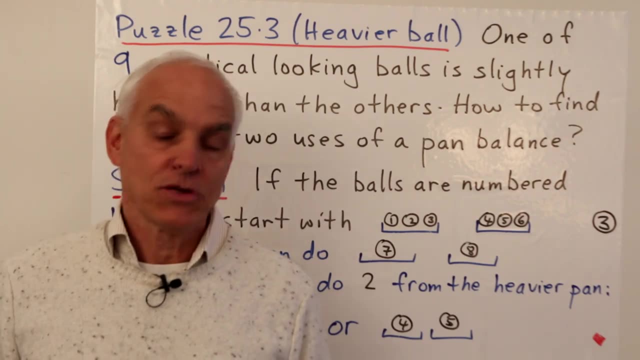 or you could have: instead of having nine balls, you could have 20 balls. There's all kinds of variants that you could discuss in the same direction. So there's a lot of exploring to do behind this particular puzzle. That's why it's such a classic one. 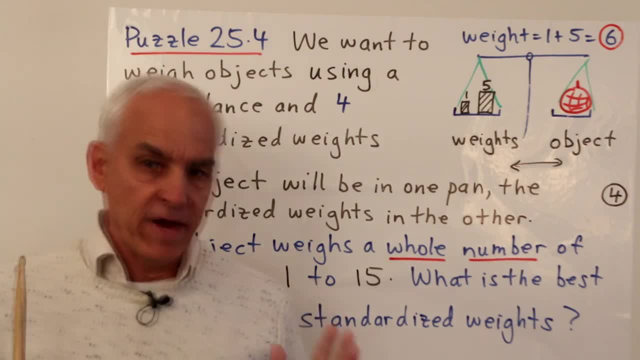 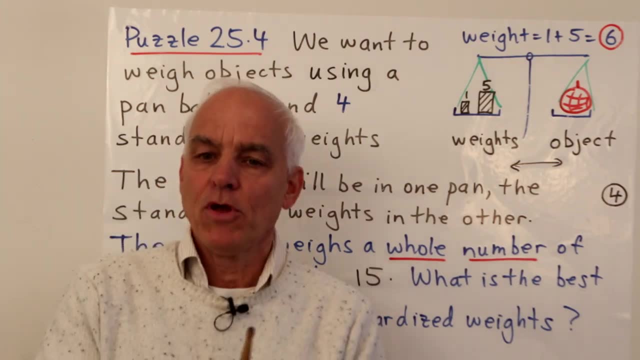 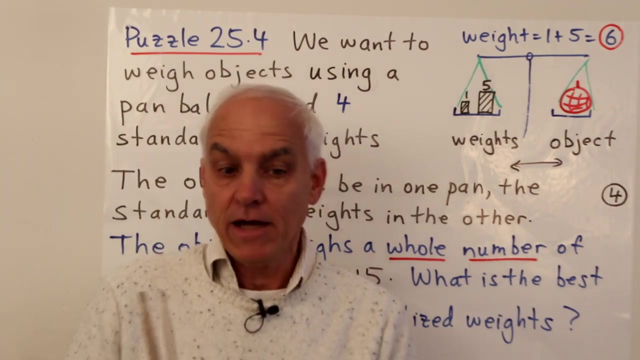 Okay, our next puzzle is also very instructive and actually practically quite important. We can easily convince some young people of the usefulness of being able to solve this particular puzzle And in fact, historically, exactly this kind of puzzle would have been wrestled with. 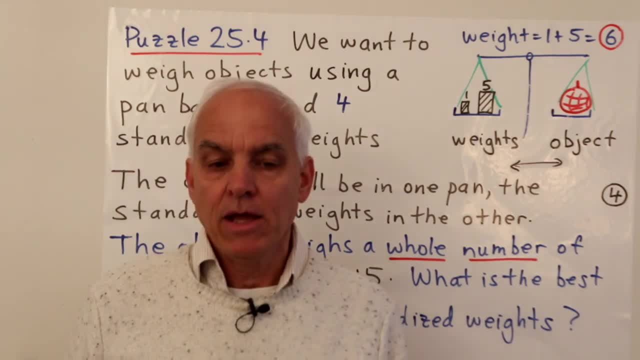 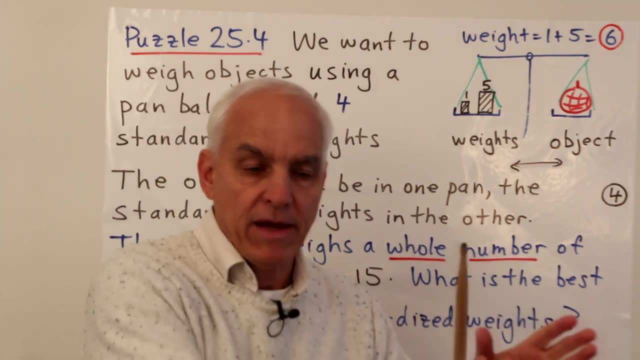 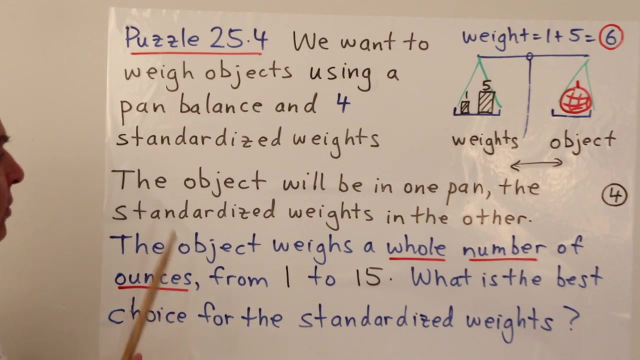 by ancient peoples. We're talking about creating standardized weights in order to be able to weigh things using a pan balance. That's the context. So we want to weigh objects using a pan balance like this and four standardized weights. So we're going to create four standardized weights. 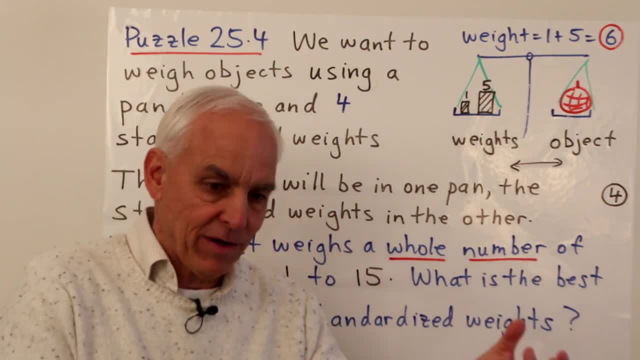 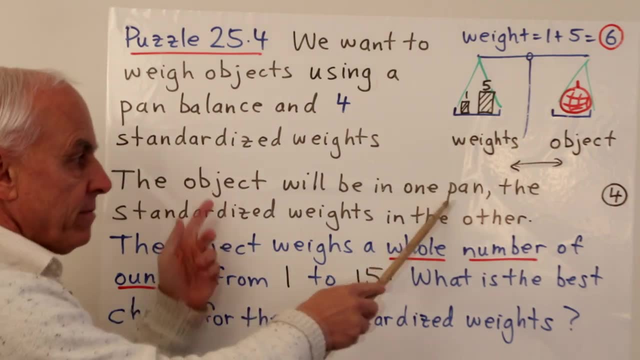 One, two, three, four. We're going to have these four physical weights that we're going to be able to use And we're going to agree that the object will be in one pan, like over here. Maybe that's a tomato or something. 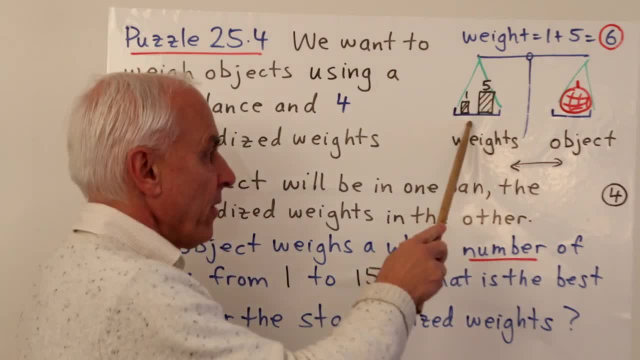 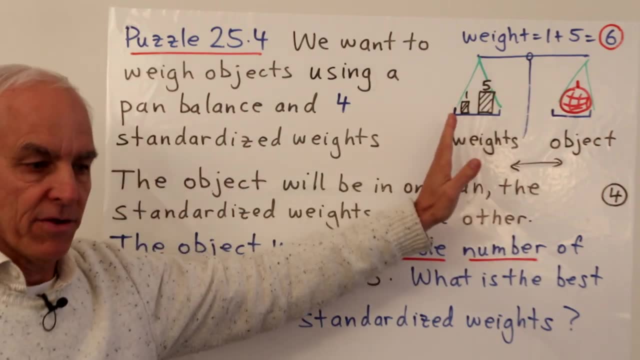 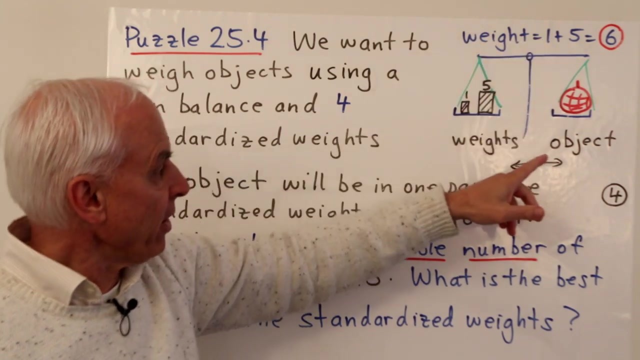 And the standardized weights will be in the other. So object in one pan, standardized weights in the other, And we want to weigh the object. That means we want to create a balance. So in this situation, for example here there's a standardized weight of one. 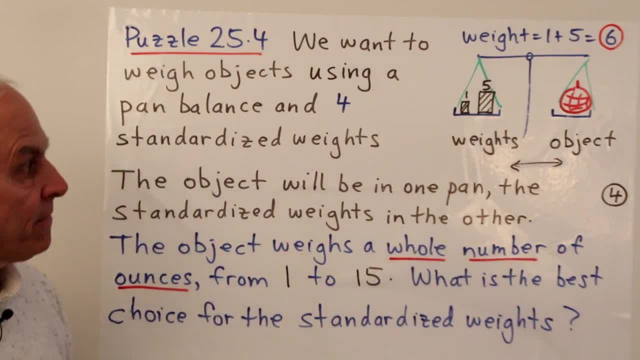 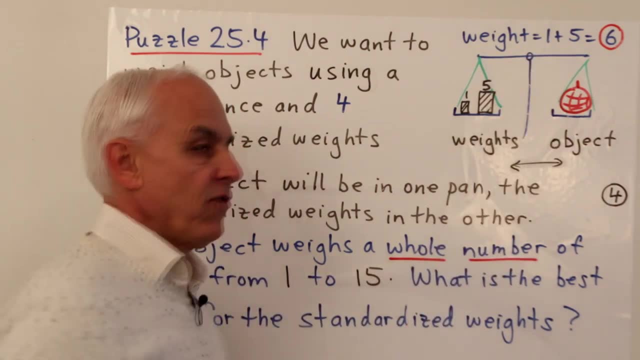 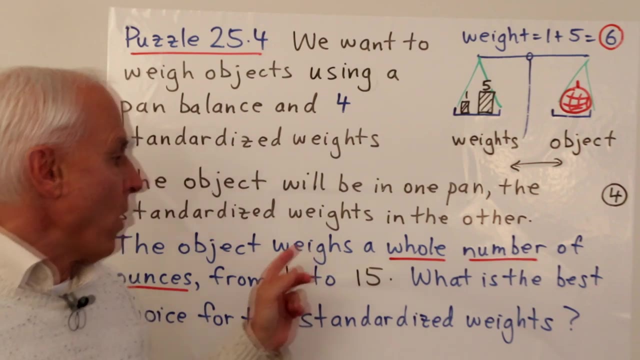 a standardized weight of five in the left pan. So if there's balance, we deduce that the weight of the object is one plus five, which is six. OK, so we're going to assume now that the object that we're weighing weighs a whole number of ounces. 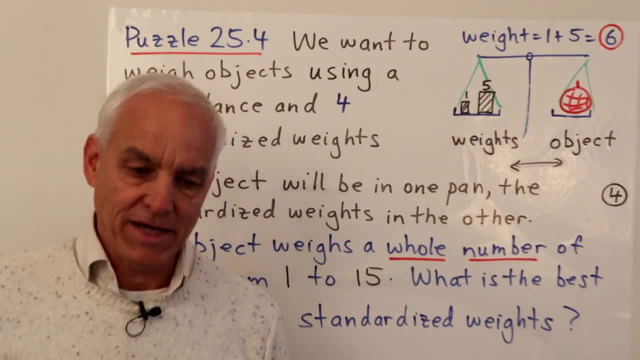 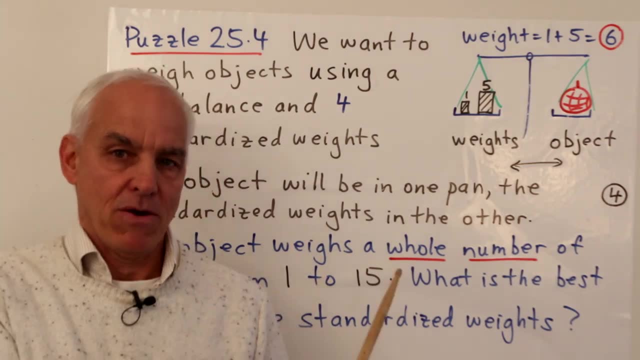 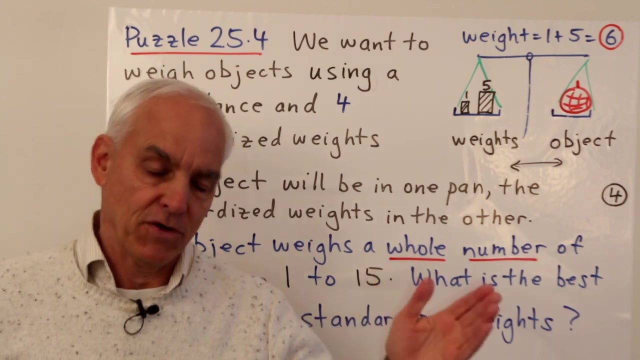 We're going to shift to the imperial or US system Weights. talk about ounces And I remind you that 16 ounces make a pound, And a pound is a little bit less than half a kilogram. You're coming from the metrical system, all right. 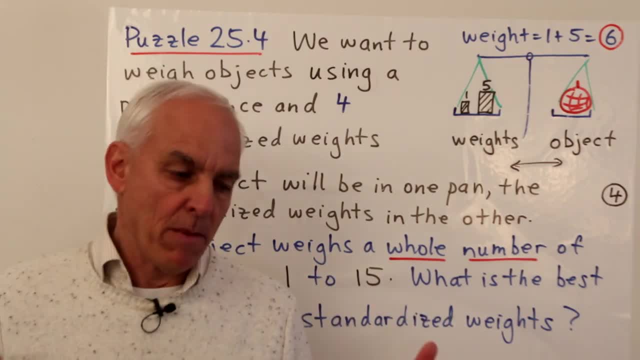 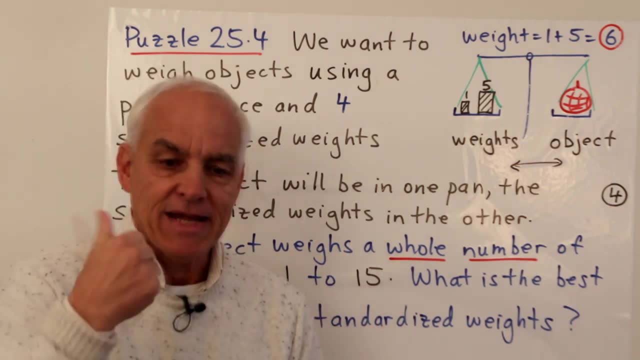 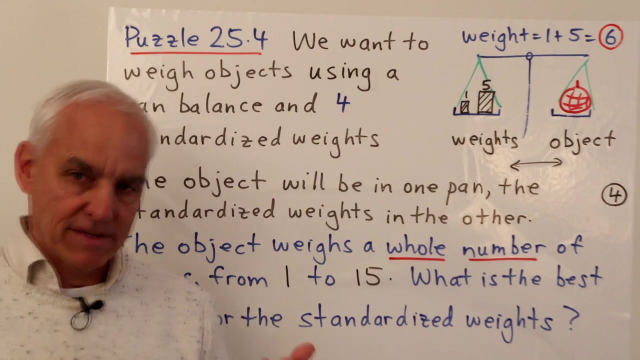 So 16 ounces make a pound, So we're going to assume that we have some object and it weighs a whole number of ounces. So what do we mean by that? Well, it means that it's exactly one ounce, or two ounces, or three ounces, or four ounces. 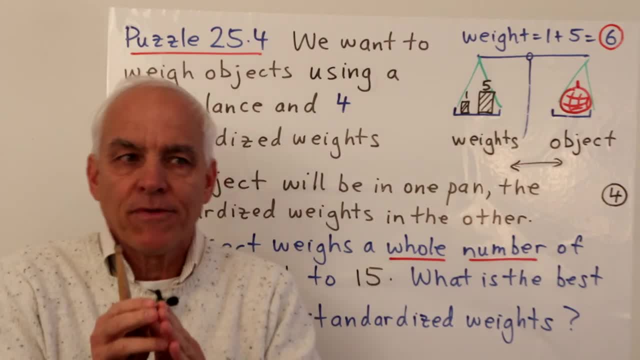 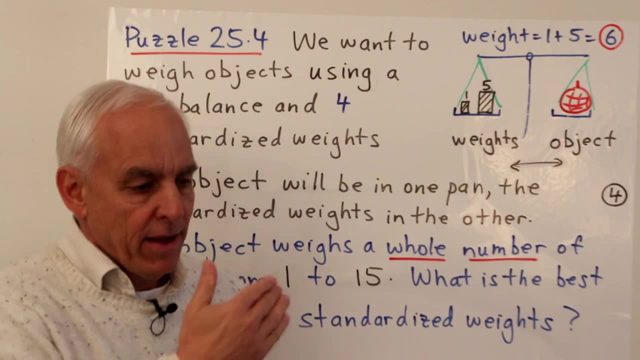 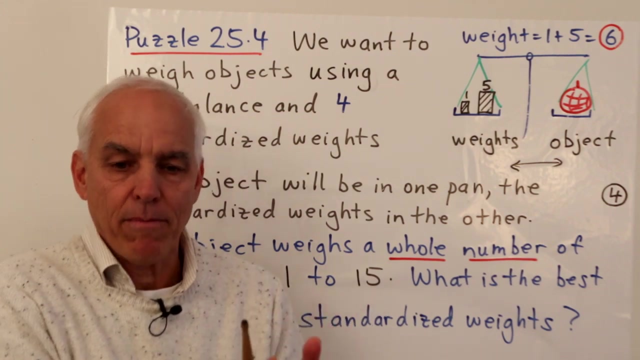 something like that. It's not some fraction between two of those whole numbers. So usually when we weigh things we expect there's a dial and we get some reading which is generally approximate and not exactly a whole number. But we're assuming here that our objects are exactly. 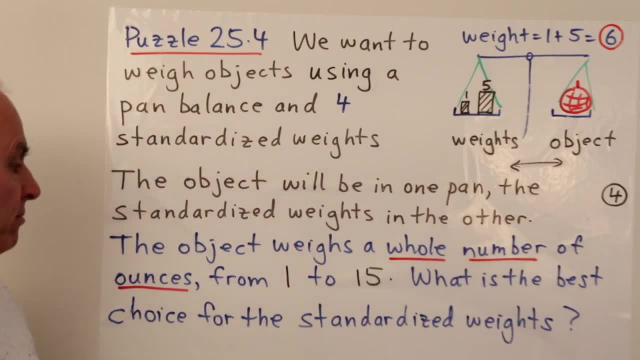 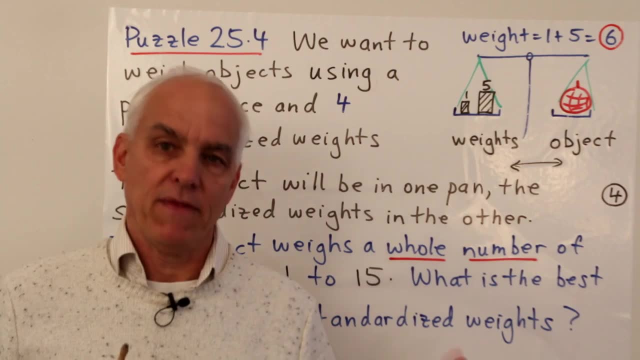 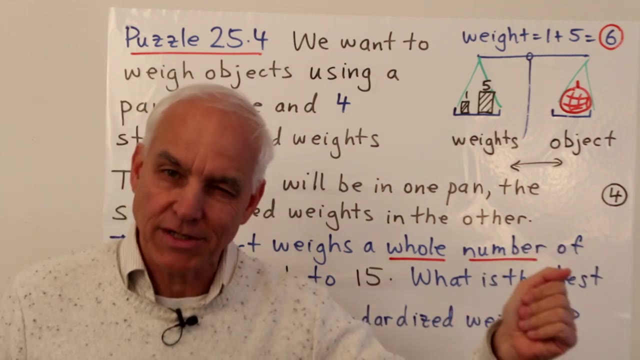 whole numbers of ounces. OK, And we're going to restrict ourselves to the number of ounces that the thing weighs being 1 to 15, somewhere in that range The object could weigh one ounce, it could weigh 15 ounces, or it could weigh any whole number of ounces. 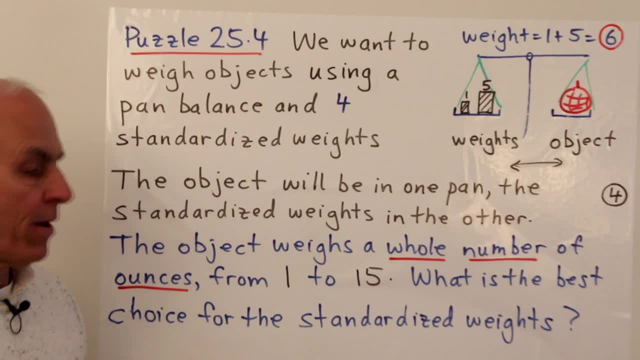 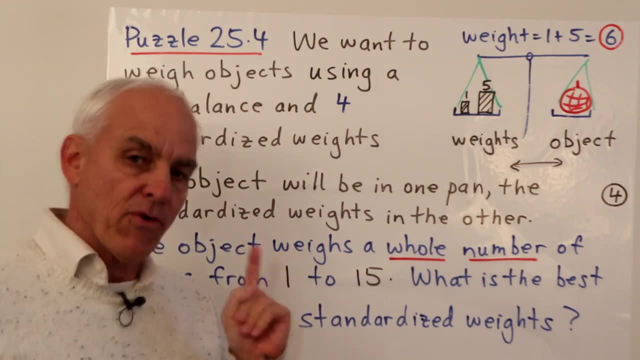 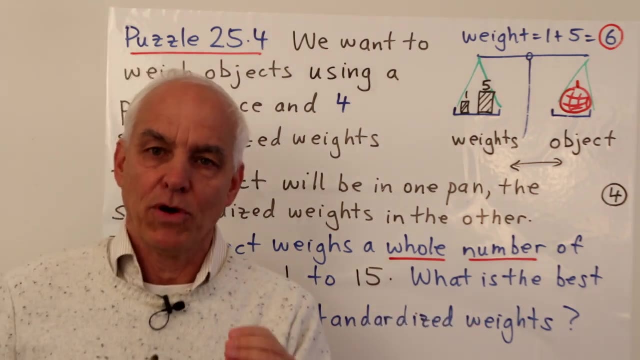 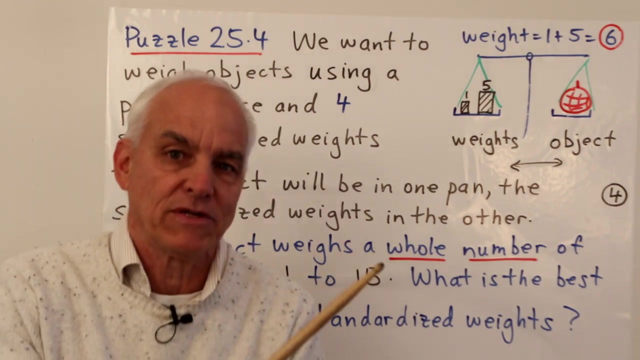 in between that. Now, after all that preliminary, what is the actual puzzle? The puzzle is to figure out what is the best choice for the four standardized weights that we're going to create. We want to create four standardized weights and we get to choose the weights of those four standardized weights. 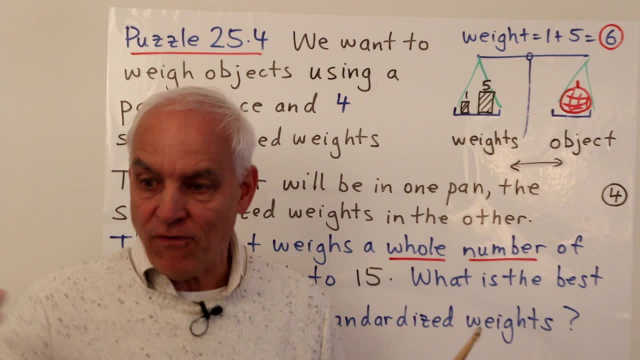 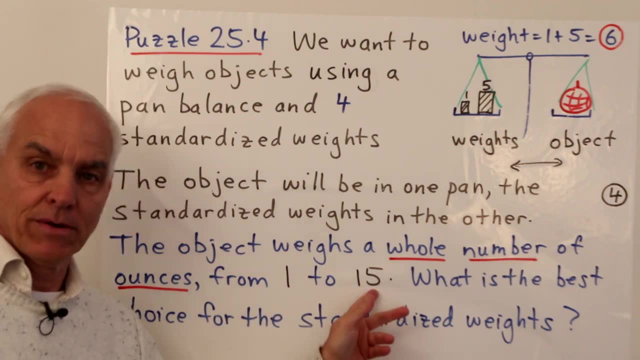 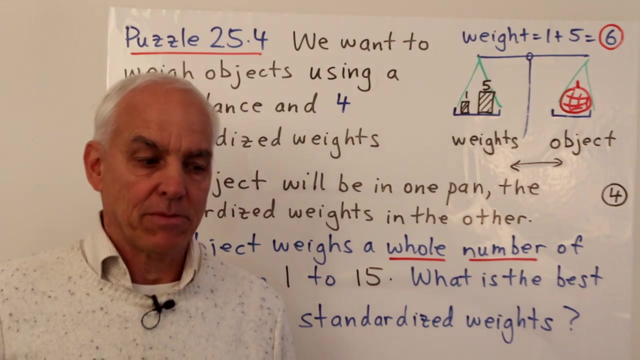 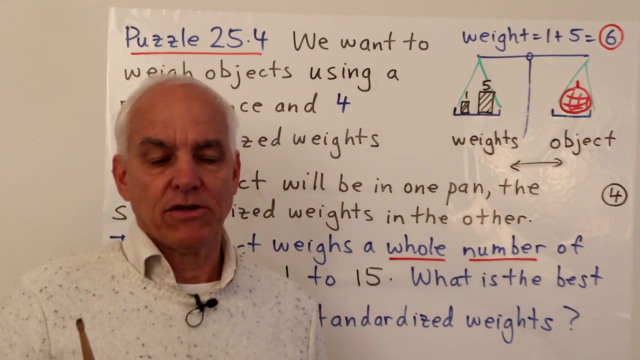 And we want to choose them well so that with just those four weights we are able to weigh any object in this range. So this is obviously an interesting and useful question And, pleasantly, it also connects very naturally with some important mathematics relating to the binary system. 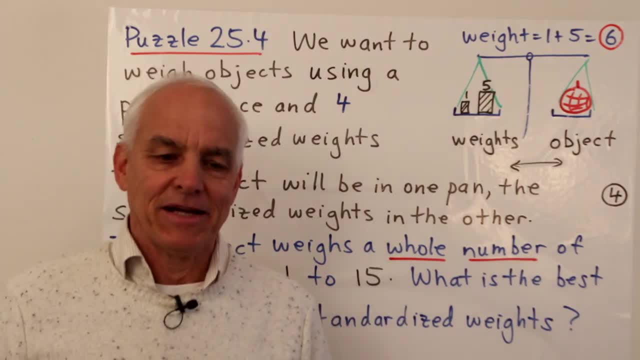 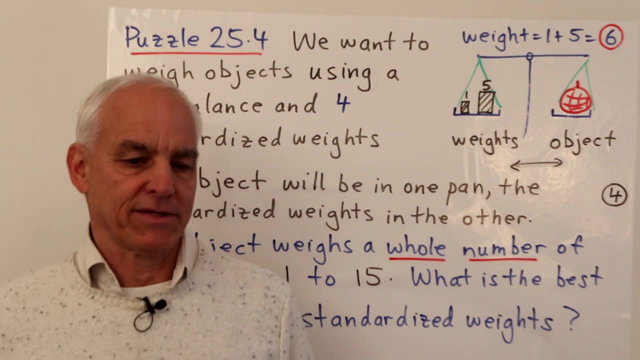 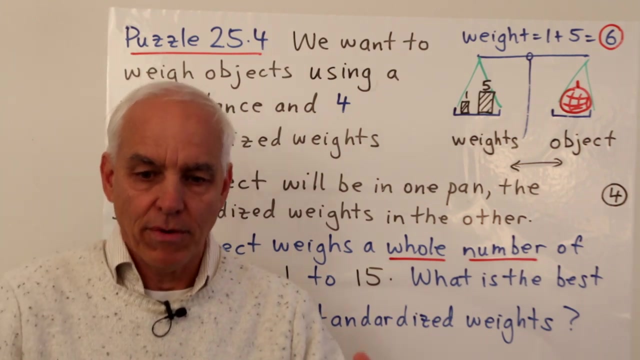 Actually to a situation that we've already discussed in the arithmetical context in our previous video, But we don't have to say that to our children, who are wrestling with this. So this is an important and interesting puzzle, which is a kind of a to-do. 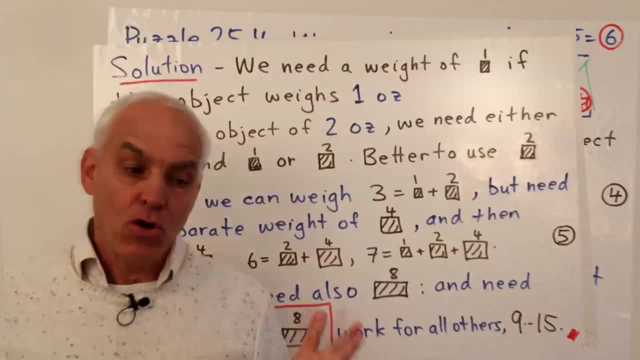 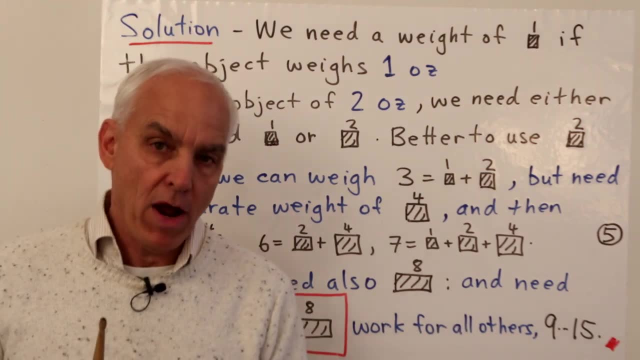 We are trying to figure out how to make this work. So what we're going to do is we're going to go through the possible weights of objects that we're going to potentially weigh from 1 to 15. And we're going to adjust our idea of the standardized weights. 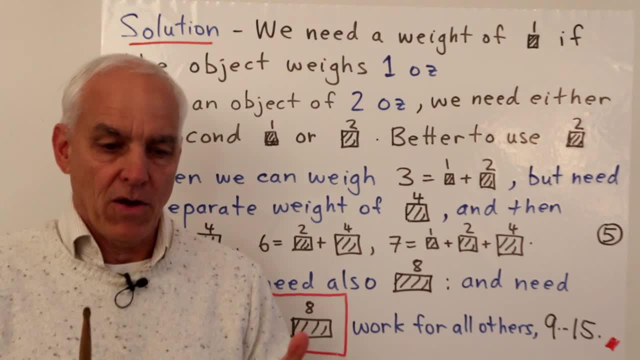 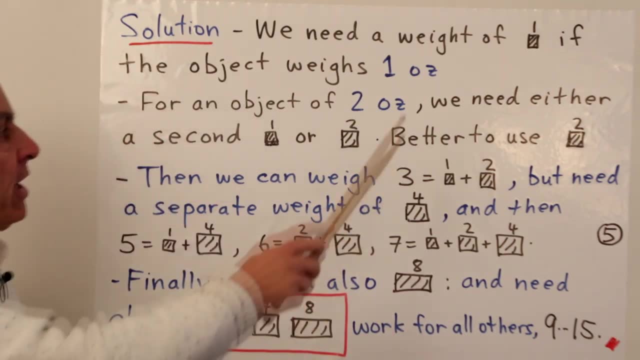 so that at each stage we'll be able to weigh all the objects up to that particular stage that we're at. So let's start with the simplest possible object. If we have something weighing one ounce and we want to weigh that using a pan balance, 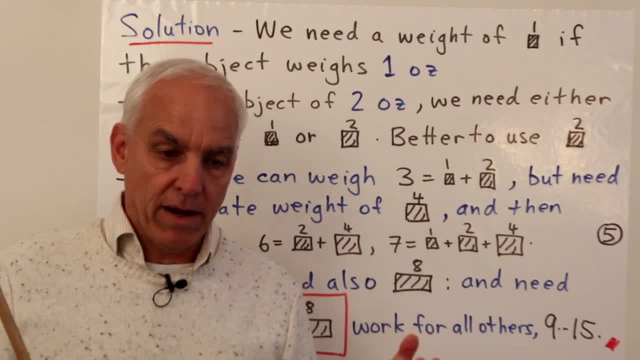 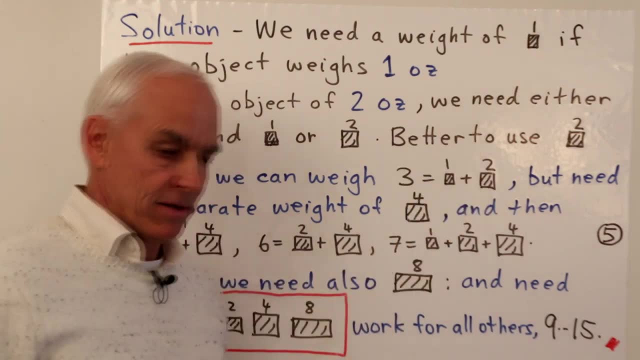 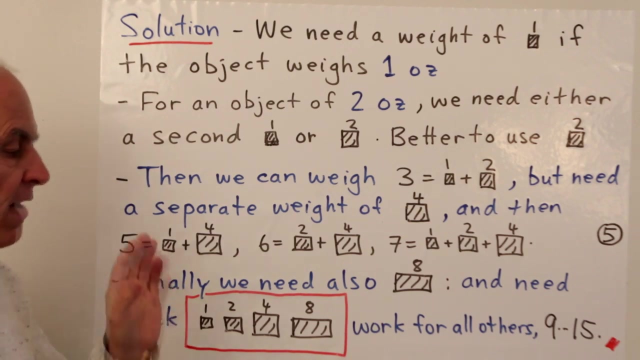 in the way that we've described. there's really only one way of doing that. So we need a weight of one ounce, And we'll illustrate that with this little black box that represents our standardized weight of weight: one ounce. So we have one of those. 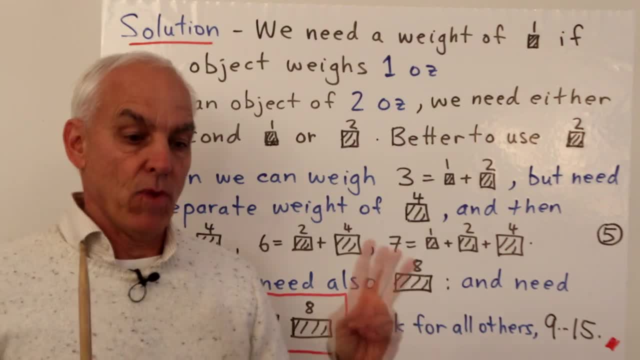 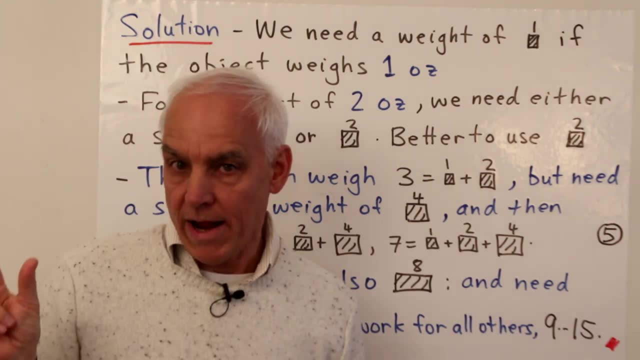 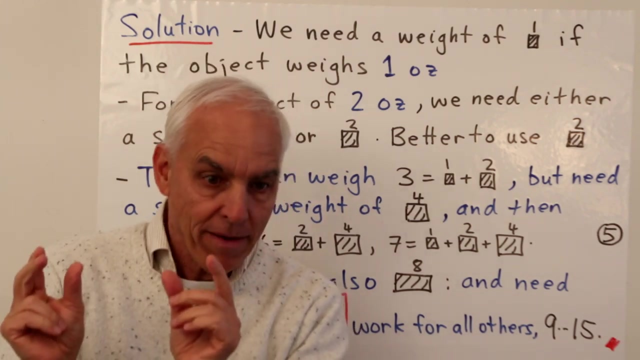 And now, what about an object weighing two ounces? We want to weigh that also Now. at this stage, we have two choices. We already have a one, One ounce standardized weight. What we could do is create a second one, So now we have two of them. 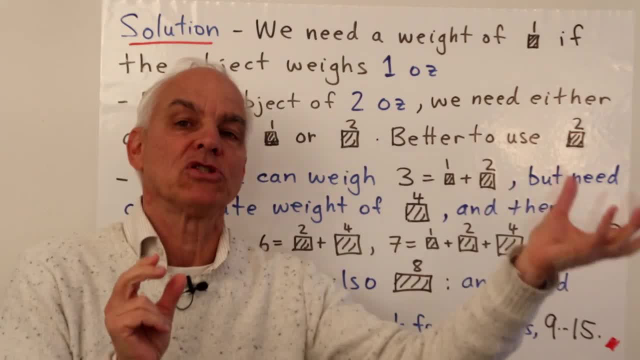 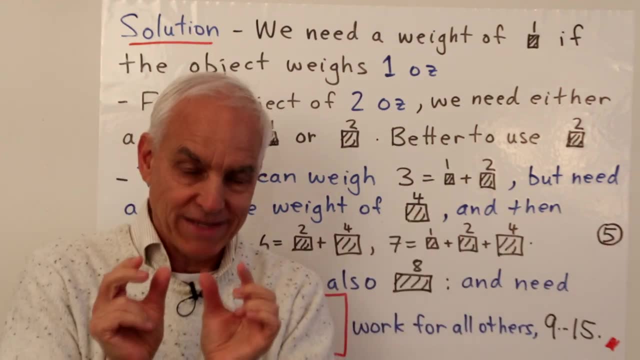 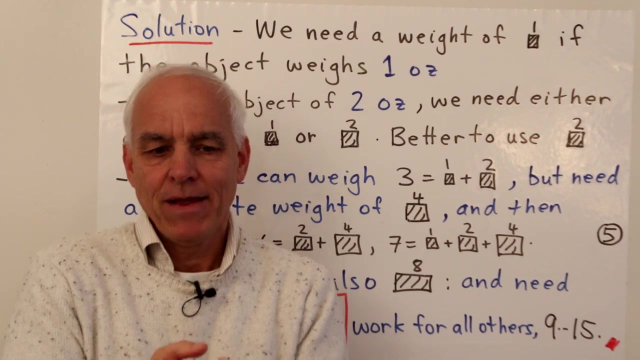 And with those two we could weigh our two ounce object. We could determine that this is two ounces by putting two standardized one ounce weights in the pan. But that would not be the most efficient way of proceeding because there's some duplication there and it's more efficient for us to introduce. 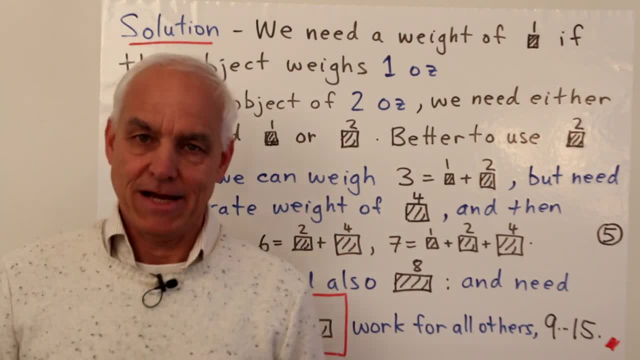 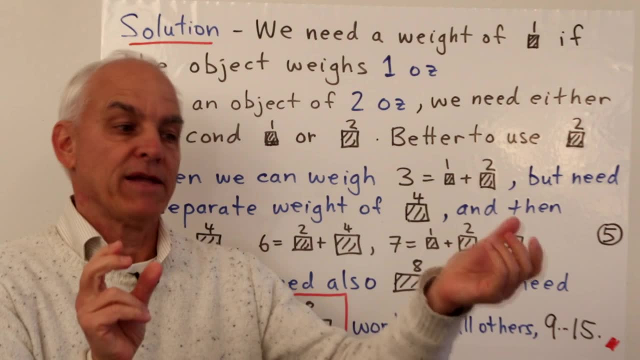 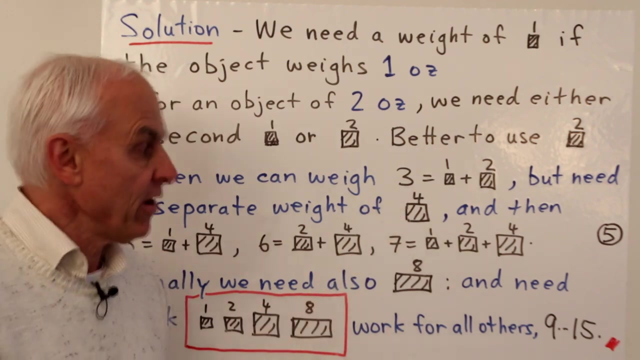 a two ounce weight instead. We already have a one ounce weight. Let's now introduce a two ounce weight, And we'll use that to weigh something that weighs two ounces. Well then, we're also able to weigh something weighing three ounces, because three is one plus two. 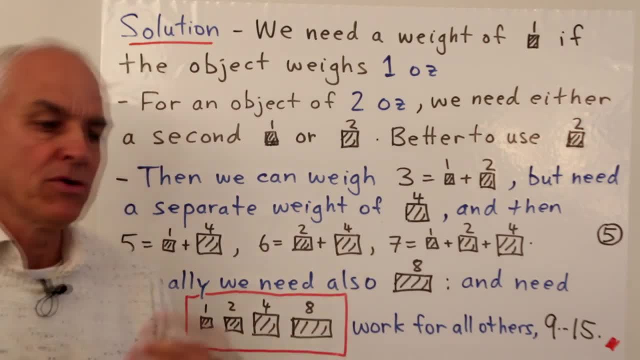 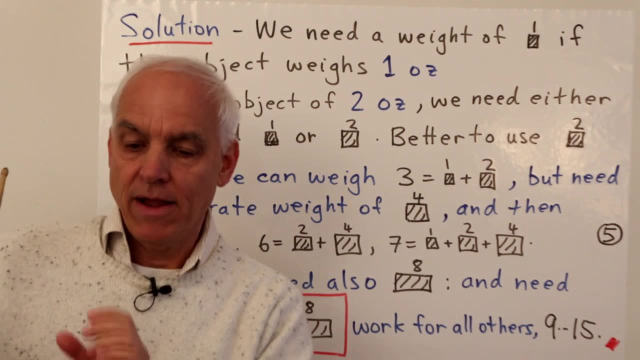 But after that we're going to require a new standardized weight of four, because there's no way for us to weigh something which is two. We're only going to be weighing four ounces if we just have a one and a two ounce standardized weights. 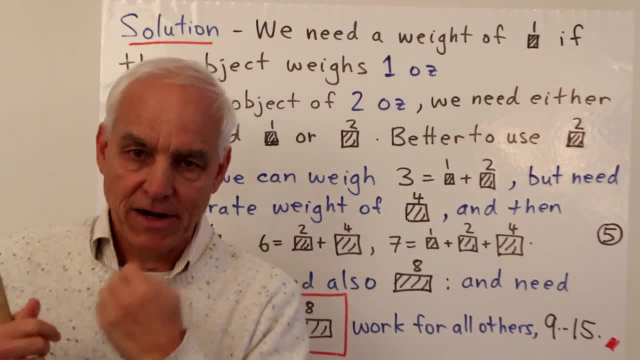 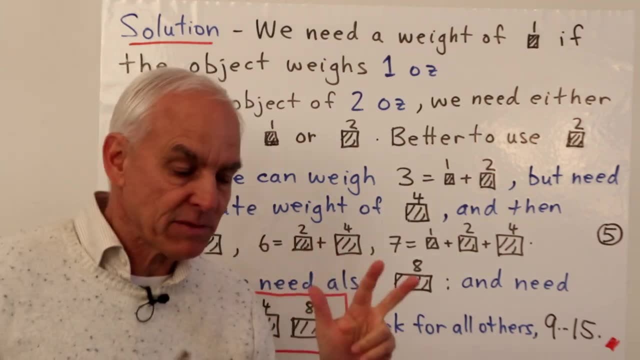 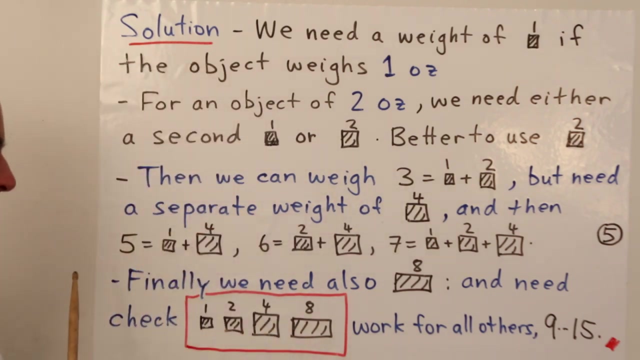 Okay, so we have to introduce a four ounce standardized weight And then, with the one, the two and the four that we have up to this point, we are then able to weigh something weighing five ounces, because that'll be one plus four. 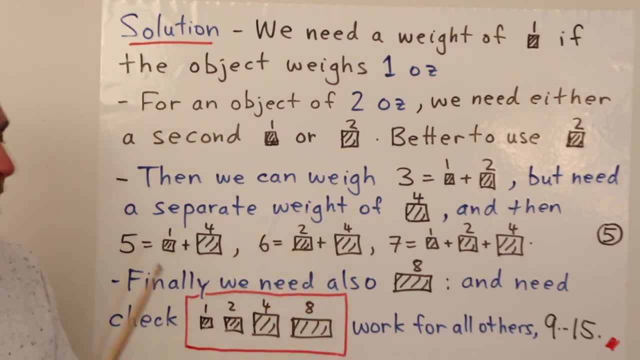 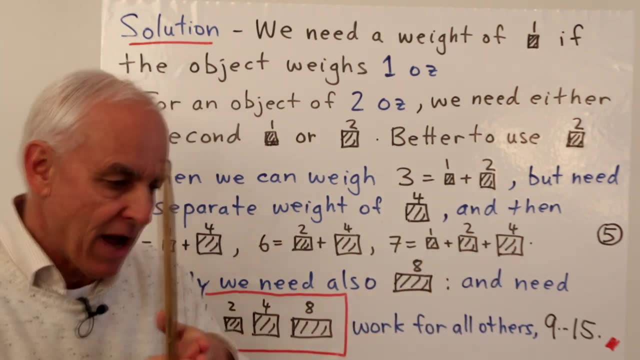 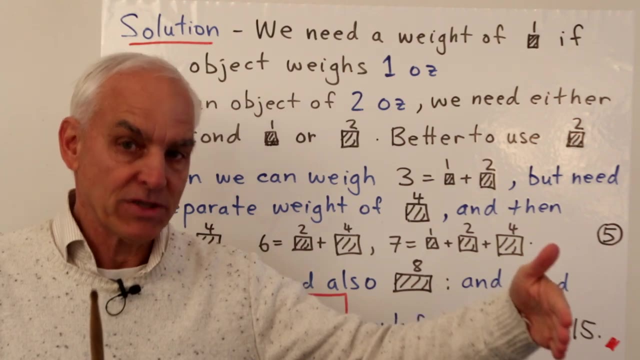 Six ounces, because that'll be two plus four, And seven ounces, because that will be one plus two plus four, So it will be good up to and including seven, But eight we will need a new standardized weight for. So, finally, we need also a standardized weight. 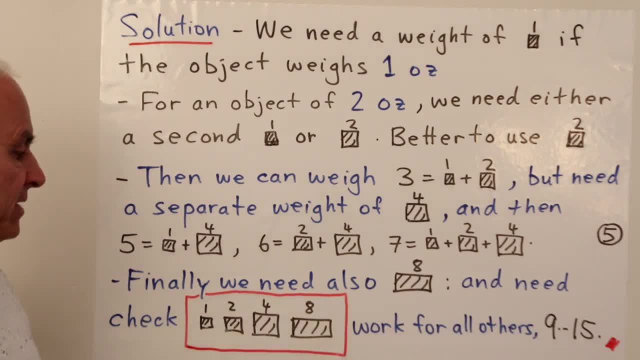 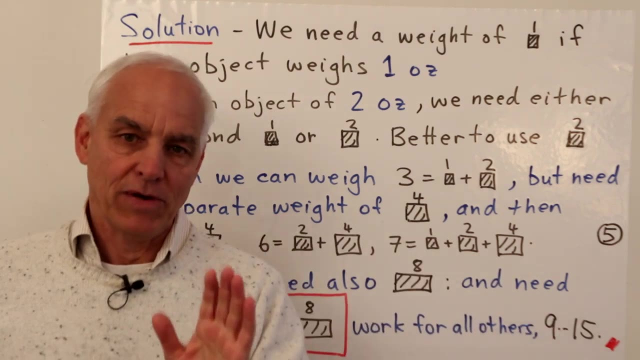 of weight eight ounces. And then we need to check that with these four standardized weights- one, two, four and eight- we're then able to weigh all the remaining weight from 9 through 15. so let me do that verbally, although we can also write it. 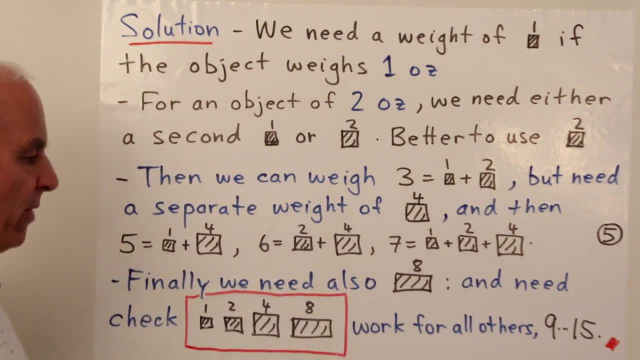 down on a piece of paper. how do we weigh something weighing 9 ounces? well, we use the 1 and the 8. they combine to give us 9 and 10 ounces. we use 2 and 8: they combine to give us 10, 11 ounces. that would be 1 plus 2 plus 8, 12 ounces would. 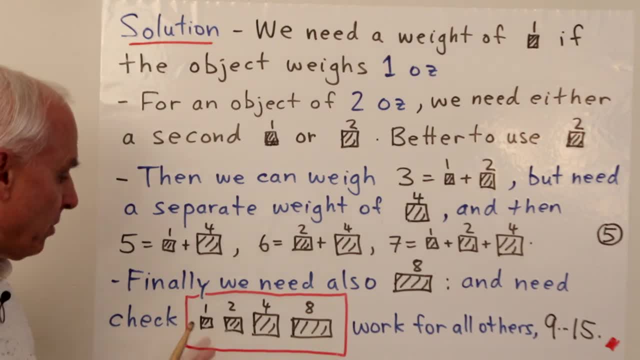 be 4 plus 8. 13 ounces would be 1 plus 4 plus 8, 14 ounces would be 2 plus 4 plus 8, and 15 ounces would be all four of them: 1 plus 2 plus 4 plus 8. 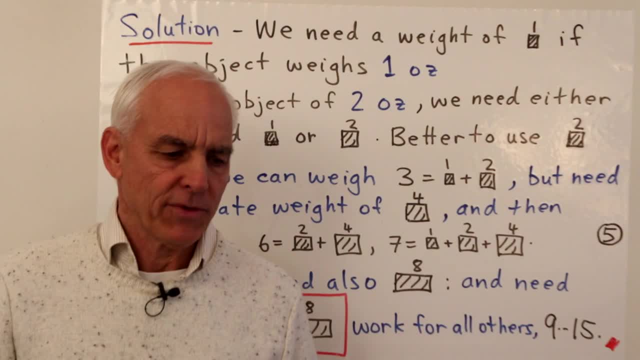 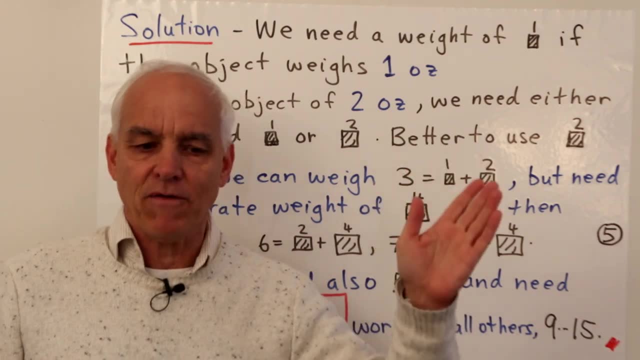 arithmetically. hopefully the student will say: wait a minute, we've. we've done the same kind of thing back in the previous week when we were talking about that puzzle involving row rectangles and expressing row rectangles in terms of ones, twos, fours and eights. 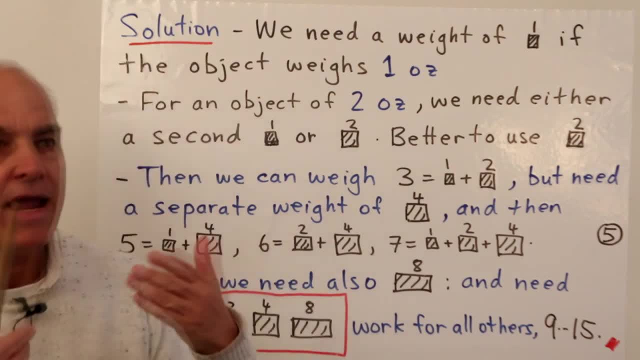 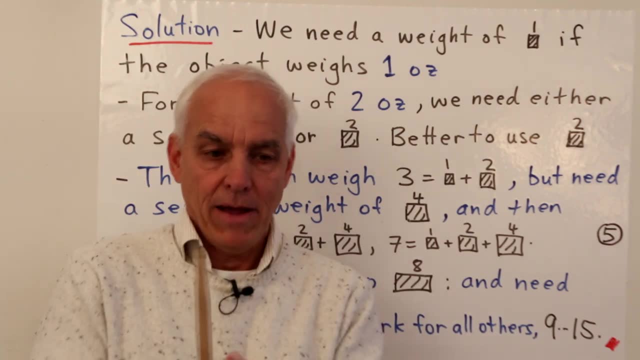 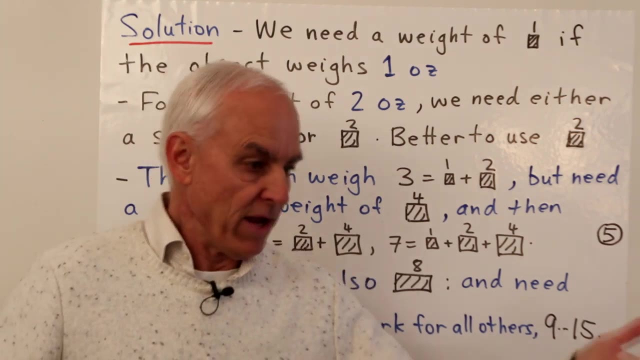 it's really arithmetically the same, but now we're thinking about it in a different way. now we're thinking in terms of actually having physical standardized weights, and that's a kind of application of this arithmetic which is going to be useful, because if we have to weigh things with a pan balance, then exactly this technology is. 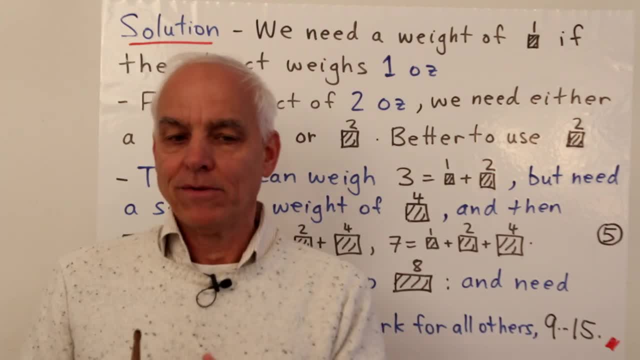 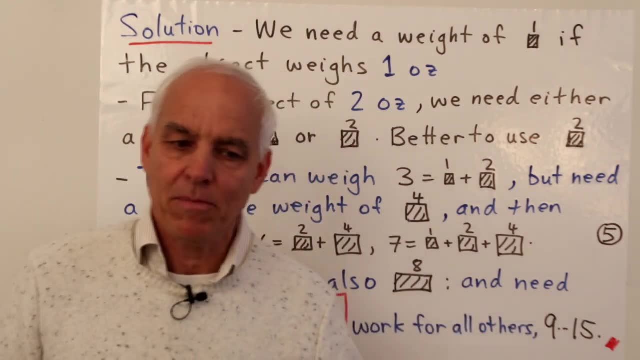 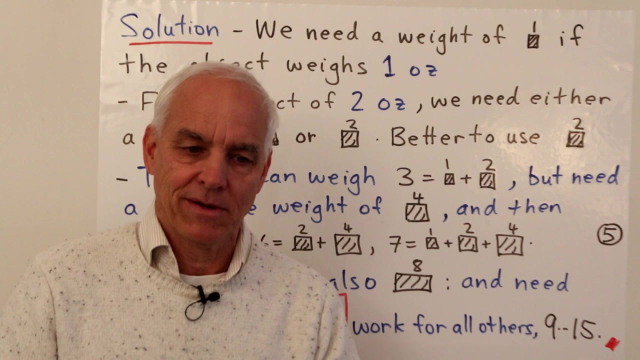 going to be useful for us and hopefully, for the more advanced students, more experienced ones. after we've gone this far, they'll be wanting to say: and what happens if we go further? what would be the next weight that we would need to introduce? well, obviously, it's going to be the weight of 16. and then how many? 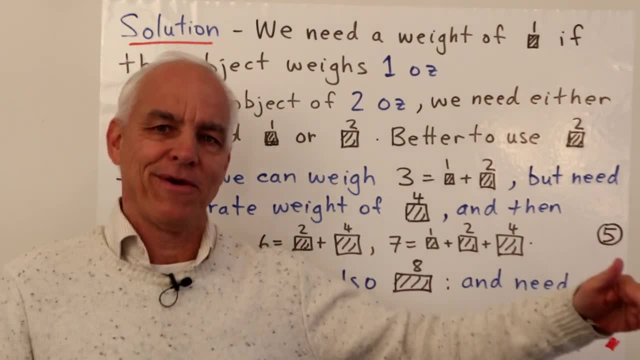 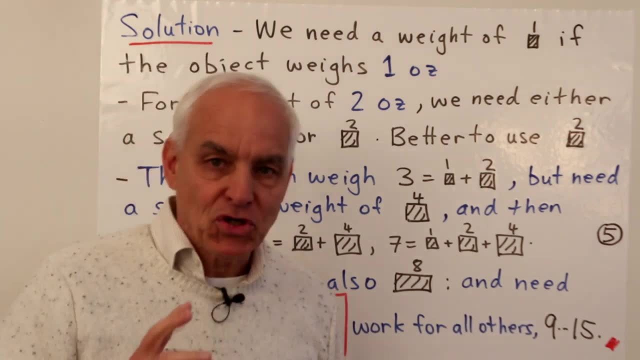 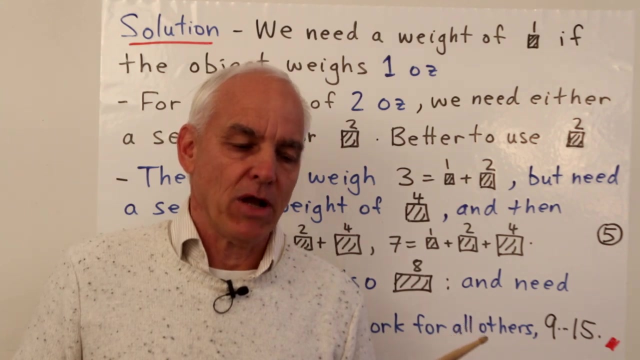 pounds would it be, and how far will that allow us to go, And what will be the next one, et cetera. So the importance of the powers of two and sort of binary representations of things, although we don't have to use that terminology. 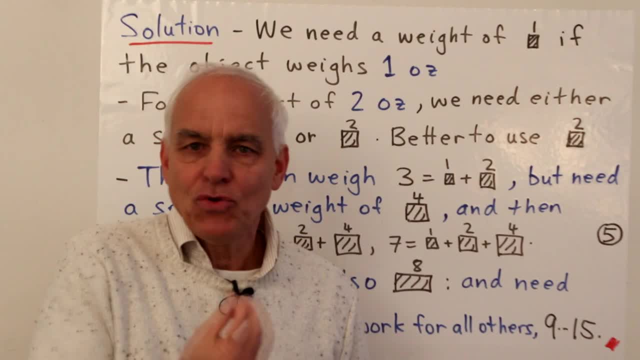 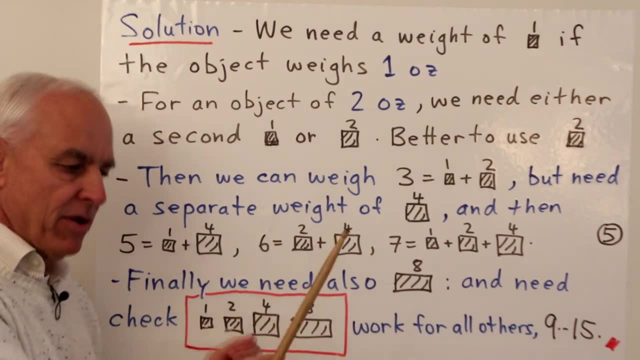 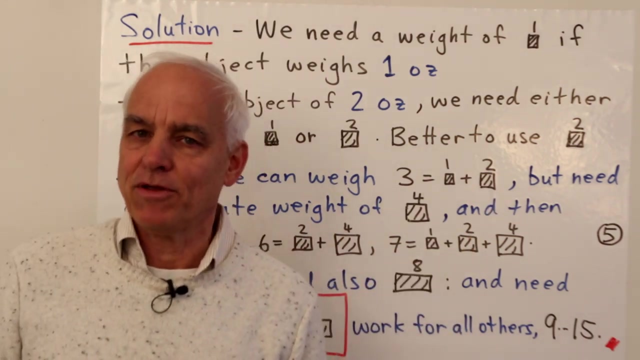 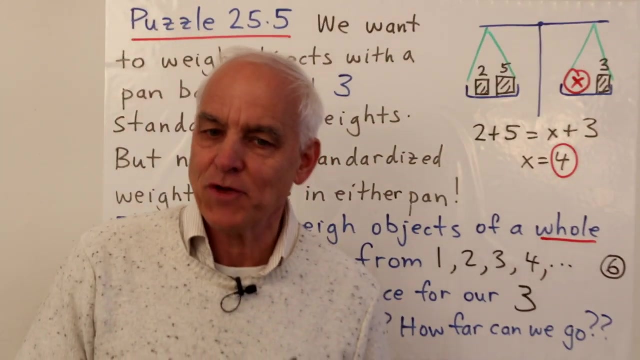 it's already becoming intuitively clear to the students because they're making these computations summing up using powers of two. So it's a very important kind of direction of familiarity with arithmetic. So this is a very good puzzle. Now our final puzzle is a variant on the previous one. 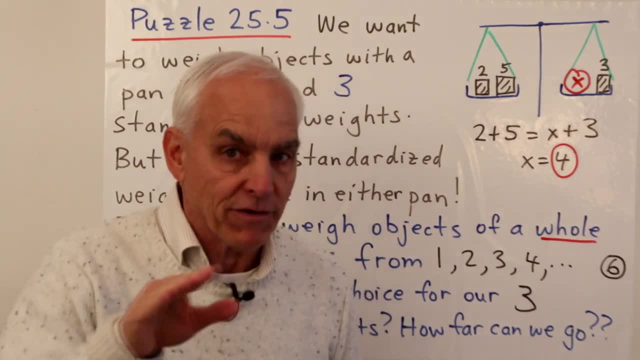 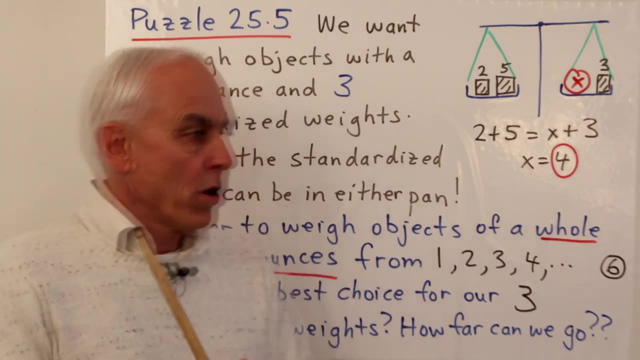 and quite an interesting one that I think will be more novel to many of you viewers also, So there'll be something for you to learn here as well. We're gonna be looking at the same kind of situation. We're still trying to weigh objects using a pan balance. 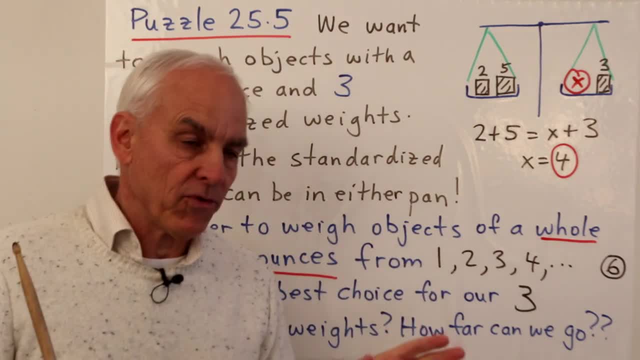 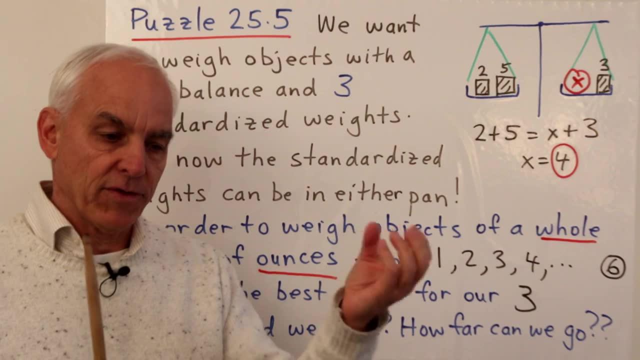 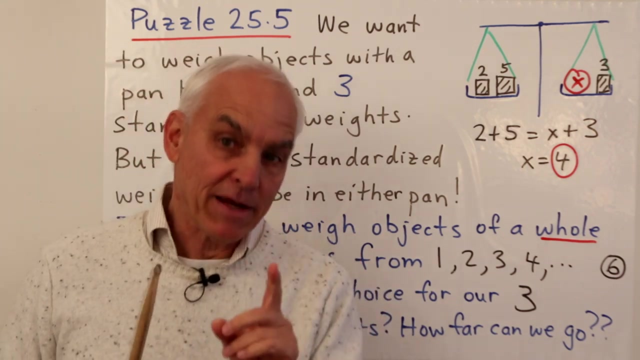 We're still in the, the imperial US system with ounces, And we're still restricting ourselves to whole number of ounces- the objects that we're weighing- But what we're gonna be doing now is allowing ourselves a little bit more flexibility about how we use the standardized weights. 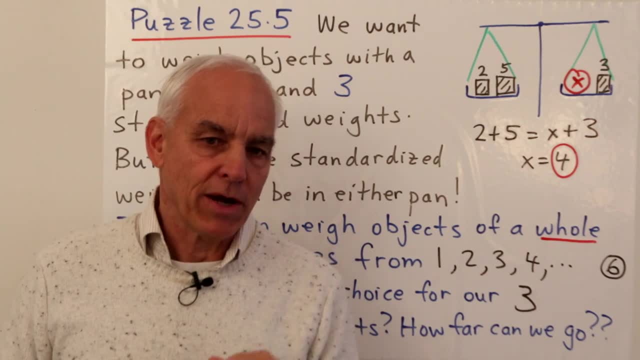 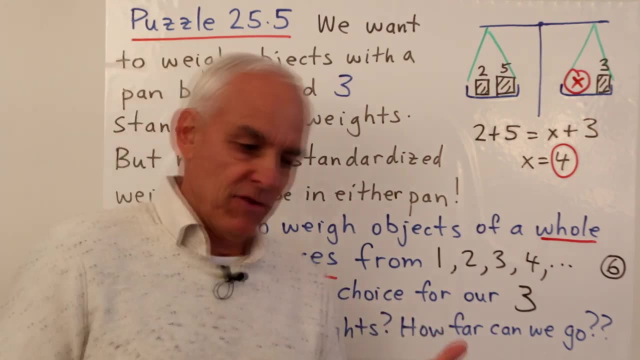 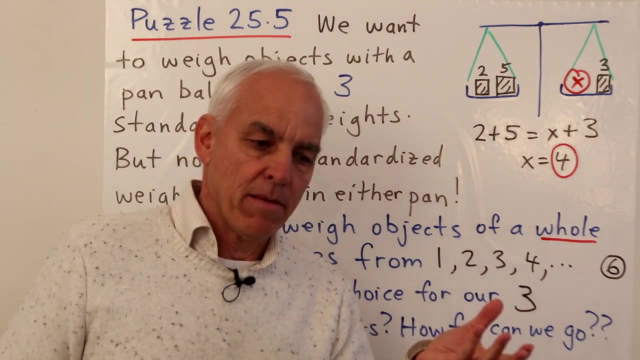 In fact, maybe this is even something that could occur to a young student. If you're playing around here, they might have this idea. Why do we need, actually, since we have these two pans in the pan balance, why do we need to insist that the object is in one pan? 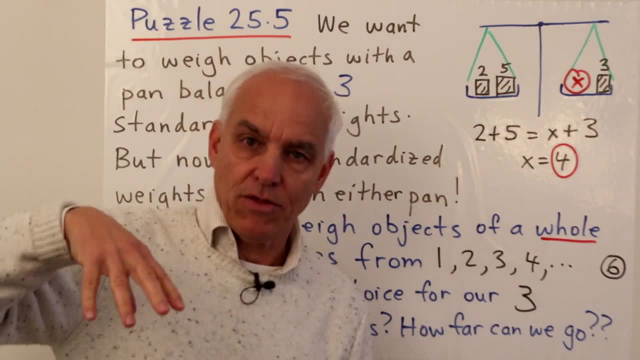 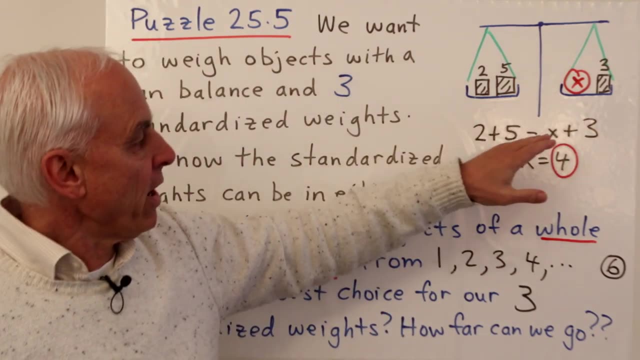 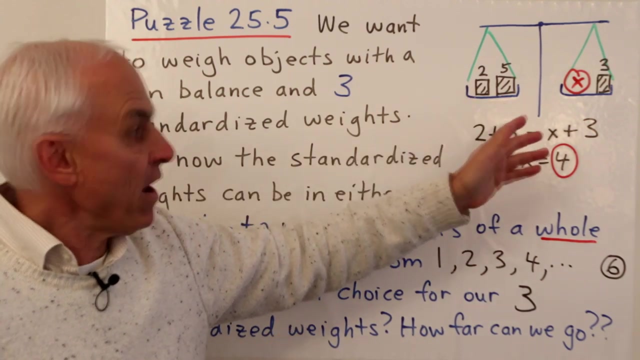 and all the standardized weights that we're gonna be using are in the other one. Couldn't we maybe combine them? Couldn't we have a situation like this where there's the object in red labeled with X, and over here we have standardized weights of, say, two and 5.. 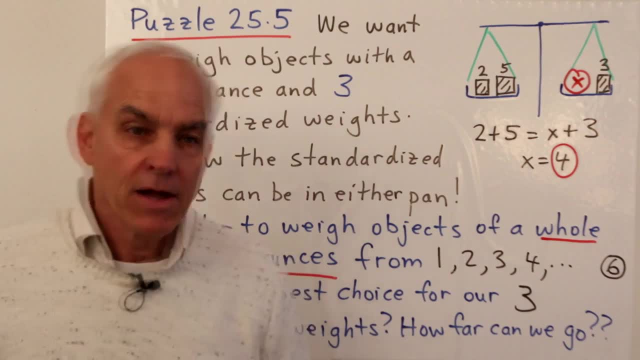 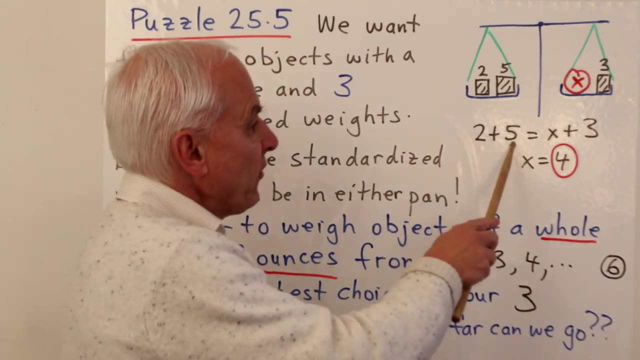 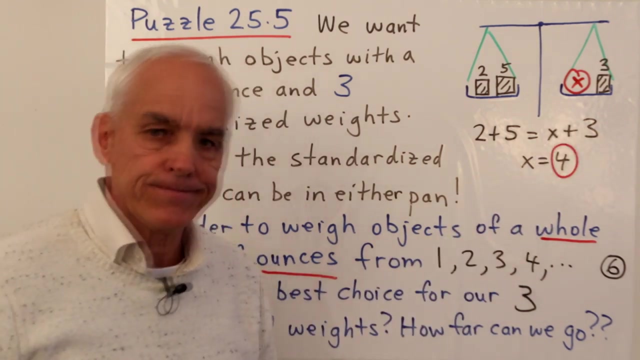 over here there's a standardized weight of 3.. Now, suppose those two total weights balance, What could we deduce? Well, 2 plus 5, the left-hand side here would have to equal x, whatever that is plus 3.. Alright, so what must x be for this? Well, 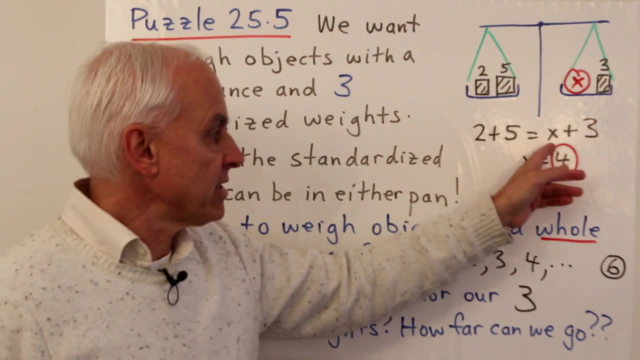 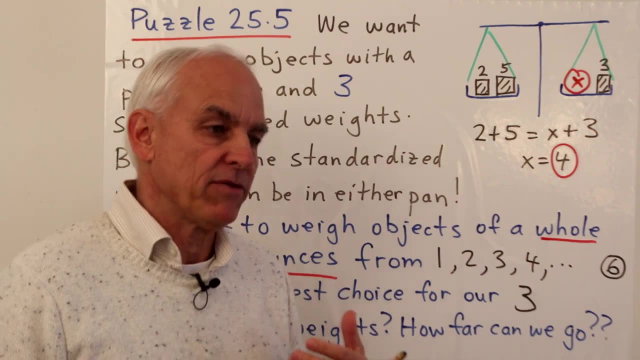 2 plus 5 is 7.. So x plus 3 is 7.. So what do we have to add to 3 to get 7?? Well, we have to add 4.. So we could deduce from this that x has to be 4.. So 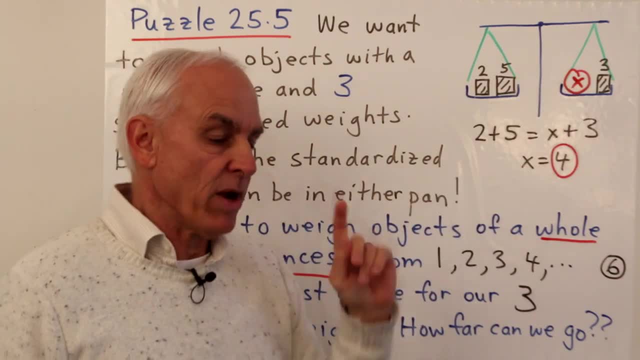 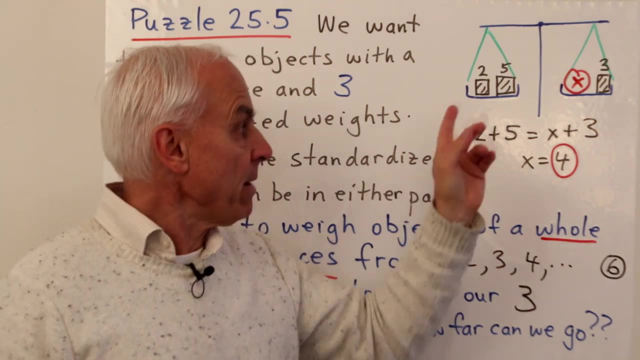 in this situation, we're able to deduce that this object has weight 4, even though we don't have a 4 standardized weight and even though we're not able, with these three standardized weights, to get a total of 4 on one side, But by 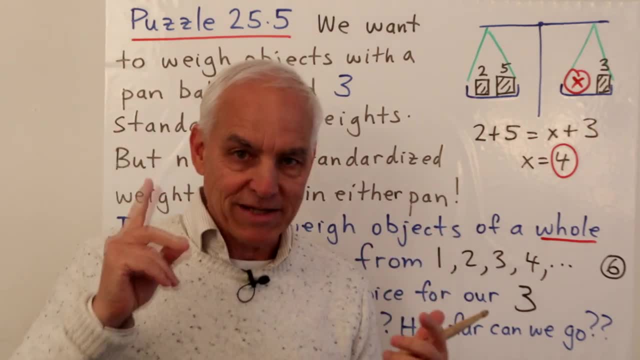 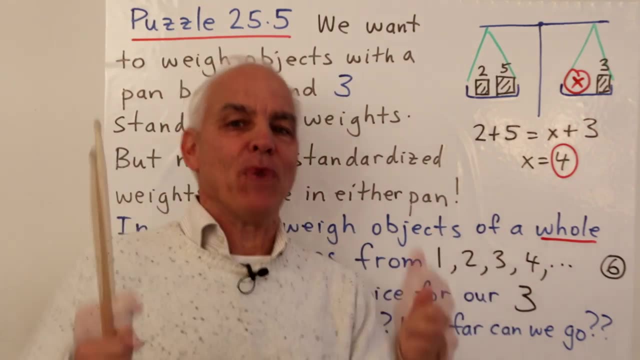 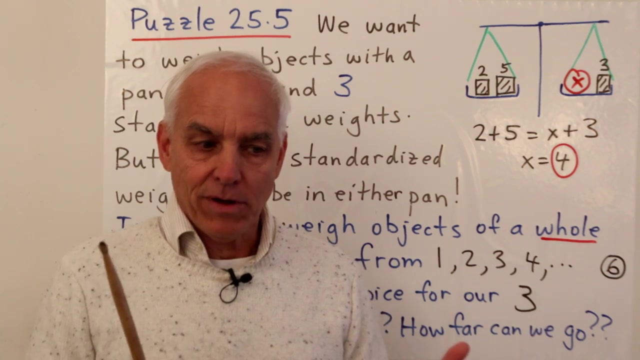 combining them, on both sides, we are able to weigh something. So that's the basic idea. We're looking for an improved technology, an improved way of using standardized weights and a pan balance to weigh stuff. Hopefully, that will allow us more efficiency. We'll be able to save costs. In fact, that's exactly what happens. 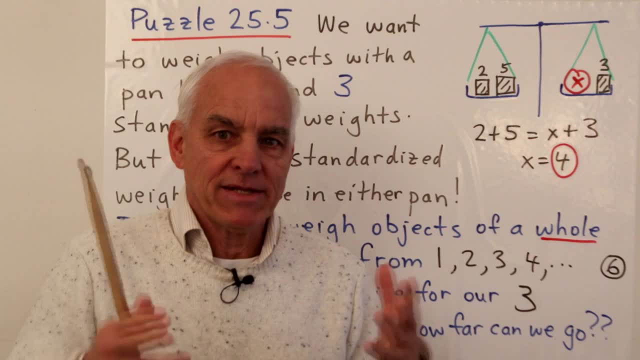 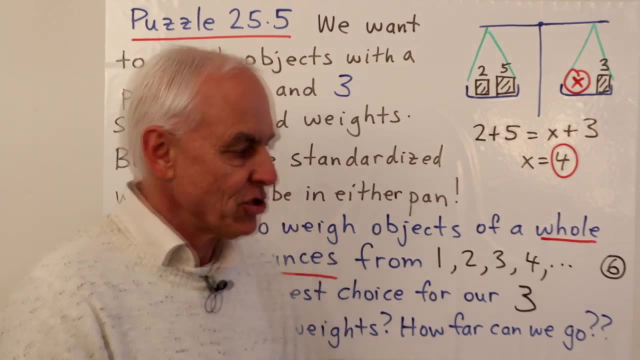 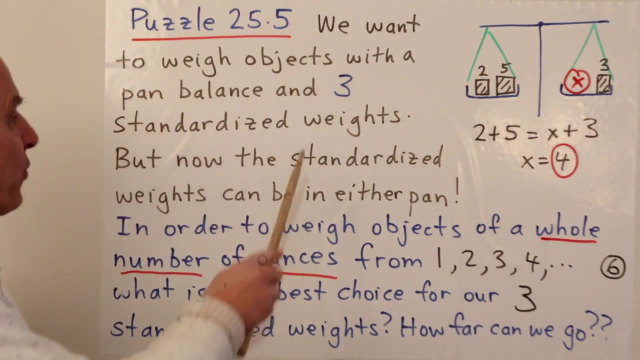 here. So the common sense, practical application of this should be quite obvious, even to young people, Children. Okay, so here is the puzzle. officially, We want to weigh objects with a pan balance and this time 3 standardized weights. to make it just a little bit simpler, We have 3 standardized 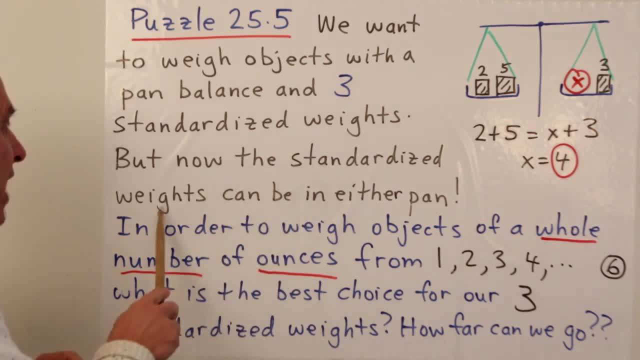 weights. But we're going to agree that now the standardized weights can be in either pan, just like here, And in order to weigh objects still of a whole number of ounces. and I'm not going to go from one up to a certain amount, I'm just going to say 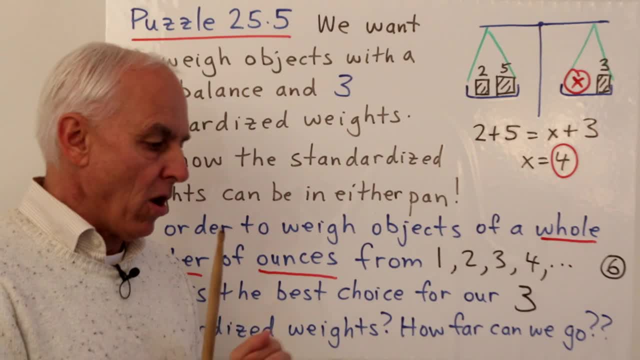 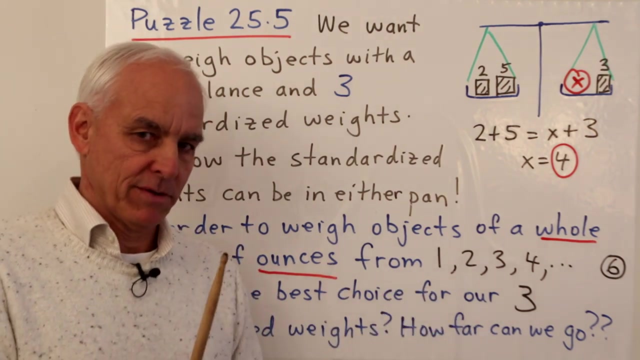 let's try to ensure that we can weigh all the objects with a whole number of ounces, starting from one, including two, including three, including four, up to however far we can go, But we don't want to miss any one of those, So we want to have a way of doing. 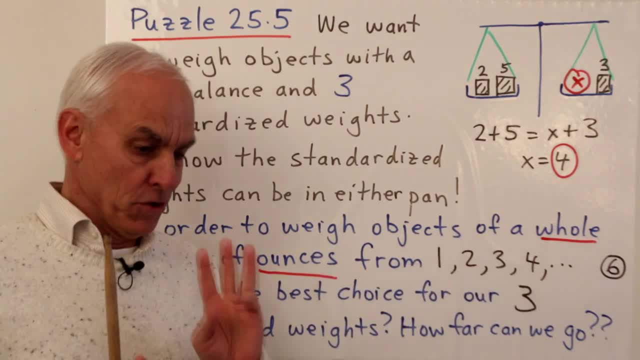 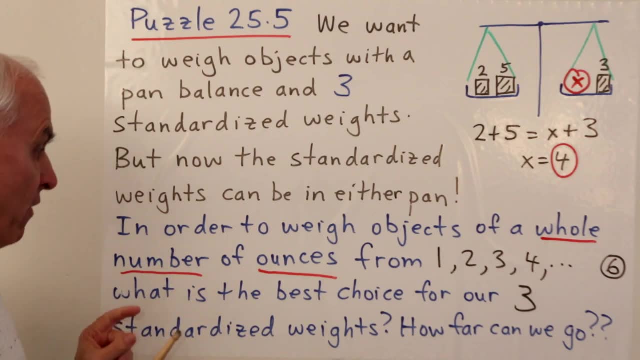 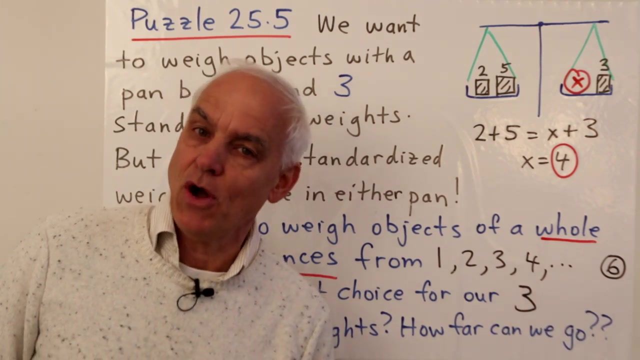 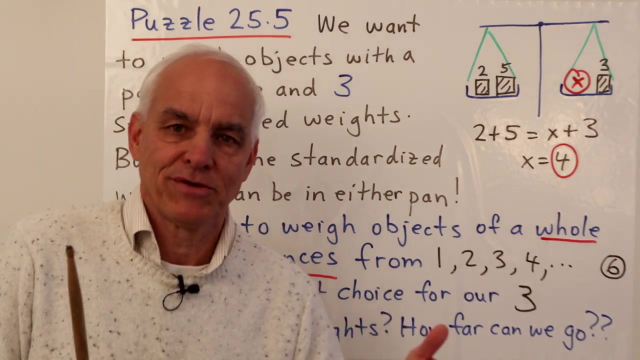 each one of those weights using only our 3 standardized weights that we have to choose, choose. So what is the best choice for our three standardized weights And how far in this sequence can we go successfully? We can weigh whole number of weights, up to how much? Now, this is a little bit of a tricky problem and it's 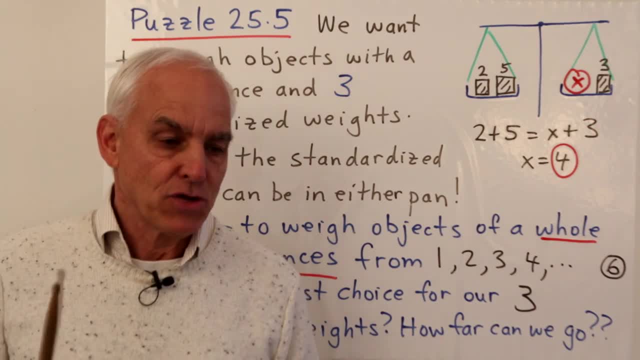 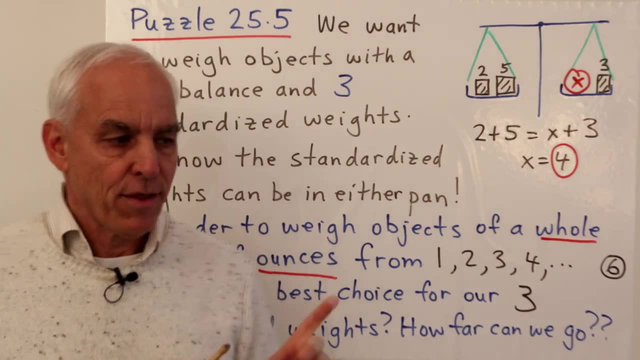 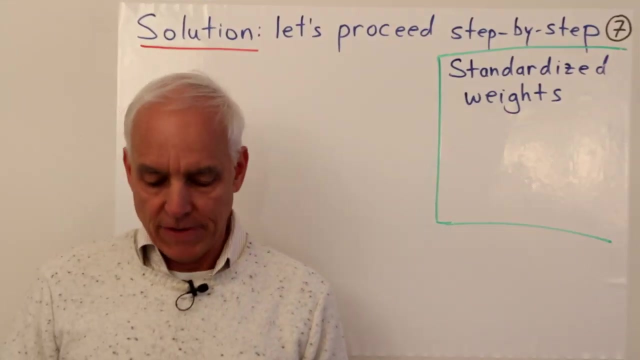 maybe a little bit unfamiliar. so I suggest that, educators and parents, you might want to pause the video now and spend a little bit of time yourselves thinking about how you're going to solve this problem. So let me sort of kind of go through way of thinking about this. We want to 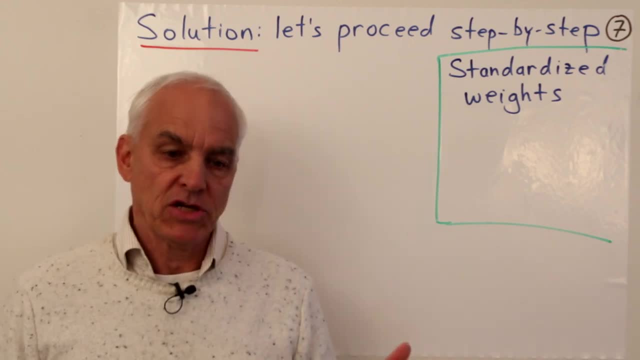 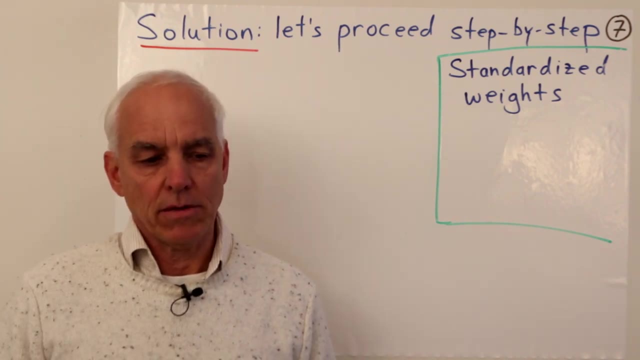 concentrate on the step-by-step procedure that we're going to be aiming for here, right? So we want to be systematic. we want to emphasize the importance of writing things down systematically. A student may not be really good at writing sentences and so on, but we can still write little equations. 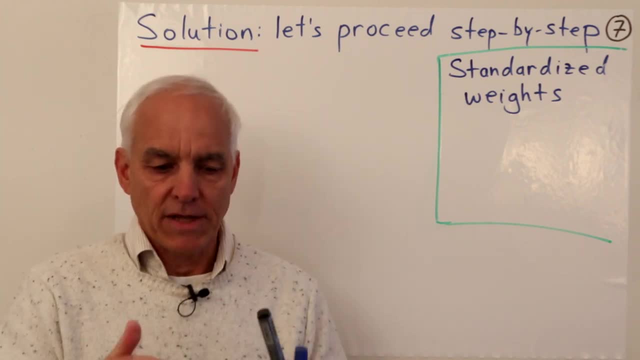 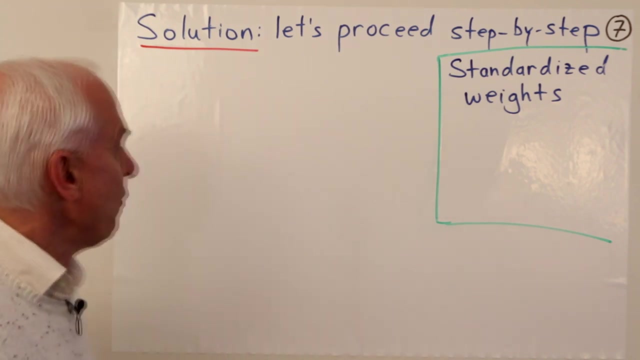 involving arithmetic, and we want to do that sequentially, one line at a time, in a way that the student can then can get a sense of the movement as we progress up through the possible weights. So let's start with a weight of one. I'll put it. 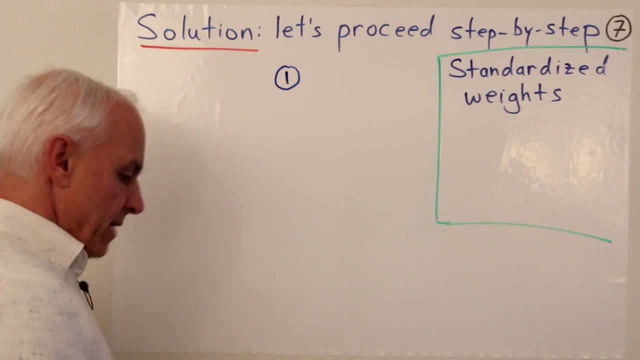 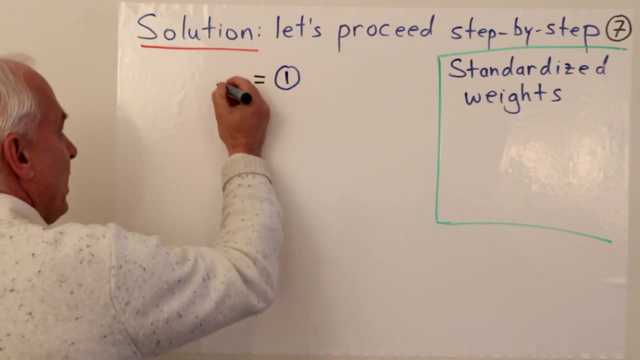 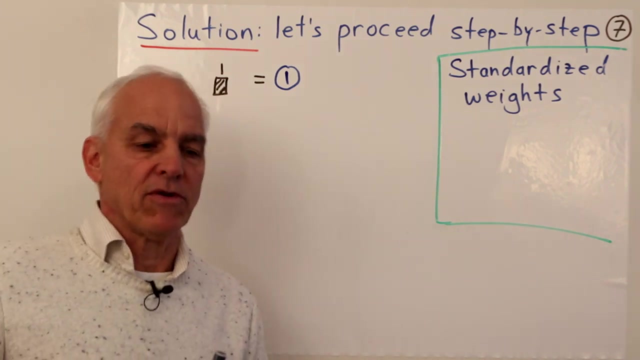 over here on the right hand side. That's a weight of one that we want to to balance, and in order to balance that well, we need a little standardized weight of weight one. So we are going to require, just as we did in the previous question, 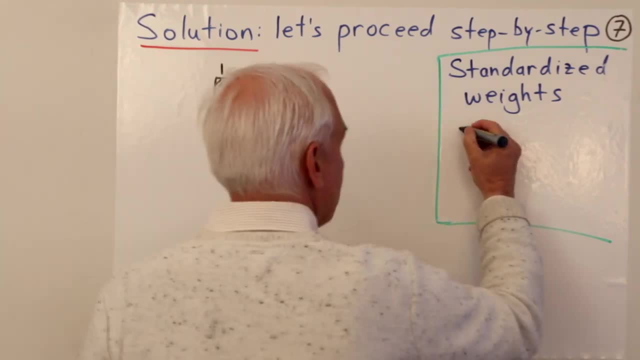 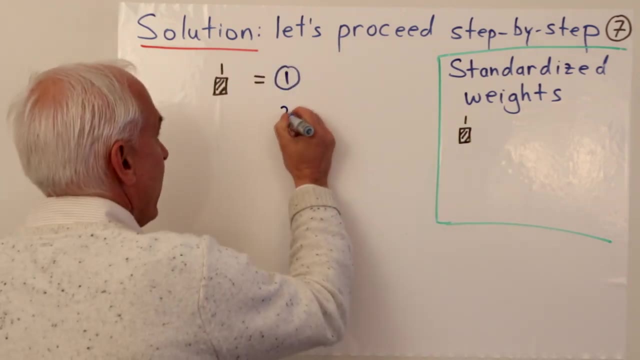 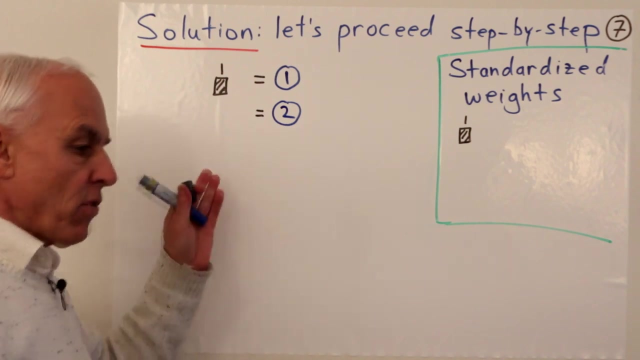 a standardized weight of weight one. Let's put that there. We're going to need that Now. we want to weigh something that weighs two ounces. How could we do that? Well, one way, of course, would be to introduce a two ounce standardized weight. 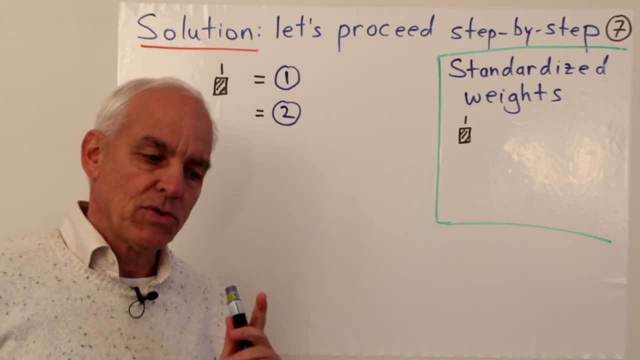 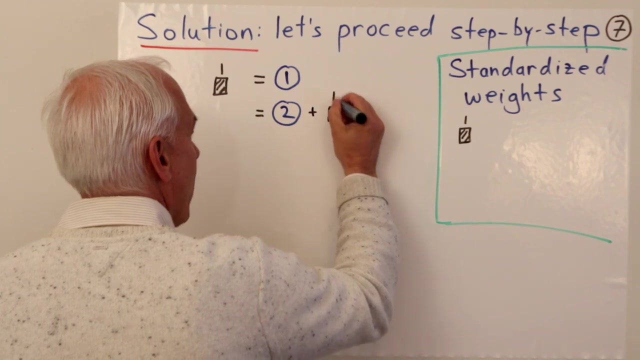 as we did in the previous case, But actually we can do something a little bit more clever by the the fact that we can use the one standardized weight that we already have And we can put that on this side one And then to to balance things. what we really want is another standardized weight. 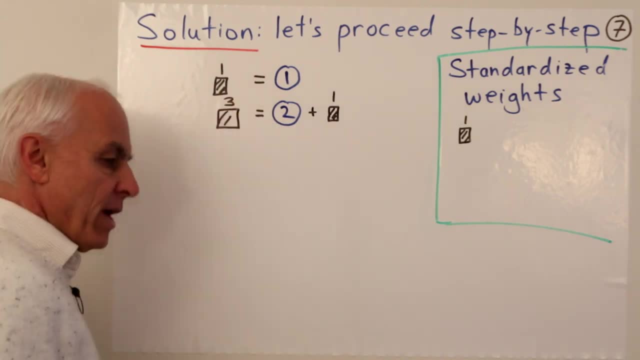 that will make it a little bit bigger- of weight three. So if we introduce a standardized weight of weight three, then exploiting the fact that we're able to use our standardized weights on either pan, then we can weigh an object weighing two ounces by creating this configuration: Two ounce. 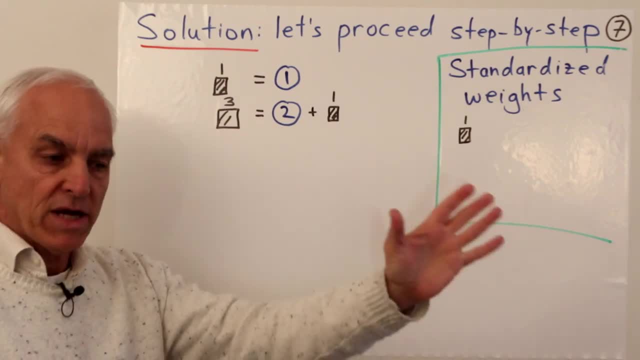 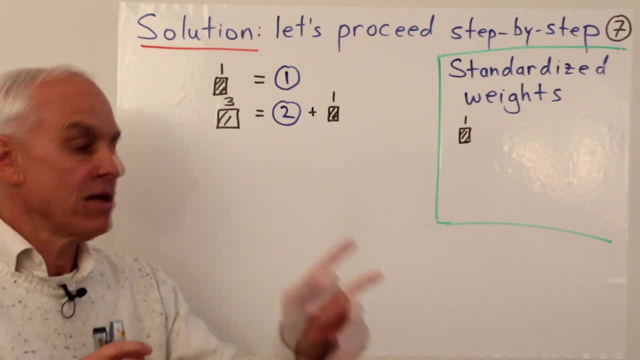 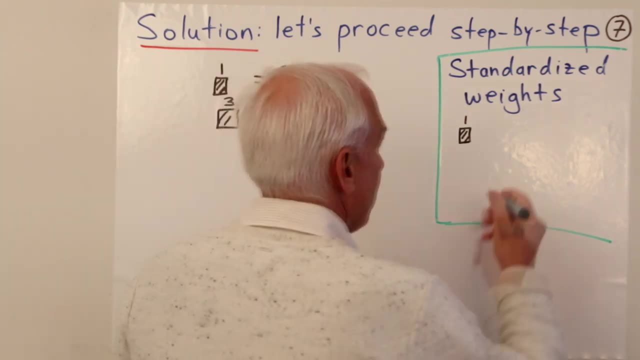 So that's what we're going to do. We'll put a three ounce standardized weight on the other. We have balance. We can deduce that that thing has to be two ounces, because one plus two equals three. Okay, so that's going to be our next standardized weight. 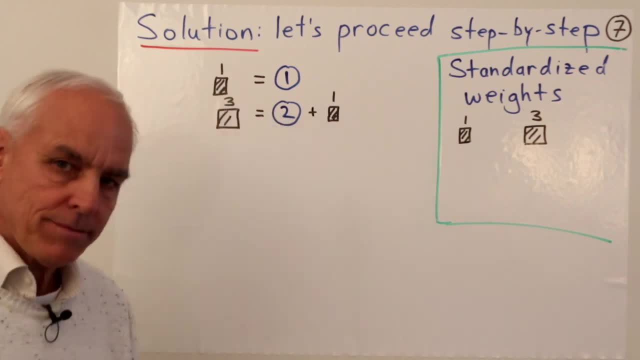 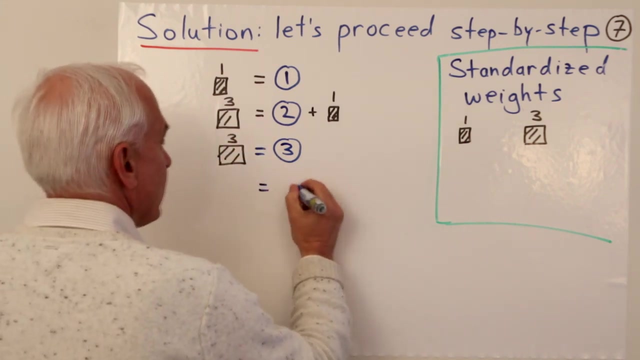 It's a three. Okay, so let's do some more weighing. How do we weigh something that weighs three ounces? Well, we're just going to use the standardized weight of three. That's easy. And how about something that weighs four? How are we going to weigh that? Well, we're going to use 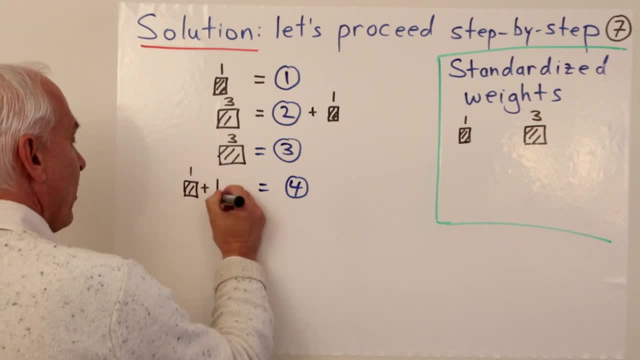 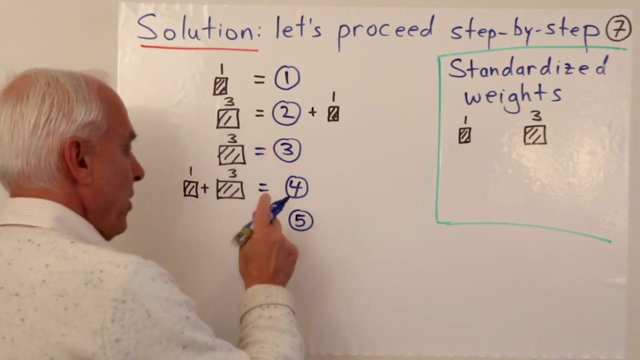 the one that we already have, plus the three that we now have, and that will balance with four. So four is good. How about five? Five, Can we weigh five just with the one and the three? No, We can't. We now need a new. 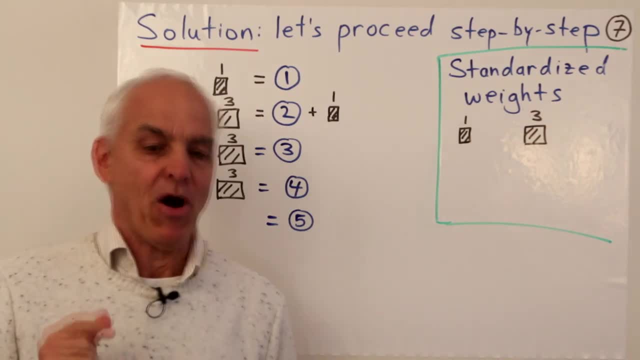 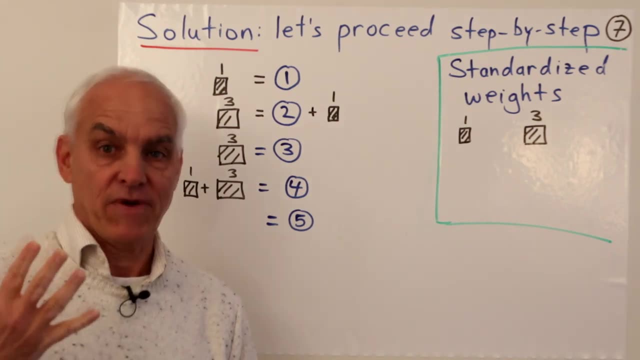 standardized weight. and now we have to scratch our heads and pause and think carefully for a minute. Which standardized weight are we now going to introduce? Of course we can introduce five, but that's not the most efficient thing to do, That's not the cleverest thing to do. You could also use six. 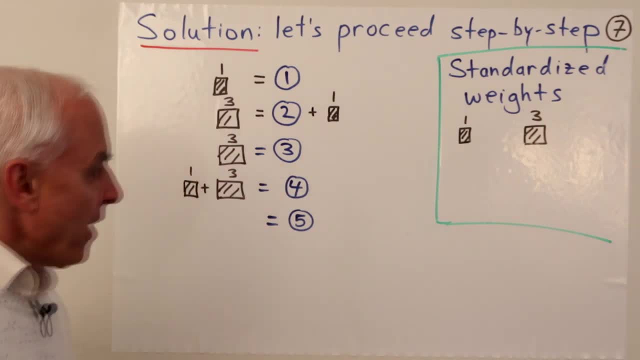 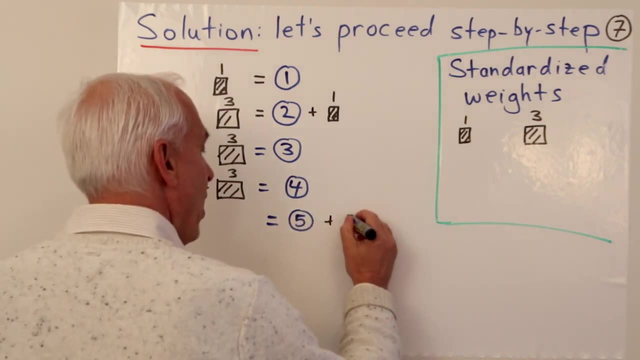 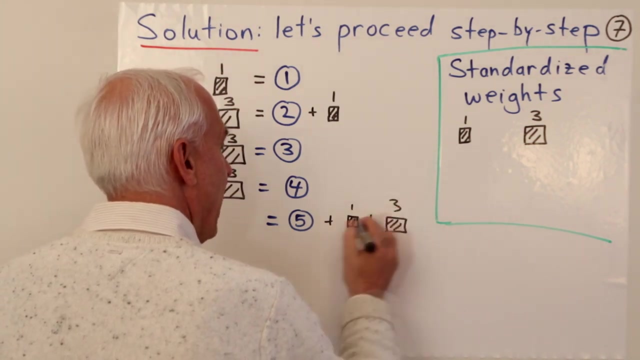 or seven, but neither of those is the cleverest thing to do. The clever thing to do is to realize that we can weigh five by putting the totals that we already have, the one and the three plus three, over in the same pan as the five. 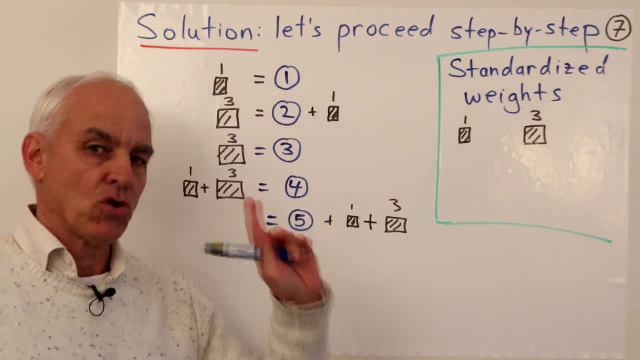 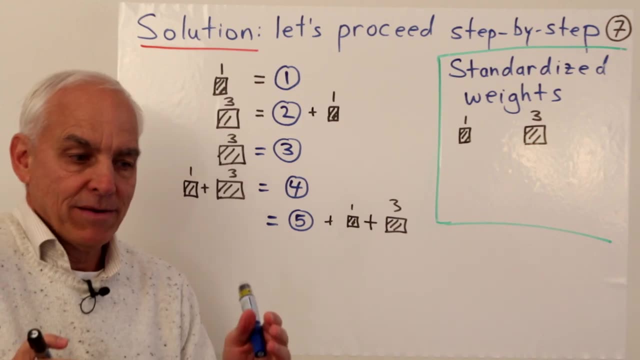 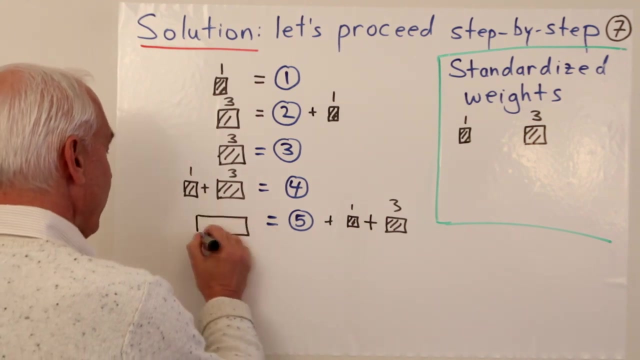 and then that would form a total of nine. And so if we're able to have a standardized weight of nine ounces, we can balance this situation and determine that that's five. So let me make a thicker one like this: So there is one of weight nine. 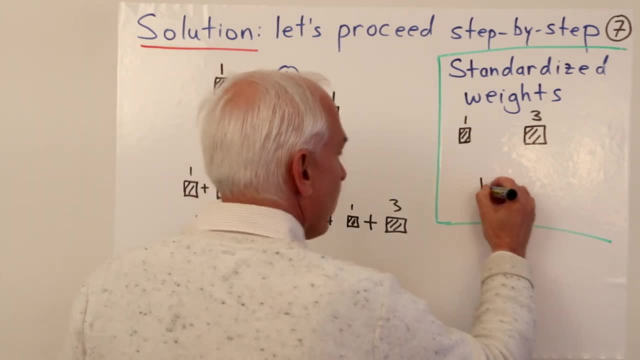 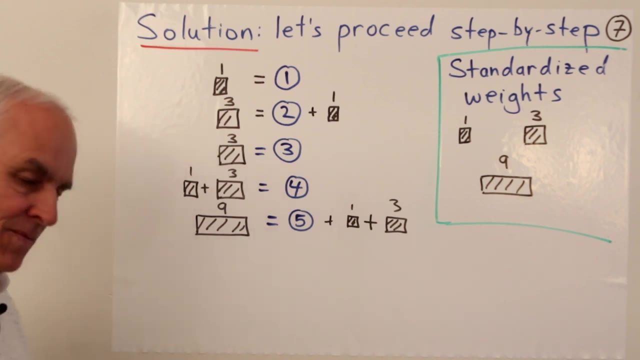 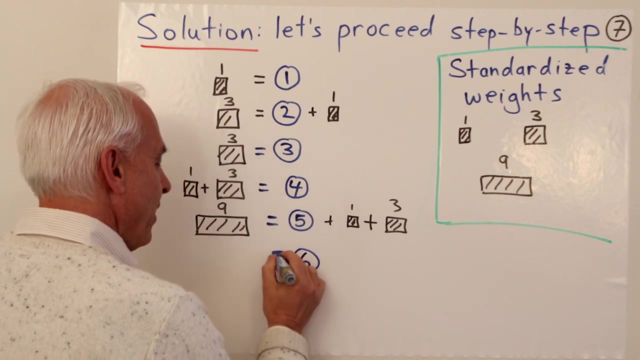 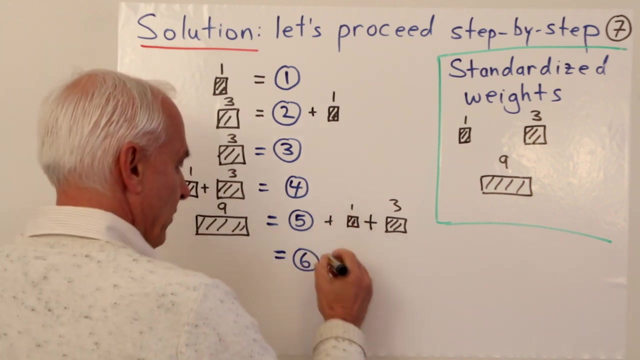 So there's our third weight: nine. Okay, what about six? How would we weigh that? Well, that's one more than the previous. so what we should do is kind of get rid of that one that's sitting there and just use the three. 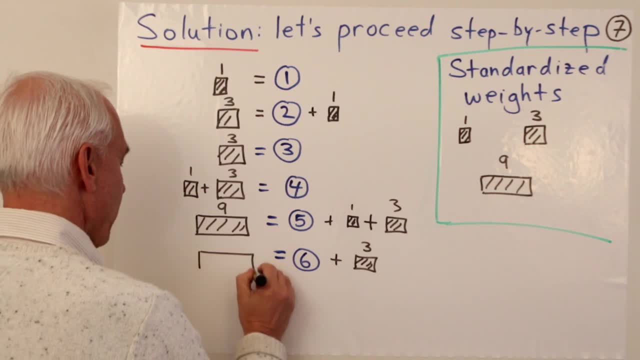 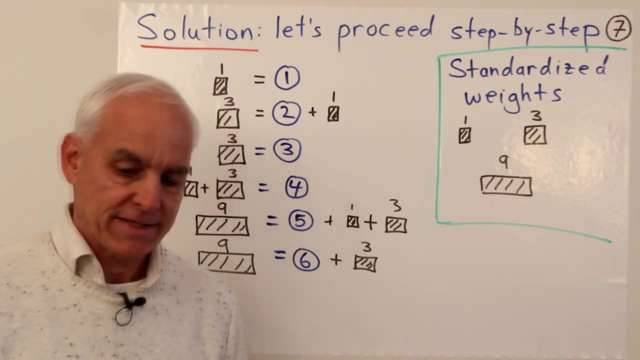 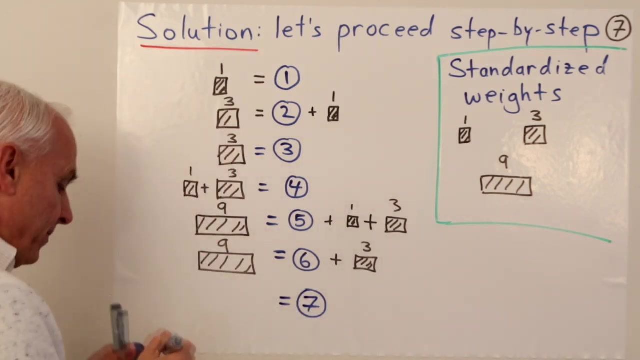 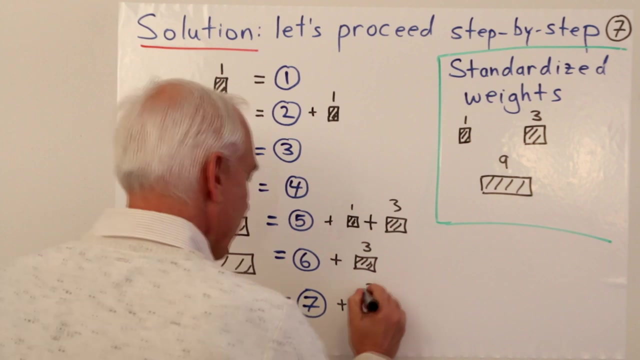 And then over here we still have a nine. So, yes, we're able to weigh something weighing six ounces. What about seven? Well, seven. we could also have a three on this side. That would give us a total of ten. 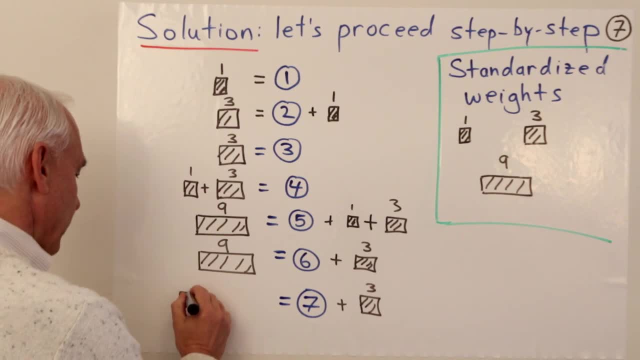 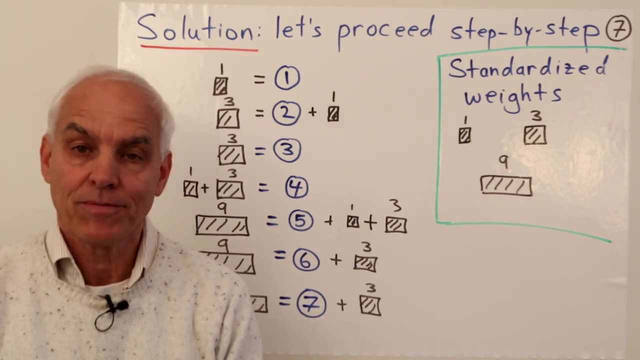 And can we cook up a ten with the other two? Well, yes, we can, because we can write that as one plus our nine, So we can also weigh something weighing seven ounces. And now we can actually proceed, and I'm going to let you figure out how to do. 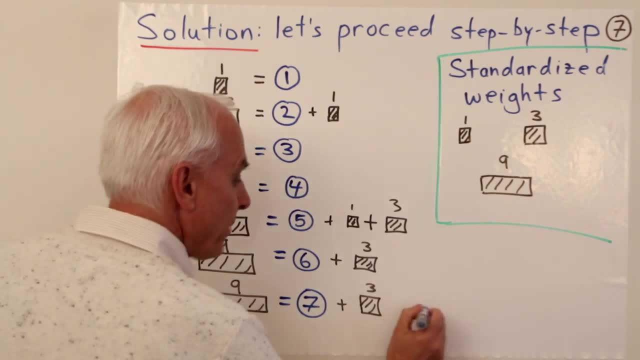 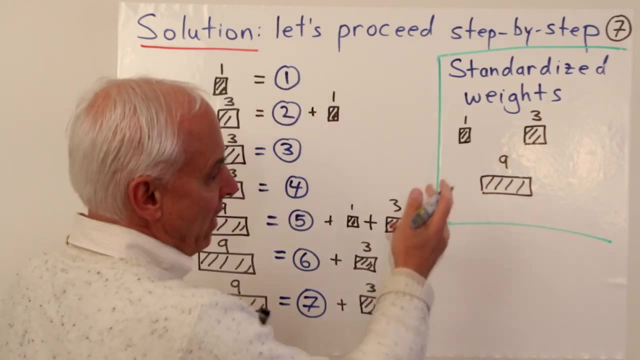 the remaining ones, And it turns out that we can keep going up to well kind of obvious what the largest one is going to be. right, The largest one is going to be when we use all of these three on the one side. 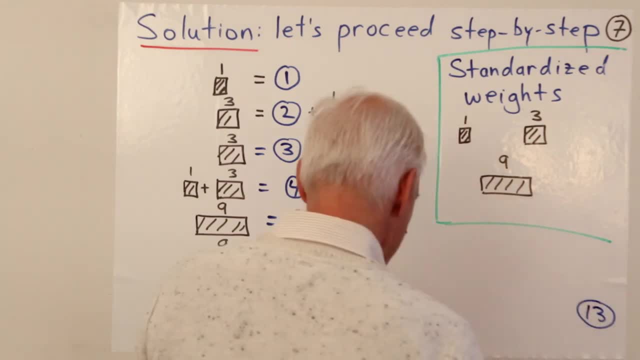 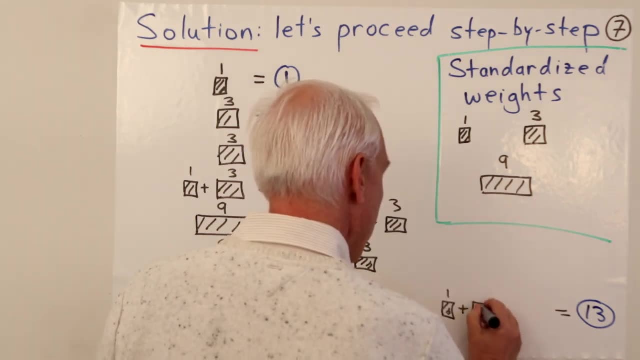 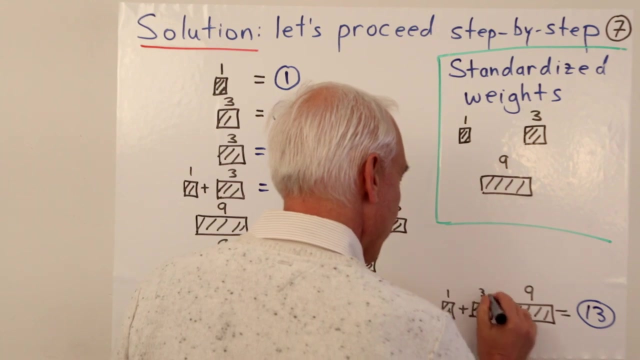 So I'll put the thirteen over here, And that's equal to a one and a three, and our nine. One plus three plus nine is thirteen. And of course there are the intermediate ones which I'm leaving to you. So that's part of the story. You have to write them down. 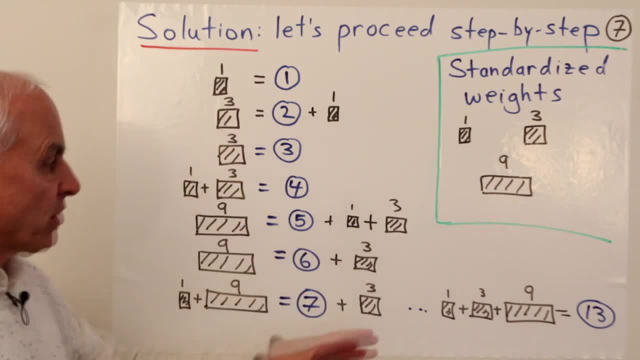 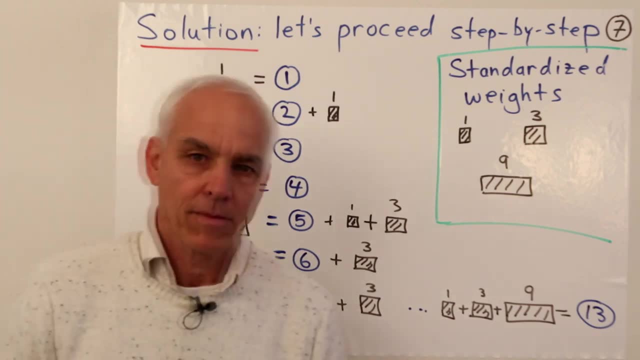 But I'm going to leave you to do that, And so that's as far as we can go with these three standardized weights. So this is more efficient than with the one, two and four. With the one, two and four weights we can only go up to seven. 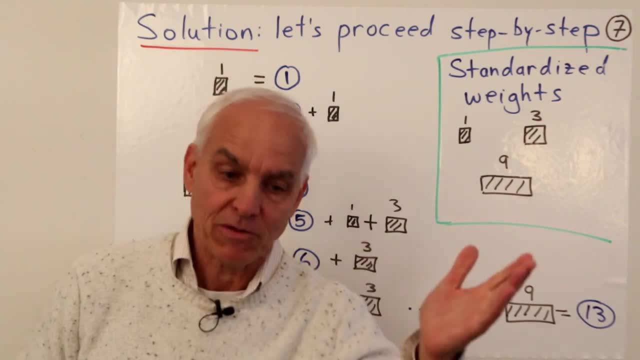 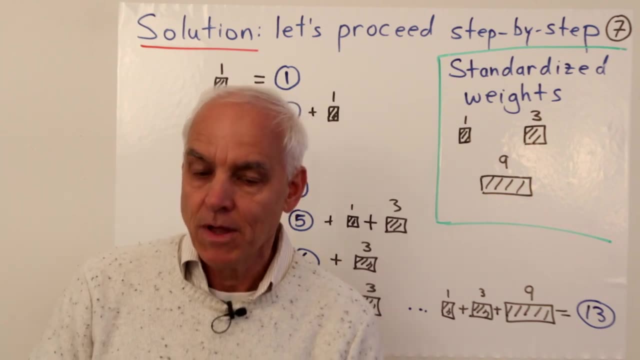 Now we're going up to thirteen because we're more flexible about using the pan balance. We're using the pan balance sort of in a more sensible way really. So this is great because, first of all, it's a little bit clever. 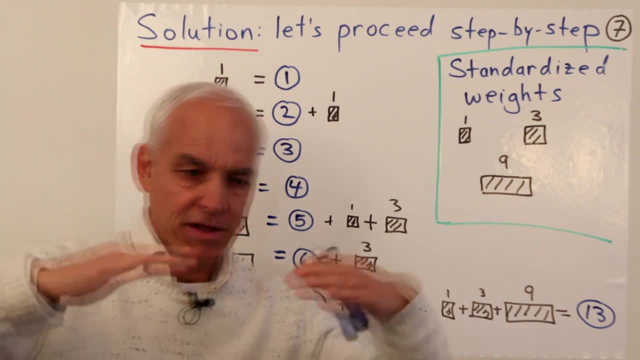 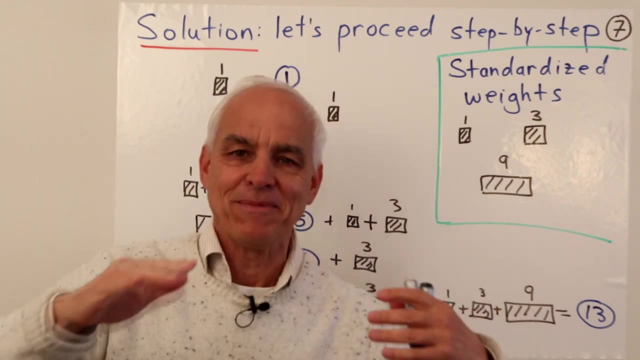 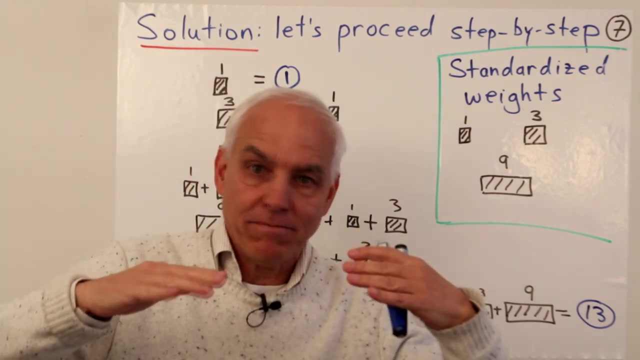 We're getting the students to think about the importance of balancing, that we can put stuff on either side of the balance. That's so important when it comes to doing arithmetic and algebra later on, because an equation is very much like a balancing situation. 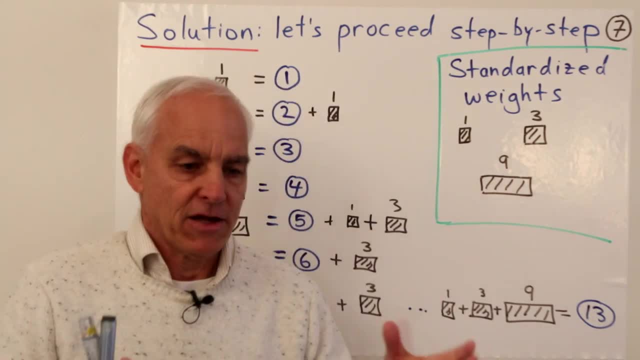 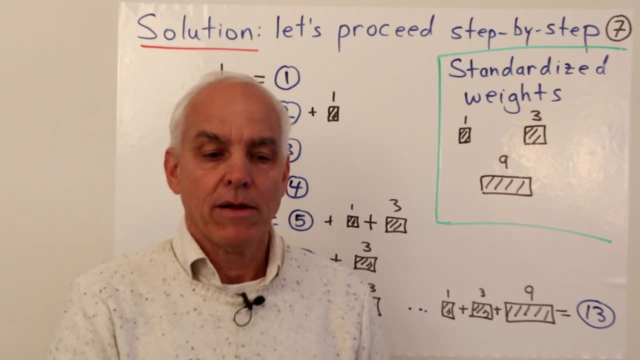 Very much like that. So this idea of moving one from this side to another side, how does that affect the rest? That's really good practice for later on, learning to be confident about manipulating equations, And also it's intrinsically interesting. 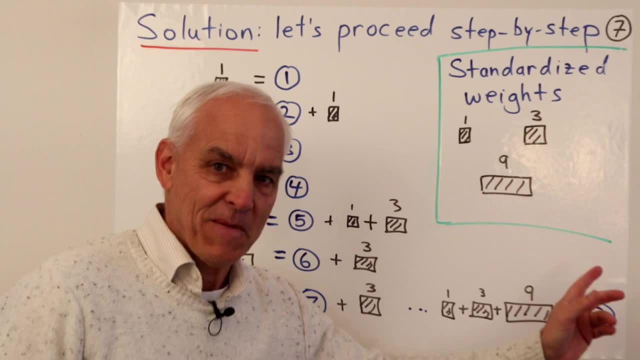 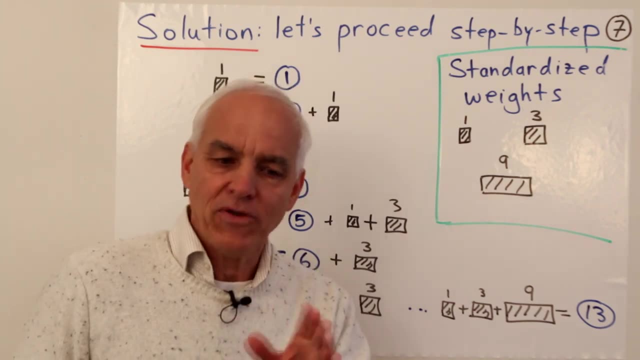 and naturally suggests what should be the next weight that we should introduce if we want to go further, And hopefully you'll be able to figure that out- Even a good primary school student will be able, after some thinking, to make a good guess as to what that next standardized weight. 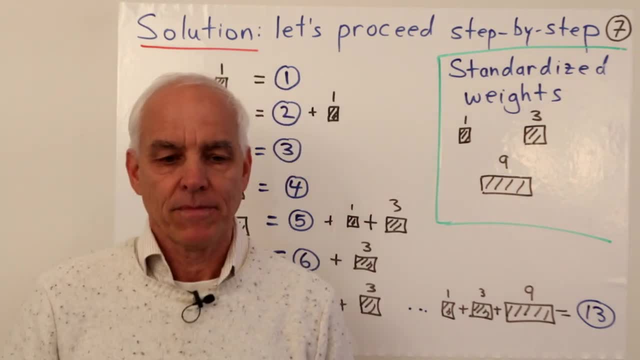 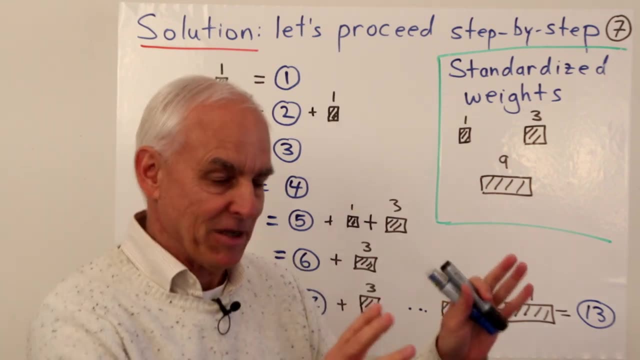 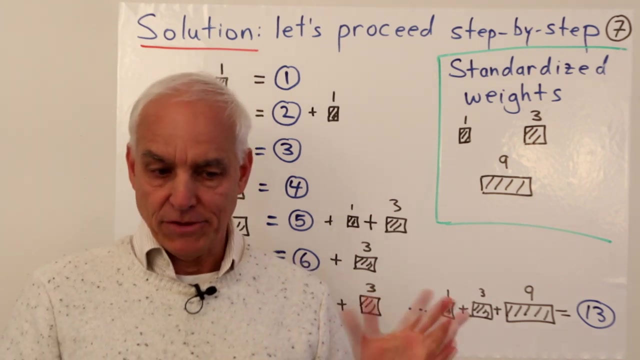 in this sequence ought to be So. we see here that there's an interesting alternative to the important binary system involving powers of two That's such a big part of our world. Here in the standardized weight story there's also- well, there's also- powers of something else floating around here.